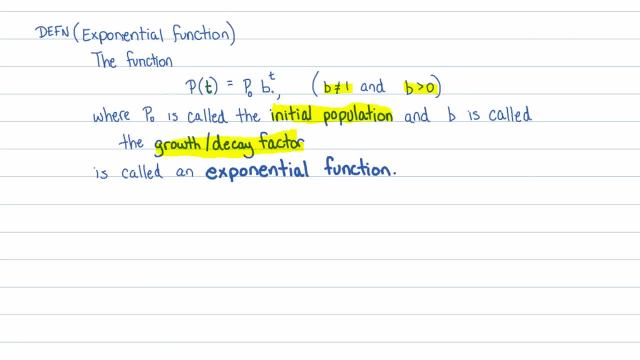 P of t is equal to P0, b to the t Again, where the base here cannot be 1 and it must be positive, and the base is also called the growth or decay factor. P0 is called the initial population. Now, when you're graphing, generally we just want generic axes when we're graphing, so often when we graph, you'll see that a lot of instructors or a lot of textbooks 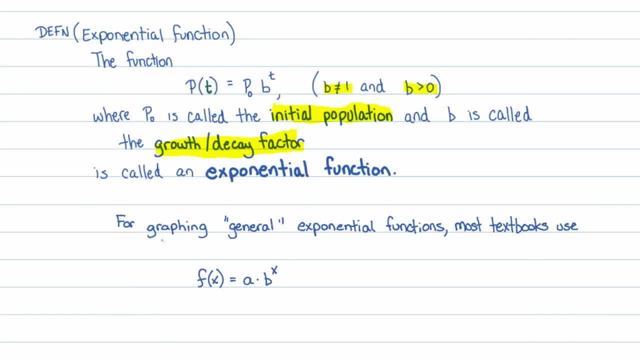 we'll use the following notation: F of x is equal to a times b to the x. Really, our unknown in this equation is still x, so our unknown is still in the exponent, which means it's still an exponential function. And instead of writing P0, we wrote a. 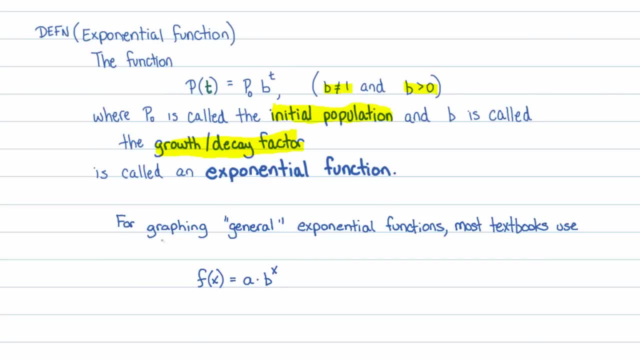 It really does. a is still the initial population. It's just that most authors use this Secondary notation for an exponential function, so you kind of have to get used to it. I don't like using two notations personally, but I'll just kind of introduce you to it here so that you're not confused when you see it in a textbook. 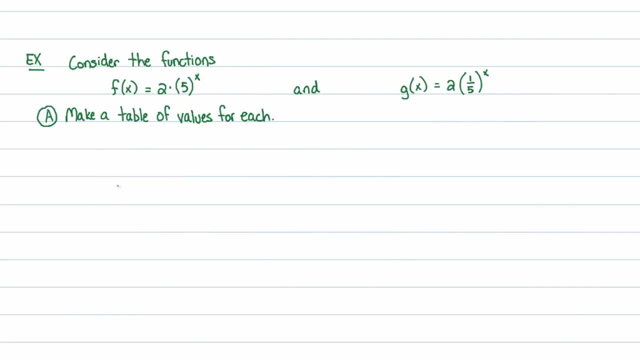 So let's consider the two following functions: F of x is equal to 2 times 5 to the x, and g of x is equal to 2 times 1, fifth, to the x. We're going to compare the graphs of these. 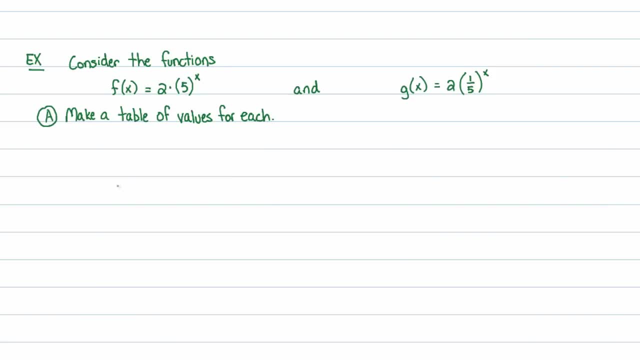 What we want to do is Make a table for each of them first, and then we'll plot points for those that exist on those tables and then compare their graphs. So for the first one, I'll go ahead and create a table. 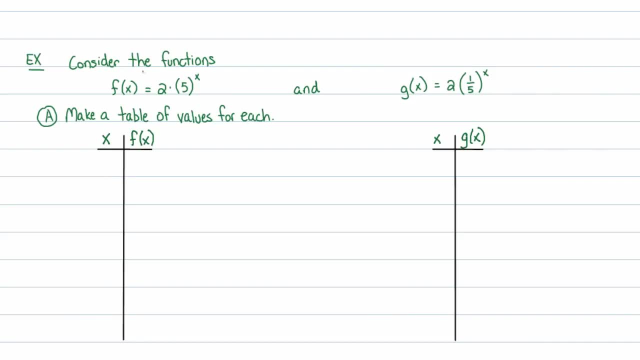 And when you're choosing values for your inputs, try to be intelligent with your values. You want to choose both negative and positive values, if you can. In this case, I'll choose negative 2, negative 1, 0, 1, 2.. 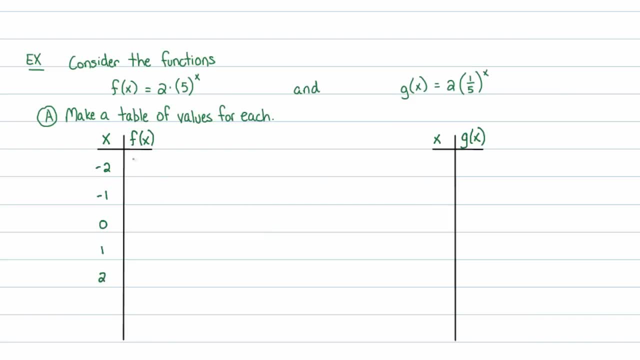 It's because exploring what the function values Are when you, when your inputs, are negative, it's kind of important. So let's see it's going to be 2 times 5 to the negative 2 power, Which is going to be 2 times 1 over 5 squared. 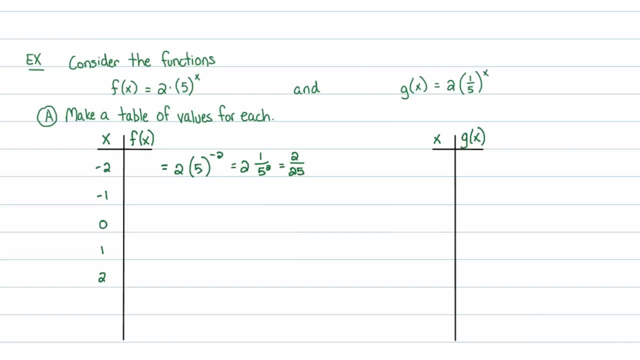 Which is going to be 2 over 25.. 2 25ths Now, if you recall from all my previous discussions about Exponential functions That I know if I'm going to increase the value of x by 1.. So I'm going from x equals negative 2 to x equals a negative 1.. 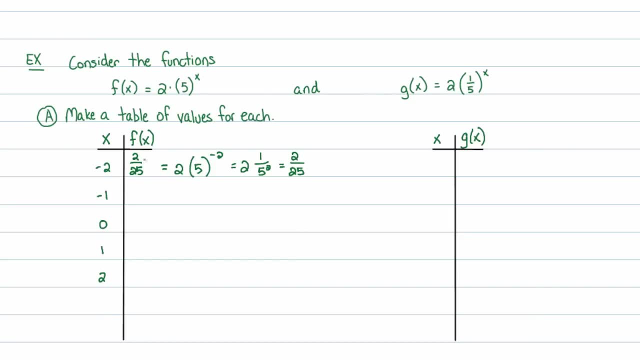 I'm going to multiply the output of 2 25ths by the base, And the base here is 5.. So I would expect this next value to be 2 over 5.. Because that's 2 25ths times 5.. 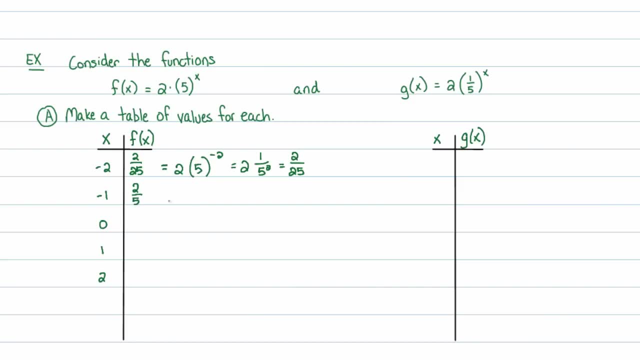 That's what I would expect it to be. Let's just see if that's true. So 2 times 5 to the negative first power, It's the same thing as 2 times 1 over 5. Or in other words, 2 5ths. 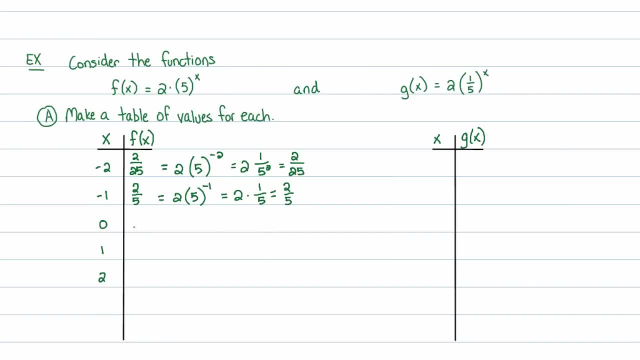 Which is exactly what I thought it would be. And again, using the fact that this is an exponential function, Take another step. a single step in the x direction Means I'm going to multiply the output by 5. again, It'll get me a 2.. 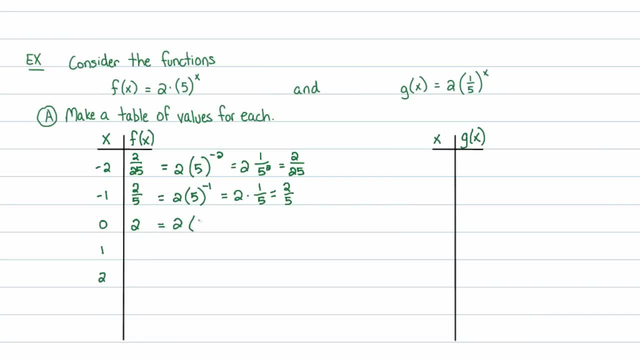 And you can double check that again 2 times: 5 to the 0th power. Well, 5 to the 0th power is just 1.. So that's 2.. And now multiply this by 5. I'll get 10.. 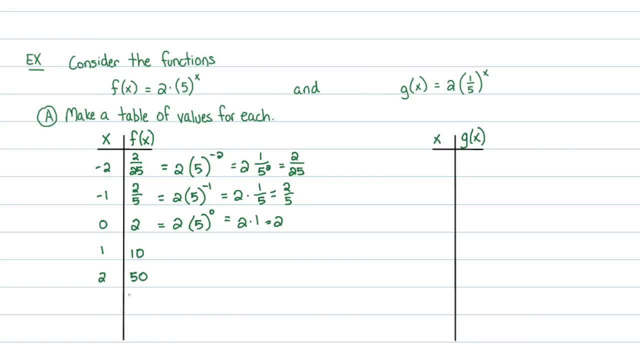 Multiply that by 5.. I get 50.. You see how easy it is once you realize you're just multiplying by 5s. So that's not so bad. So there's our table for f of x. Let's look at a table for g of x here. 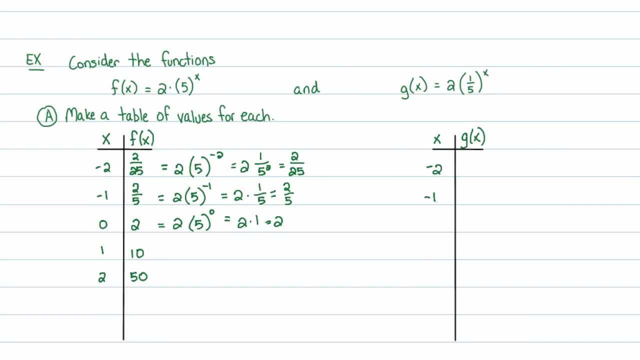 Again, I'm going to do negative 2,, negative 1,, 0,, 1, and 2.. In this first case, when I plug in a negative 2, I'll get 2 times 1, 5th to the negative 2 power. 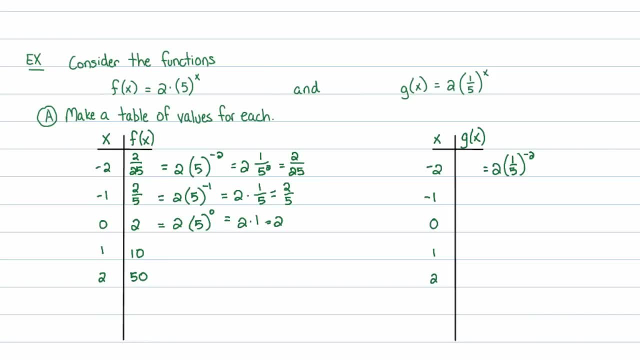 And remember that negative. I can rip off the negative off the exponent. It'll give me the reciprocal of what's on the inside. So that's 5 over 1, all being raised to the 2nd power. Well, that's 5 to the 2nd power. 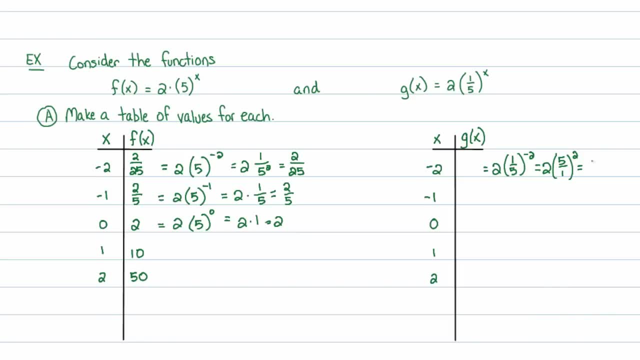 Or in other words, 25 times 2 will be 50. So this is 50. Now again, the base of this one is 1: 5th. So I know that every single step that I go in the x direction, 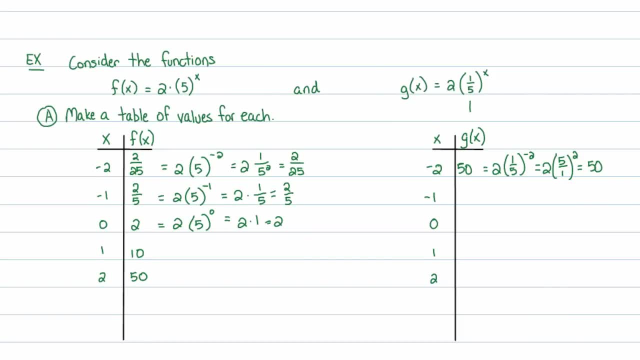 the output will be multiplied by 1- 5th. So I should ask myself: what's 1 5th of 50?? Well, I know that's going to be 10.. But let's just double check that 2 times 1, 5th to the negative 1.. 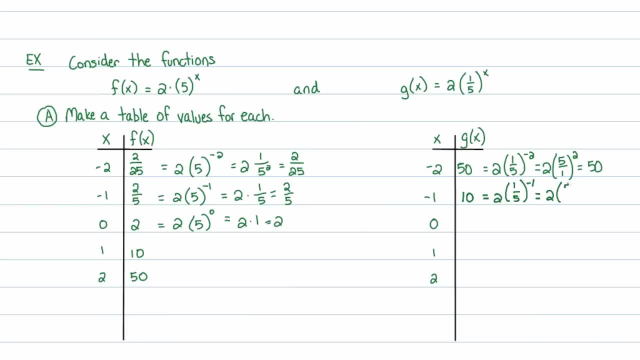 1, 5th to the negative. 1 is the same thing as 5 over 1 to the 1st, And that's just 5.. 5 times 2 is 10.. So that does work out. And take another step. 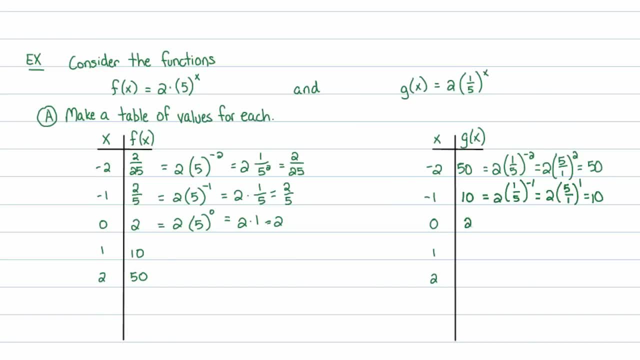 And we'll be multiplying 10 by 1: 5th, which will give me 2.. You can double check, if you want. 2 times 1, 5th to the 0th, power is just going to be 2 times 1.. 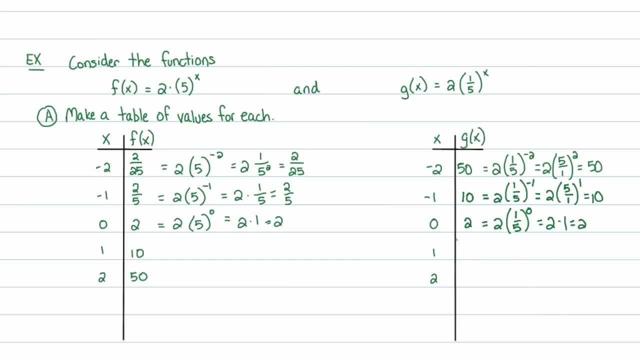 Which is 2.. And then again, take 1 5th of 2.. That's going to be 2 5ths. Take 1 5th of 2 5ths. That's going to be 2, 25ths. 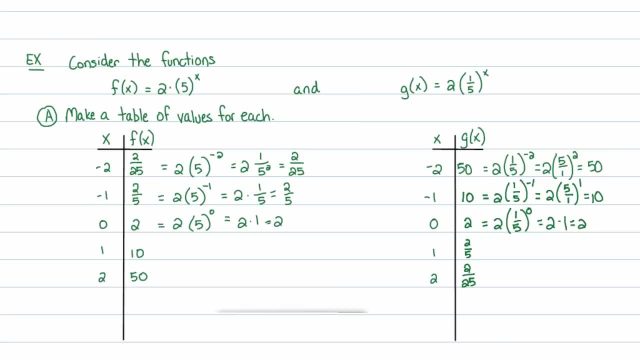 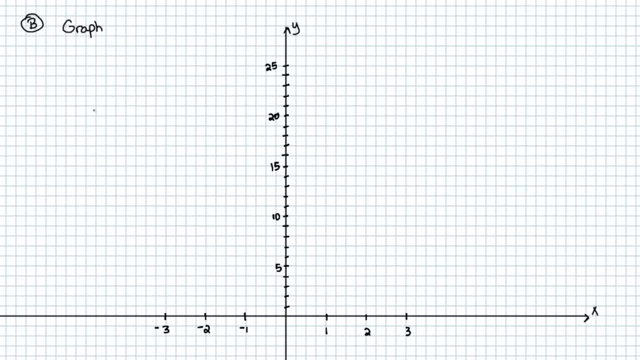 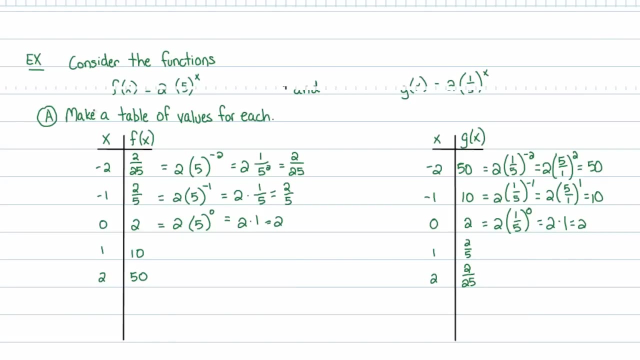 There we have our table of values here. Now we'll go ahead and make some graphs. So I've set up some axes here And we're going to go ahead and plot these points Now. if you look at the previous tables here: 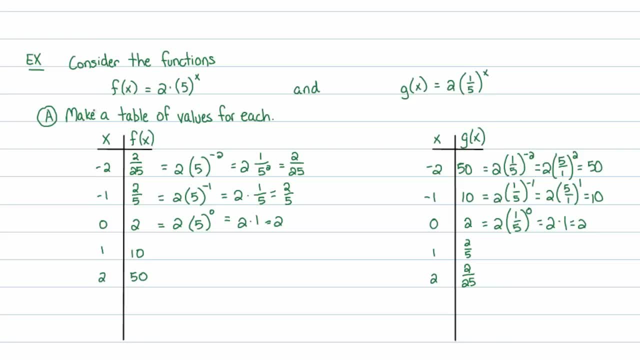 I'll go ahead and plot F first And if you want, you can pause the video and write those down. I'll just say that I know those numbers right now And I'll go ahead and plot them out. So I've plotted the points in here. 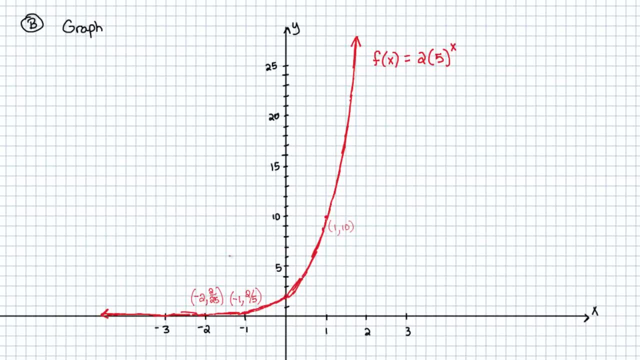 And I've connected them with a smooth curve. Now a couple things you should note here. One: the curve is increasing, So let's go ahead and note that It's increasing, And it's increasing because the fact is that our growth factor is 5.. 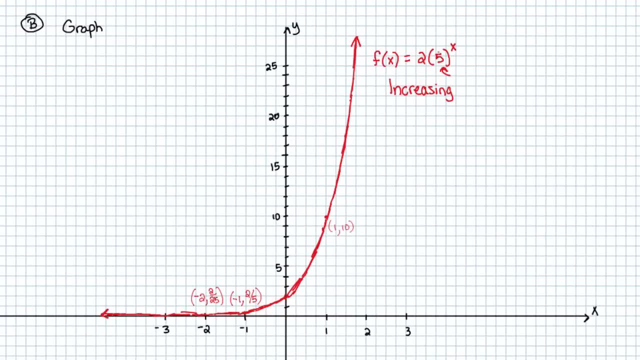 In other words, each step we're multiplying by 5.. So obviously, if you're talking money and every day you multiply the amount you have by 5, you are increasing the amount of money you have. So increasing and I'll say because the growth factor 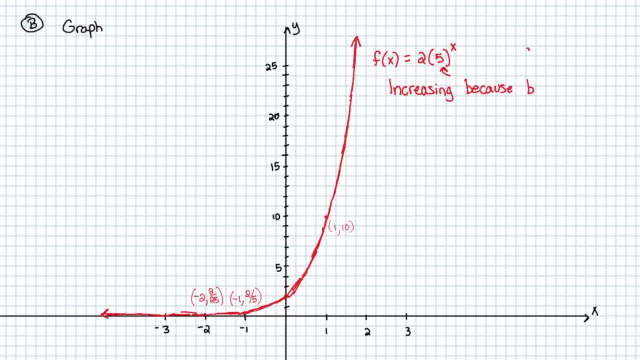 which is B for our A times, B to the X business. our growth factor is greater than 1.. If you keep multiplying the amount of money you have by a number that's greater than 1, you're going to get more and more money. 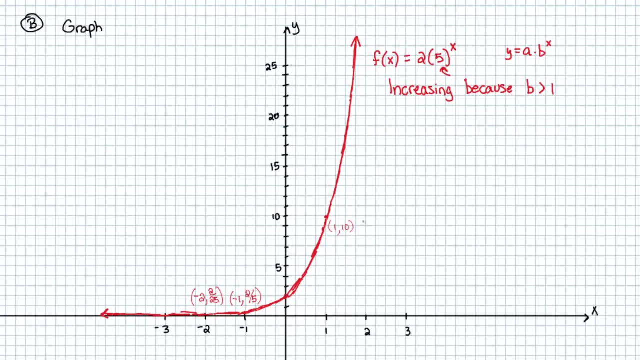 So that's increasing, All right. So that's one thing that's super important to note. Another thing you should probably note here is this point that I've kind of really highlighted right there. That point is at: X equals 0, Y equals 2.. 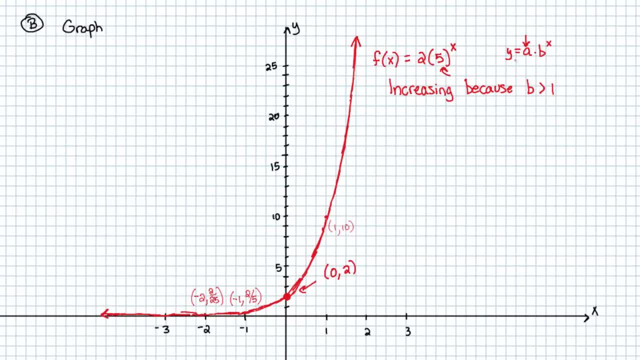 And remember what I said about that A value, or this 2 value, right here in the exponential function, We call it the initial value, And the reason why is because that's where the graph is initially, In other words, at X, equals 0.. 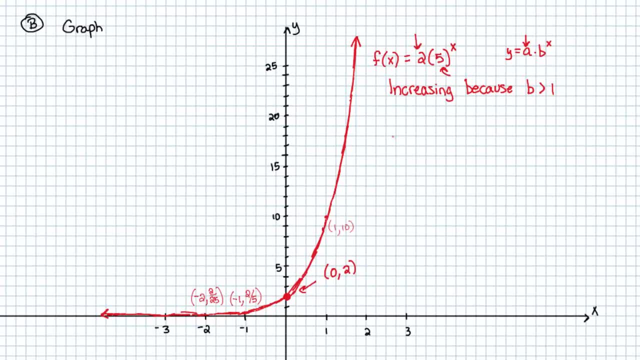 I always think of X equals 0 as the initial time, because the X axis is often in real life represented as a time axis. So you sometimes will say that's our T axis and at time equals 0, the output is 2.. 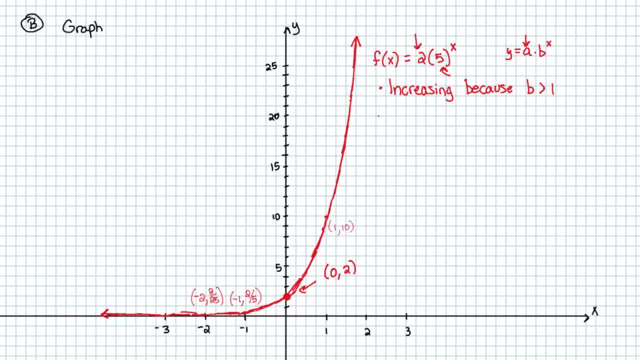 So please note as well that the Y intercept is 0, A. Okay, That's a very important point to make. It's at the initial value. So this is kind of continuing all this conversation we had previously about exponential functions and that coefficient. 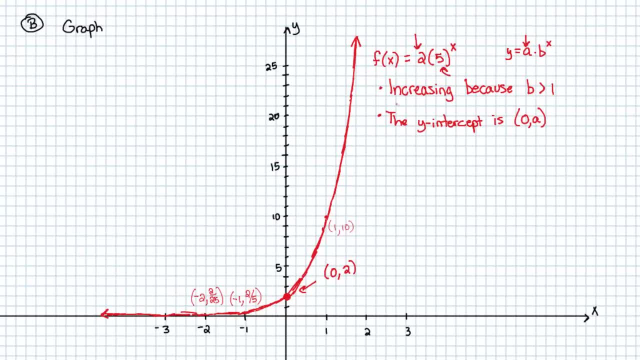 that number in front of the base there is always called the initial value, And that when you have a large base, you have an increasing function. Another thing you'll need to note about this function is that it's not only is it- always increasing. 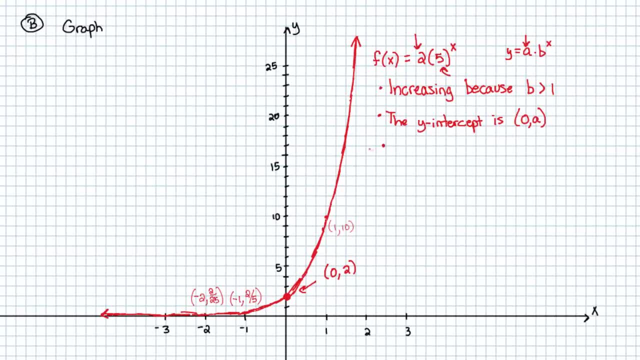 but It also never goes negative. If you look at this function, see how this curve kind of approaches the X axis. It doesn't actually go below the X axis. 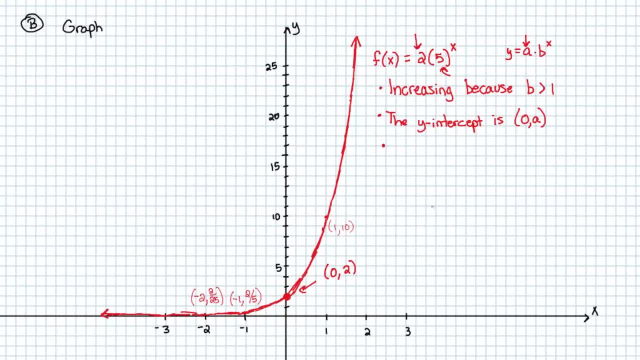 It doesn't go into quadrants 3 or 4.. So that means that the range of the function, the set of Y values the function can take on, starts at 0,, a height of 0,, a Y value of 0, and climbs all the way up, continues all the way up until. 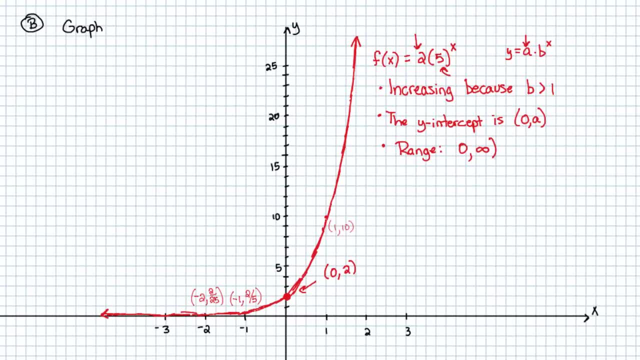 And in this case it will never actually touch 0.. 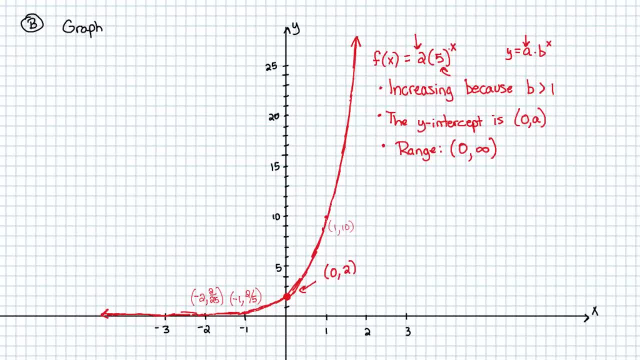 You can easily see why. plug in: let X equal. because some people will say: well, wait, if X is negative 3, it looks like it's touching the X axis, It looks like it's at a height of 0. But if you plug in, X equals a negative 3.. 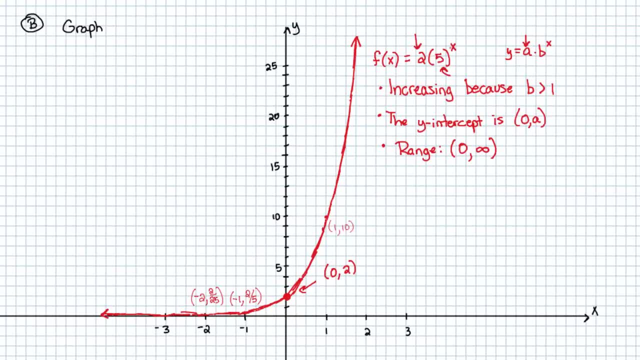 you get two times five to the negative third power five to the negative third is one hundred one over one twenty five, so that's going to be two over one twenty five. that's not zero, and in fact plug in the negative billion for x. in other words, let x be super, super far. 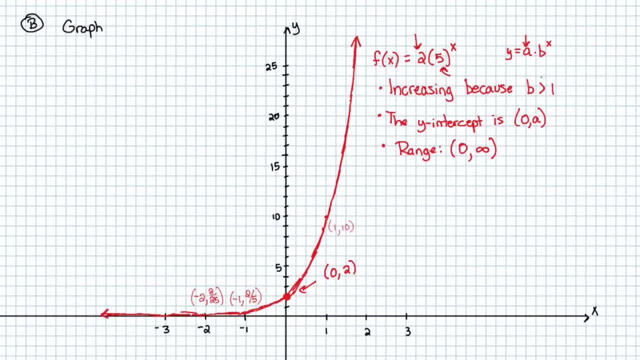 to the left on this graph and you'll find out that- and I'll erase this in a moment, just so I don't confuse anybody- but if you evaluate this at like a negative huge number, like a negative ten to the ninth power or something like that, this would be two over a huge number. 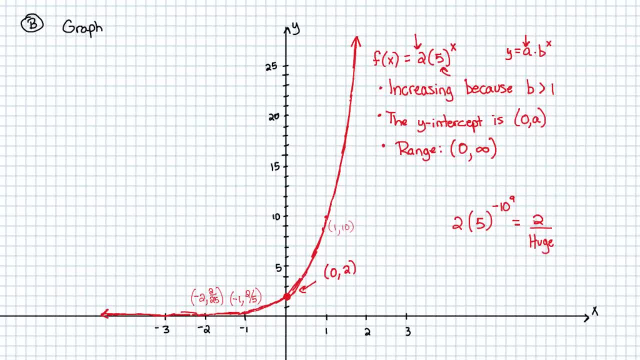 very huge number, but it's still not zero. it's, it's close to zero, trust me. it's extremely close to zero, but it's not zero. so the fact is, your set of outputs will never actually reach zero. now I actually talked about the harder part of domain and range. first, because the domain is a lot easier, remember? 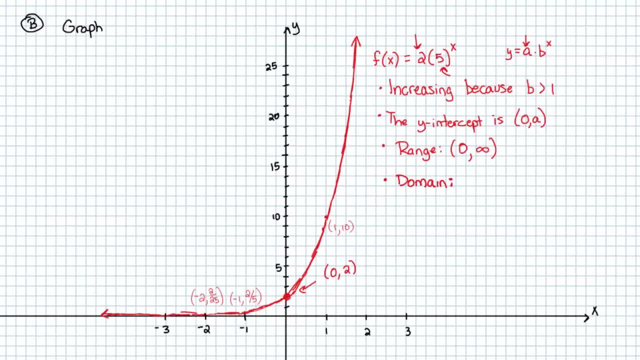 domain is a set of all possible values that the x can be and if you look at this graph, I could see that in the negative direction, x could be anything I want. it could be negative, three negative three point two, five negative thousand, whatever I want, and same thing in. 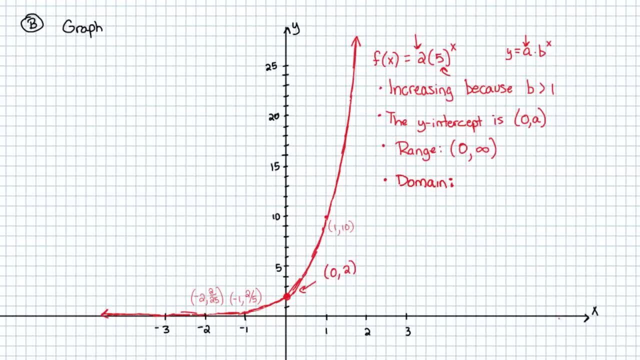 the positive x direction it. I could let x be a trillion if I wanted to. it's just that the graph would be super far up in the sky, but it's still. I can plug in those values for x. so I could plug in anything I want negative infinity. 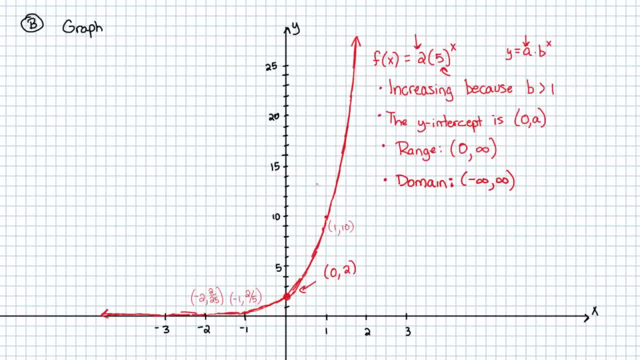 to positive infinity. now, finally, I just want to mention one last feature of this graph is that we have a horizontal asymptote, and if you recall what a horizontal asymptote is, it's just basically what your function approaches as time goes on. so maybe I should write that down as x approaches negative infinity, as it gets really, really negative. 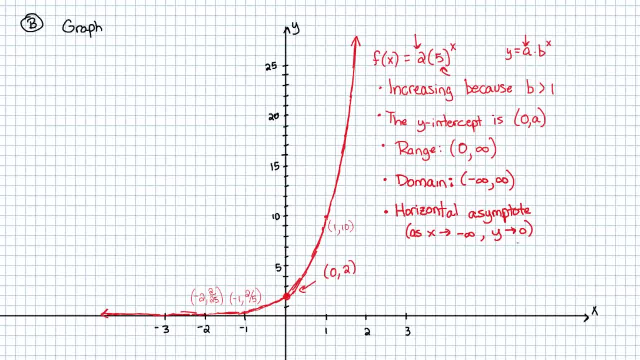 the y values approach zero, and that's what a horizontal asymptote is just saying. if you let x get very positive or very negative, do the y values approach a solid number? well, as x goes to positive infinity, the y values also blow up. so in that direction, 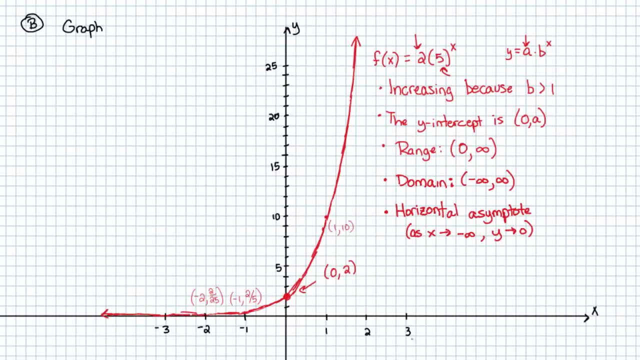 and three. there technically is not a horizontal asymptote, but in the negative direction. we see, as x gets really, really negative, this curve gets really close to y equals zero. It doesn't actually become y equals zero, but it gets really close to it. All right, so that was for f of x equals two times. 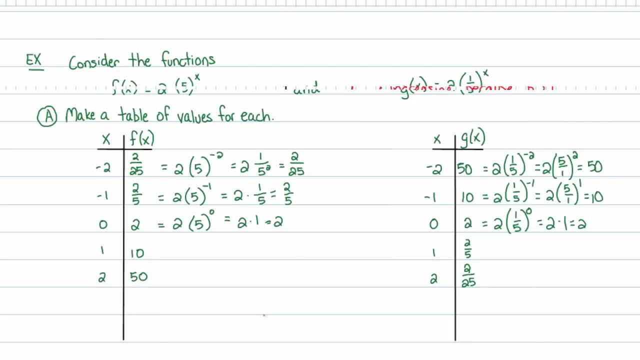 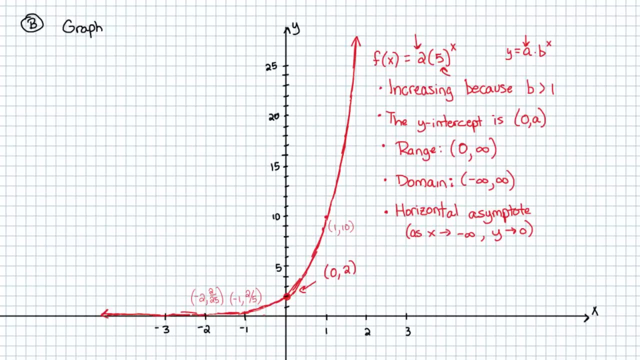 five raised to the x power. What about g of x, which is two times one fifth to the x power? How does that differ? Well, I went ahead and graphed this out and if you look the blue curve by the 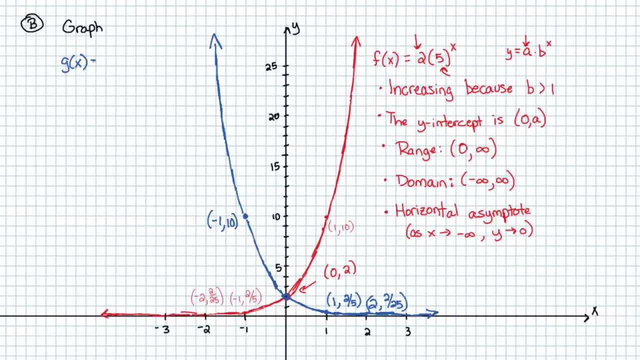 way is: g of x is equal to two times one fifth to the x power. I just plotted the points that we had on this page back here, so negative two comma fifty. I couldn't- I don't have fifty as an output on this table, so I just didn't have that on there. but 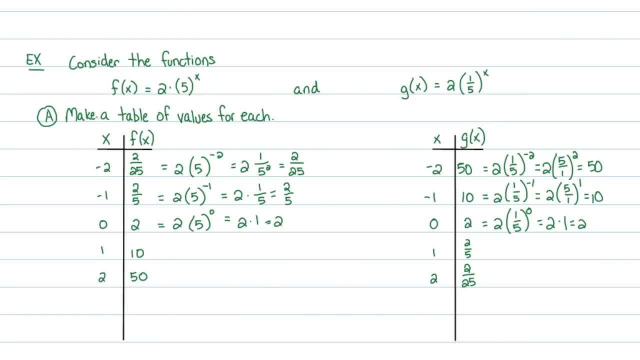 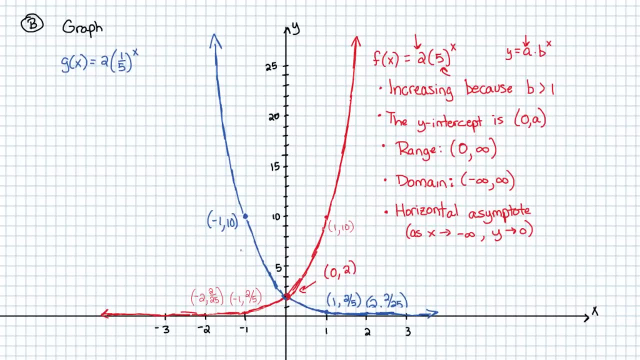 um, I did plot negative one comma ten and zero comma two and one comma two fifths and two comma two twenty-fifths. You can see it all right there. So the question is, can we make the same descriptions or similar descriptions as we did for the? for the f of x equals two times five to the x. Well, 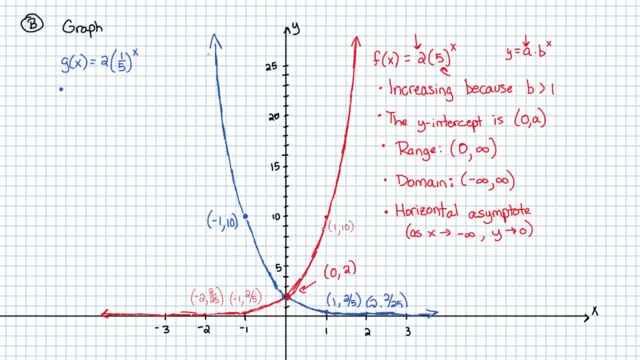 let's see: Is this increasing or decreasing? Well, when reading from left to right, this function is dropping down. so it is a decreasing function. and it's decreasing because every single step you take, you're multiplying by the base, and the base here is one-fifth. So think of it this way. 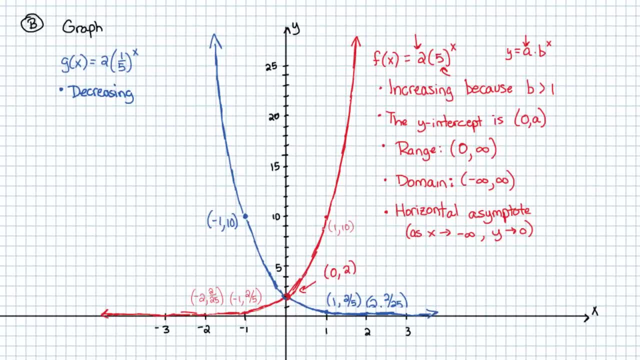 You have a thousand dollars Every day that passes. you multiply that by one-fifth. That's what you keep. You keep one-fifth of that money. So you start with a thousand dollars and the next day you have two hundred. So obviously you're losing money, right? So that's a decreasing pattern. 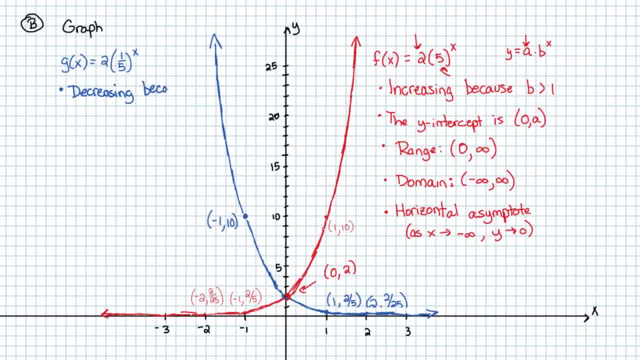 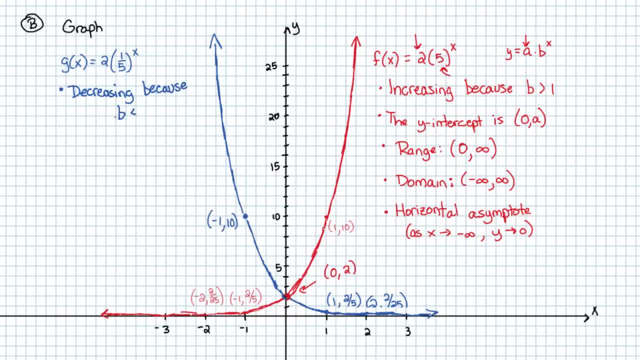 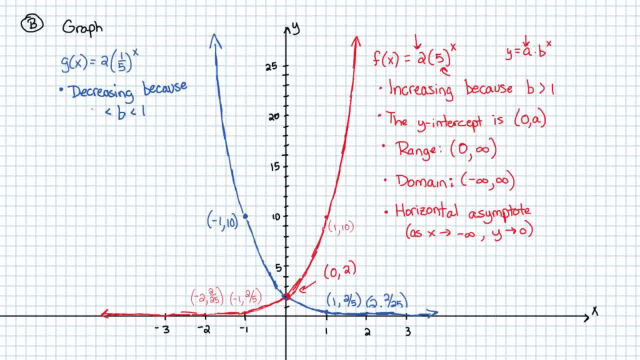 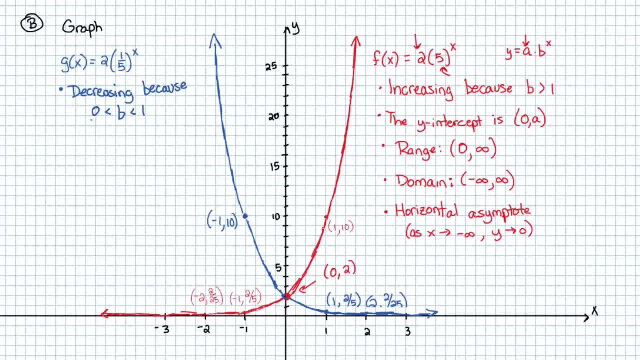 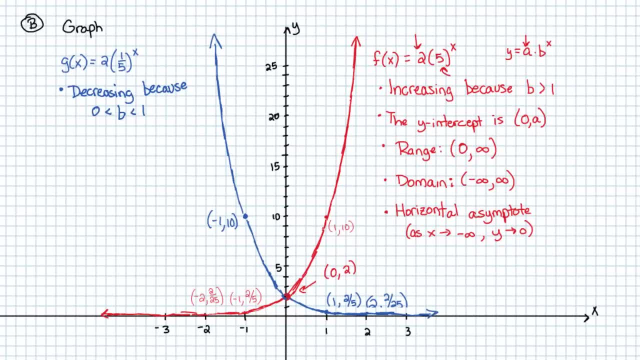 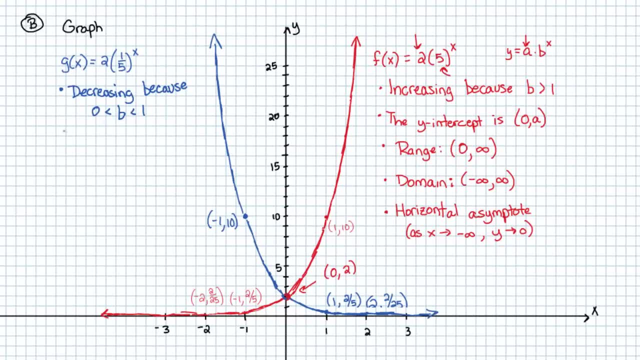 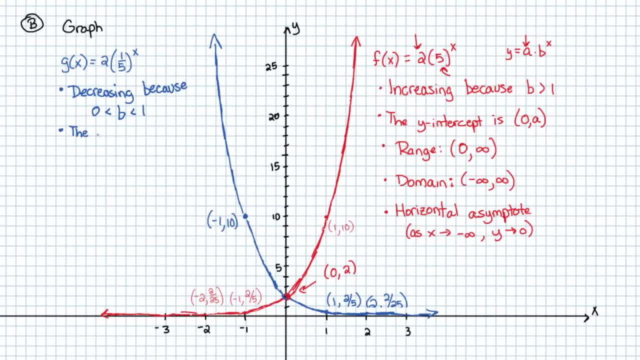 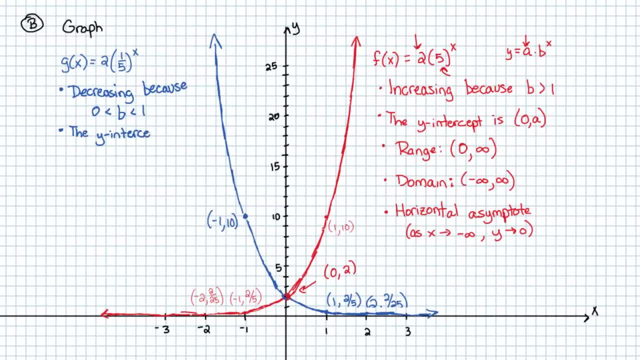 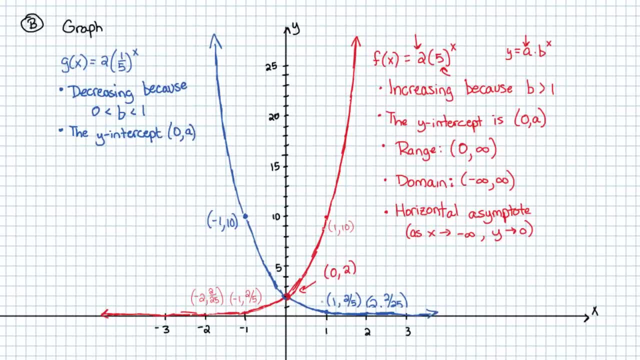 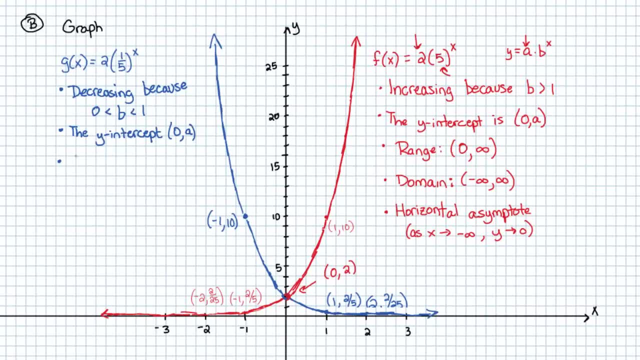 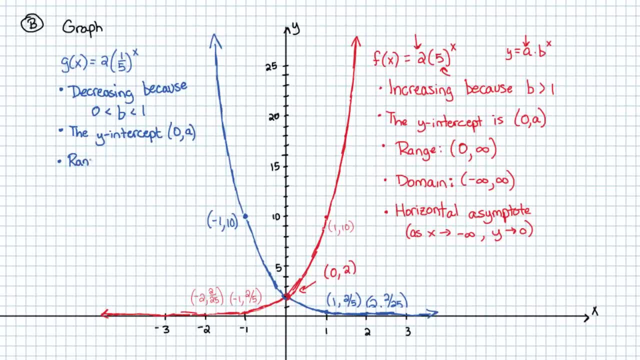 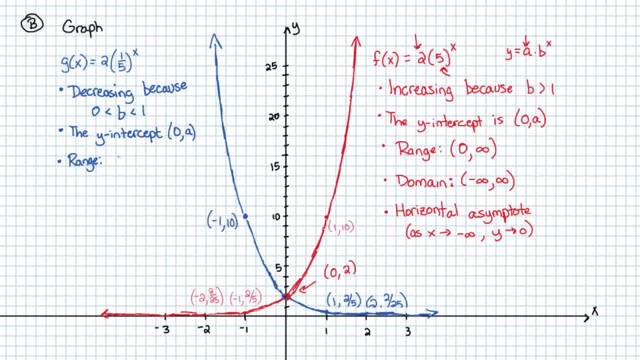 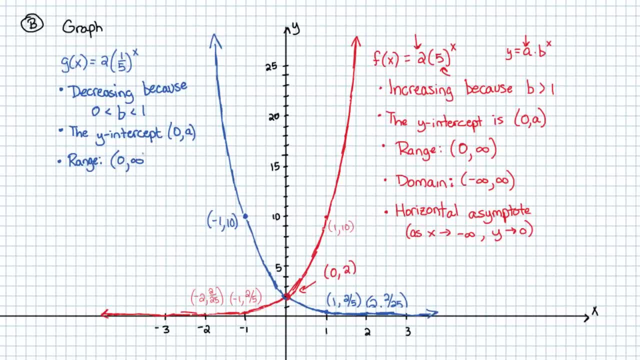 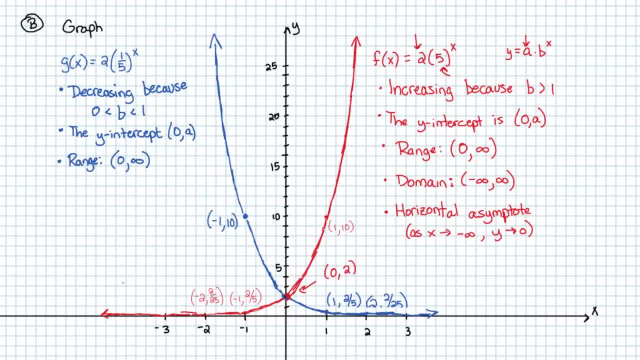 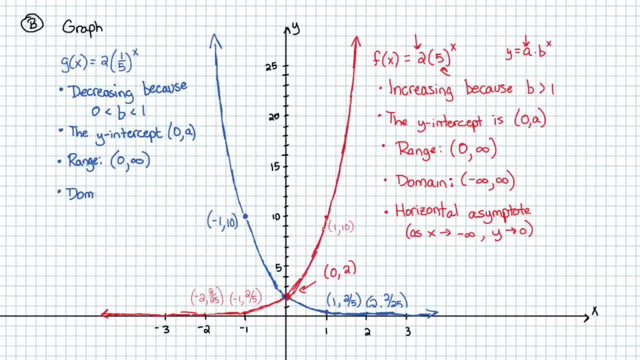 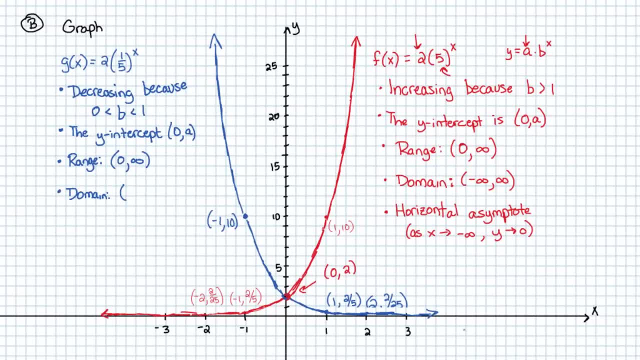 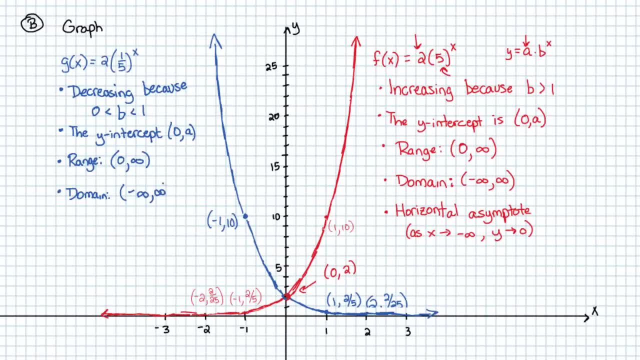 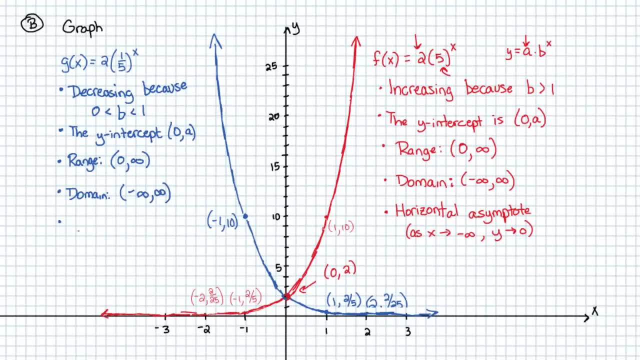 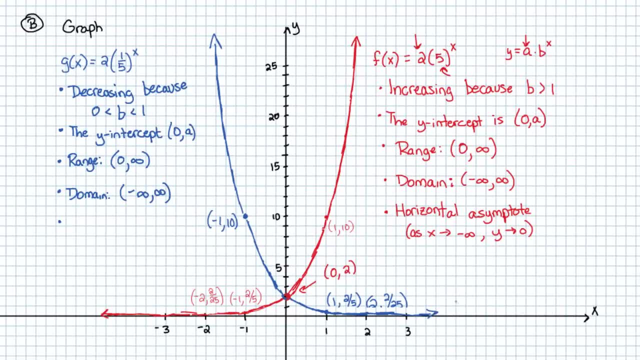 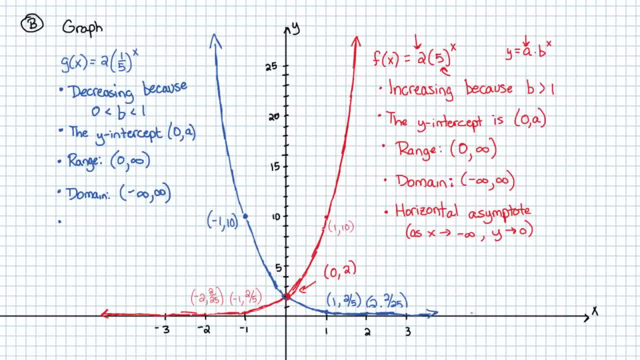 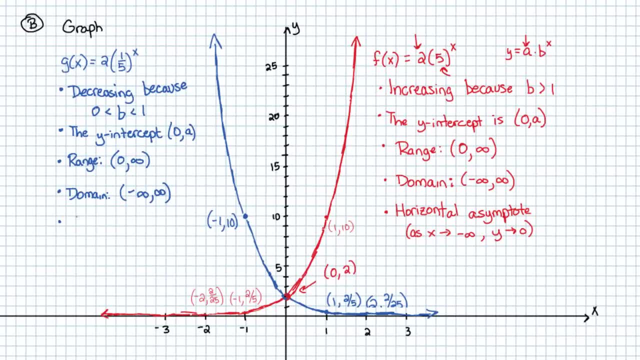 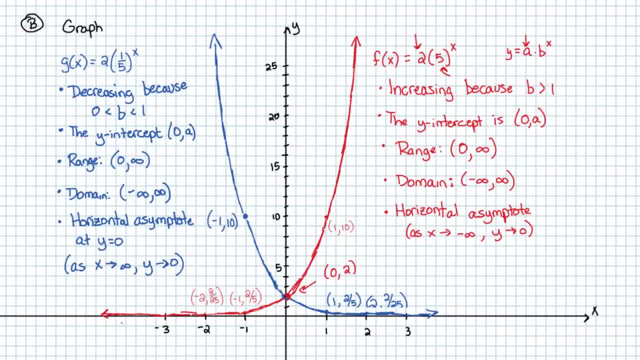 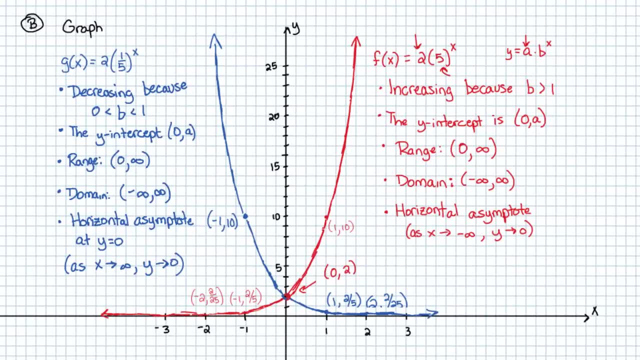 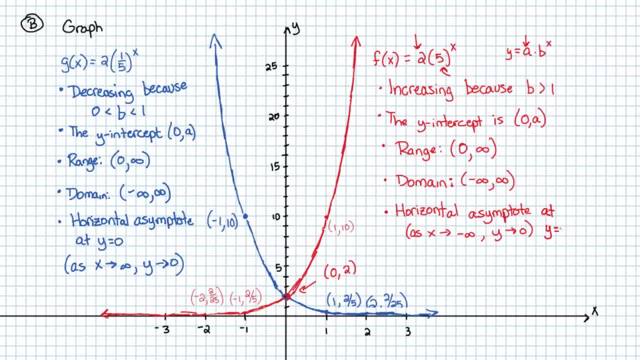 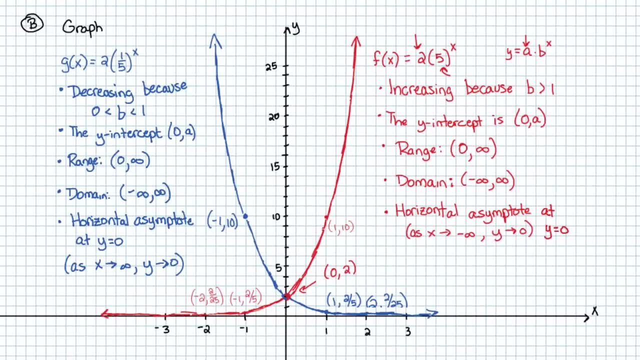 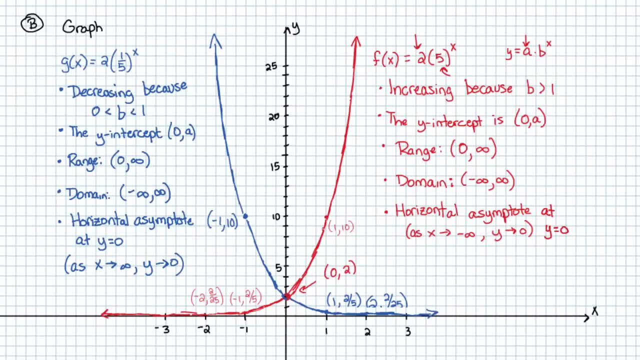 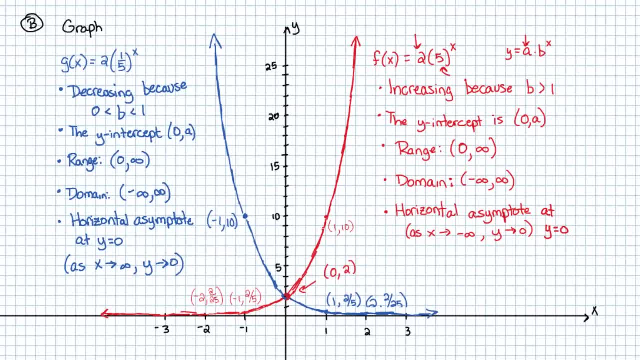 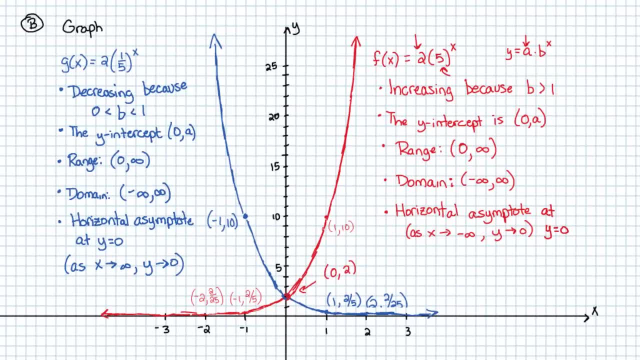 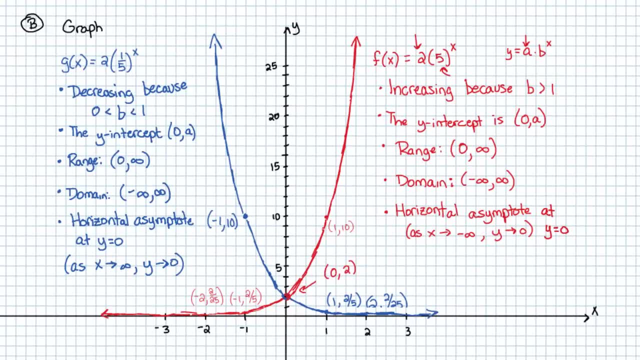 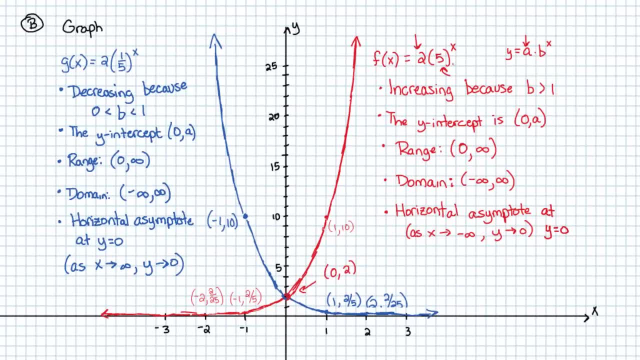 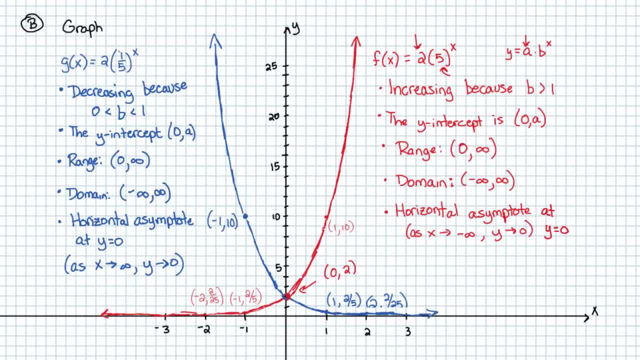 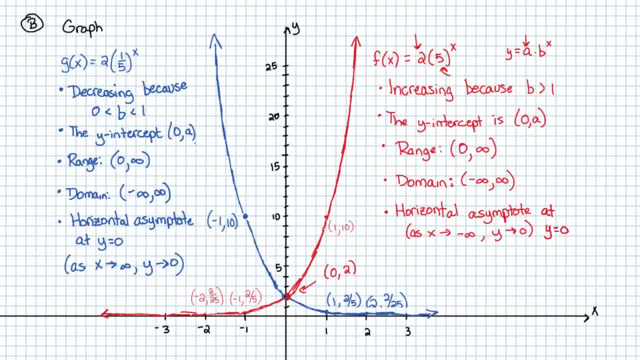 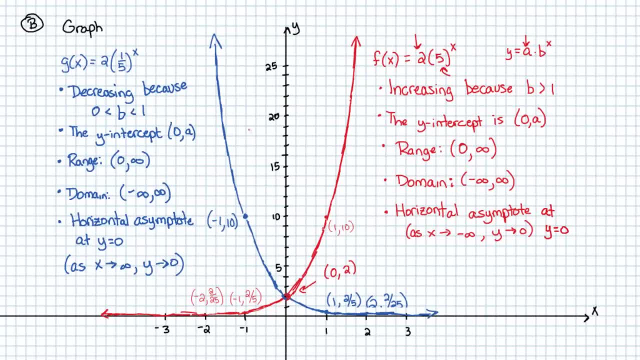 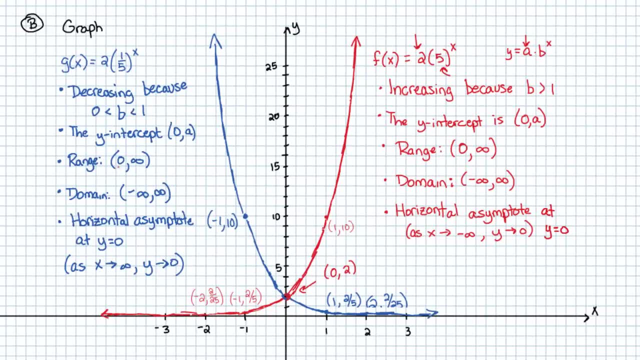 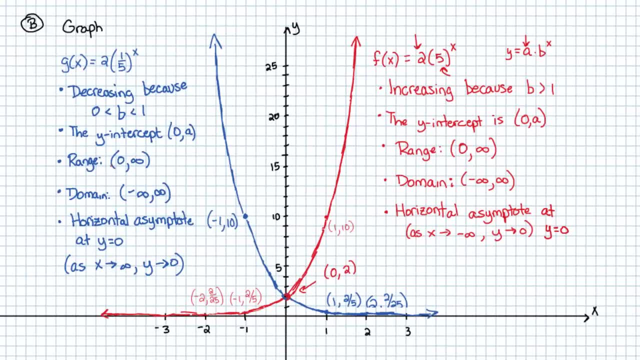 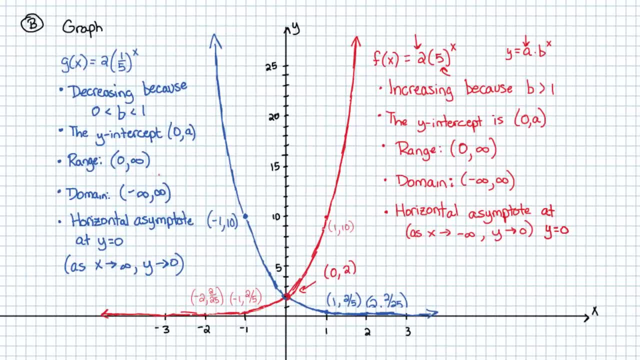 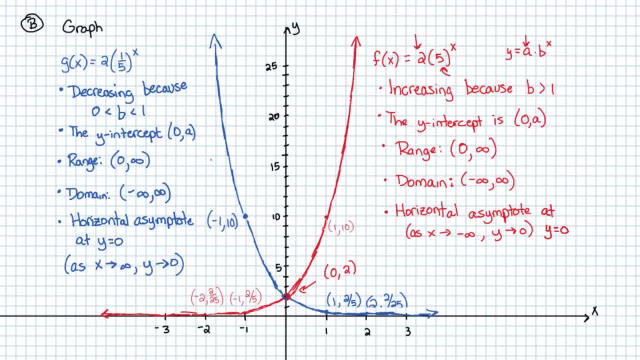 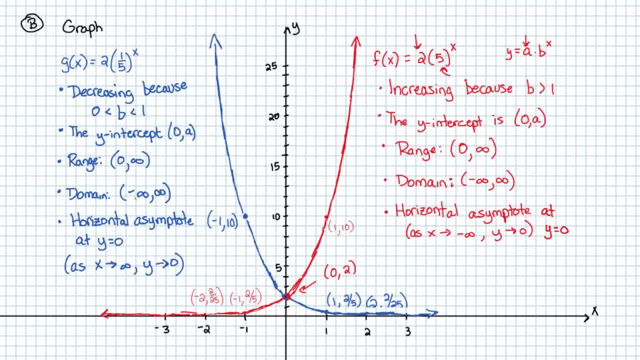 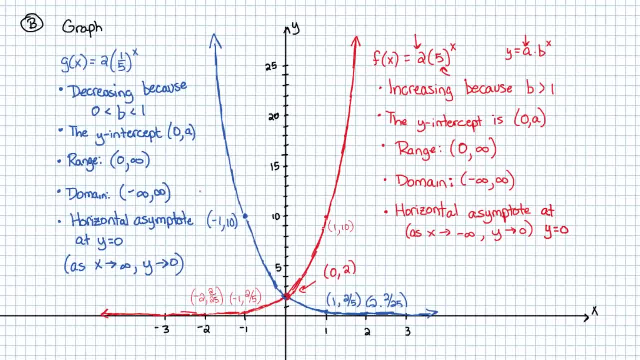 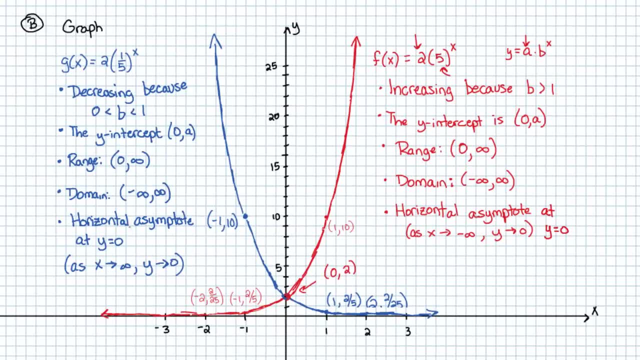 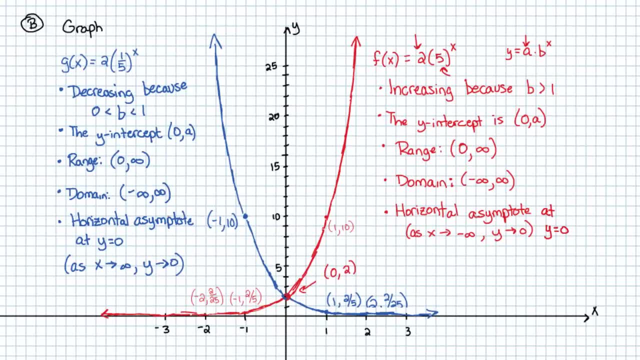 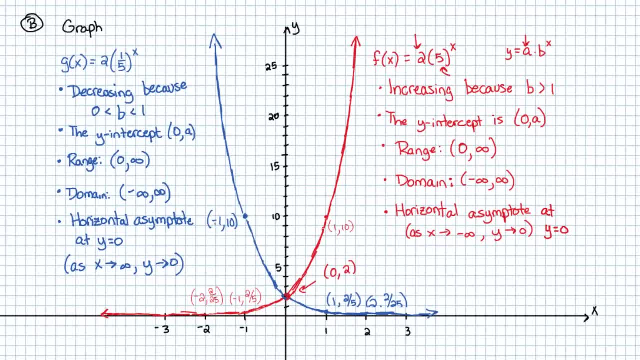 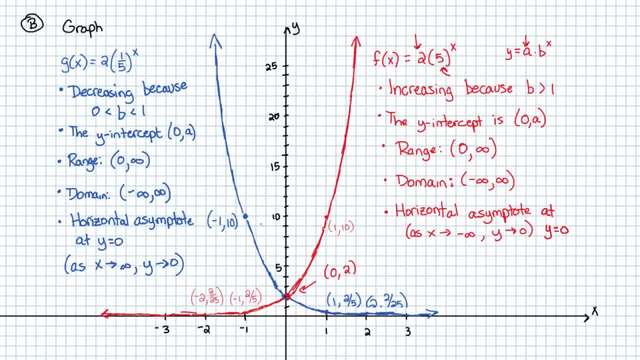 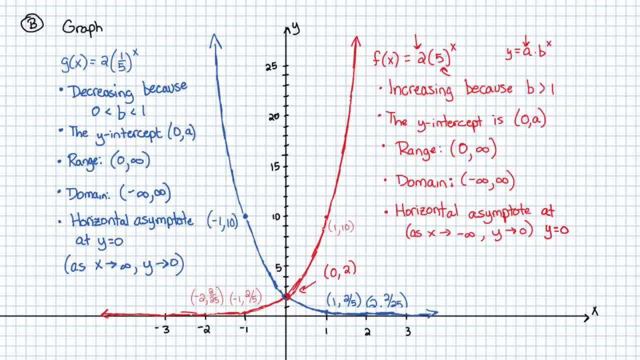 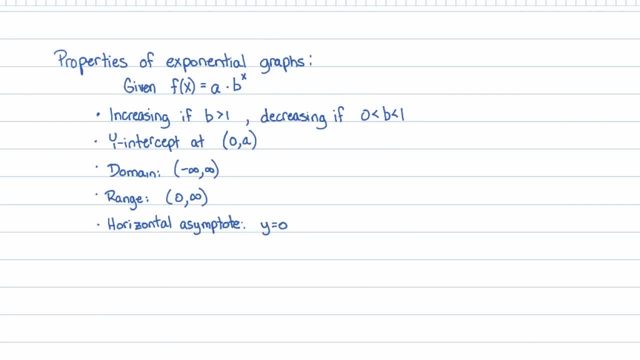 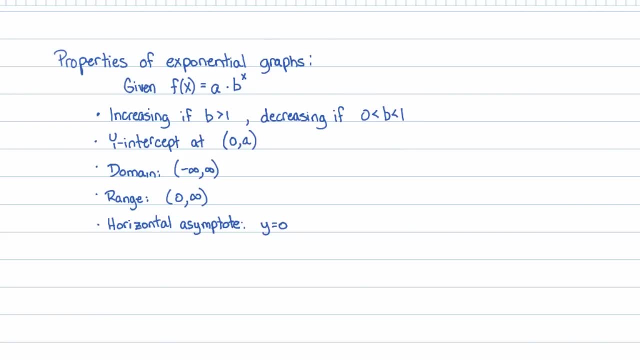 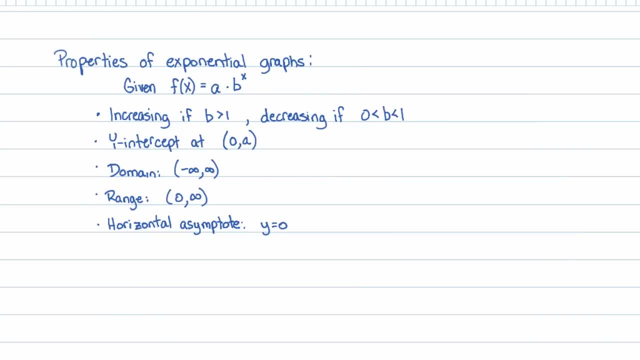 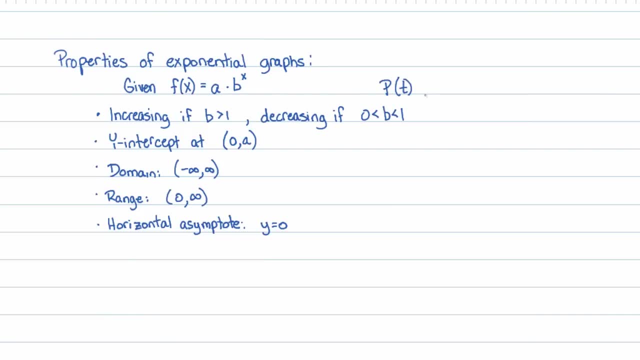 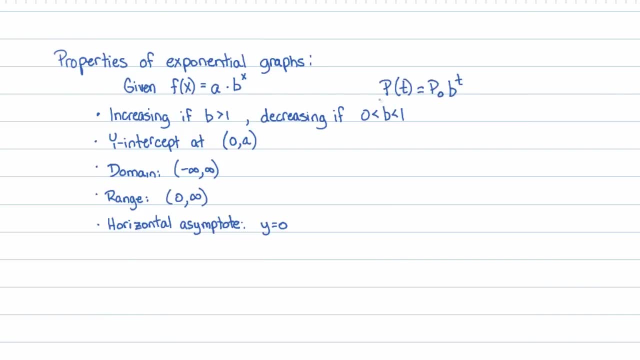 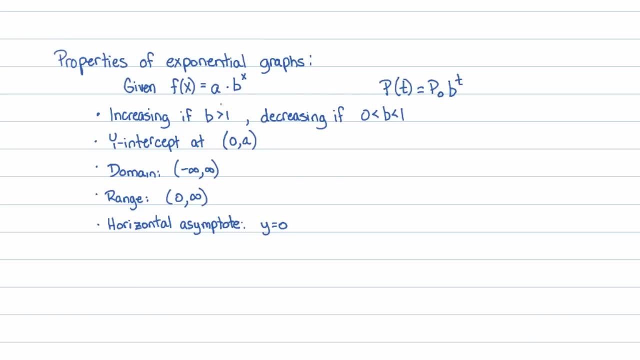 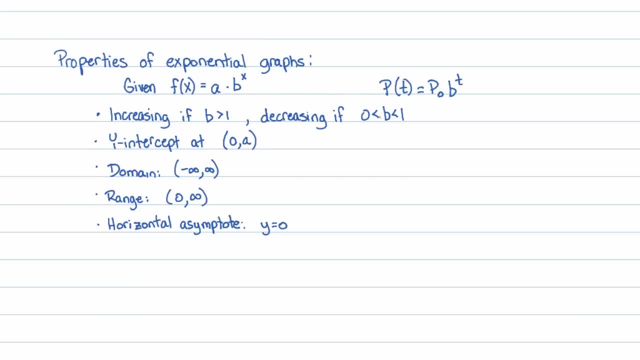 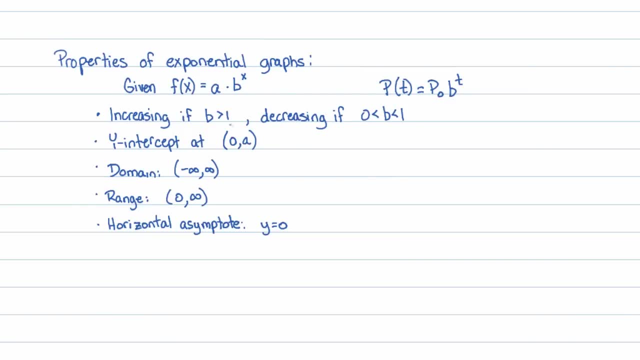 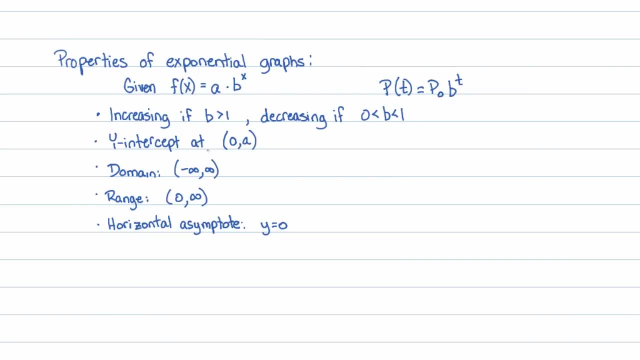 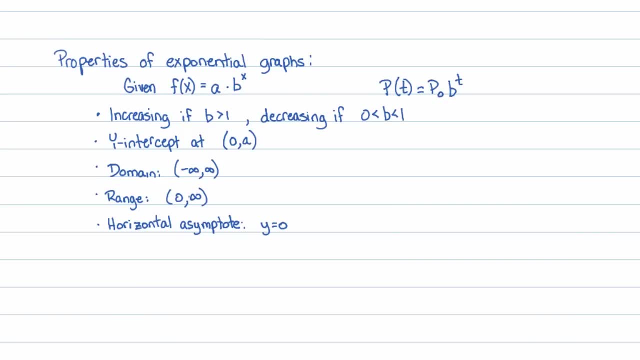 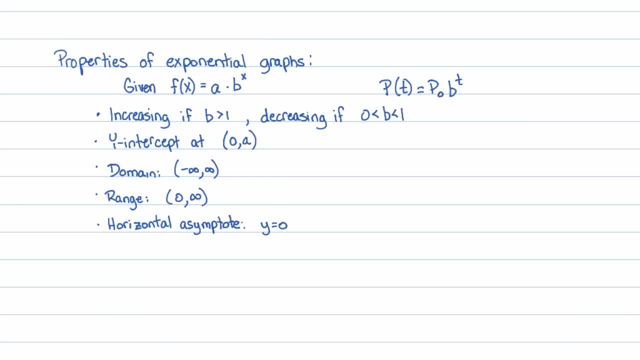 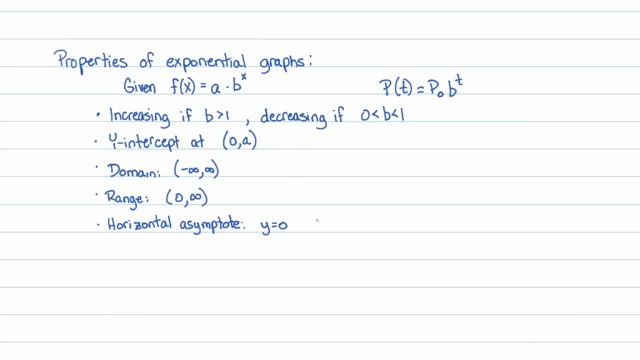 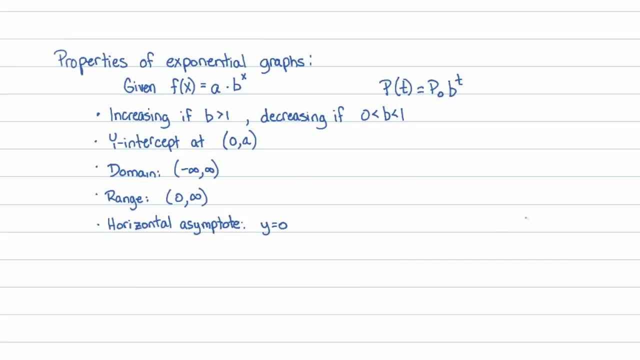 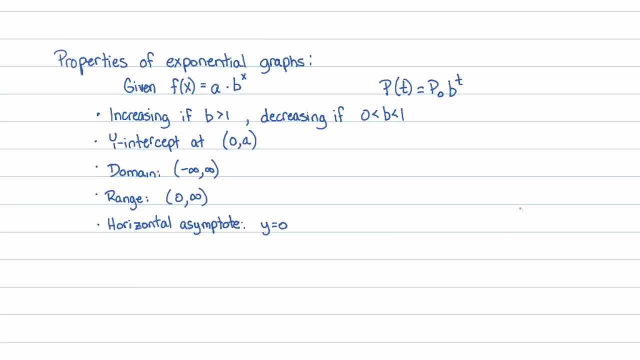 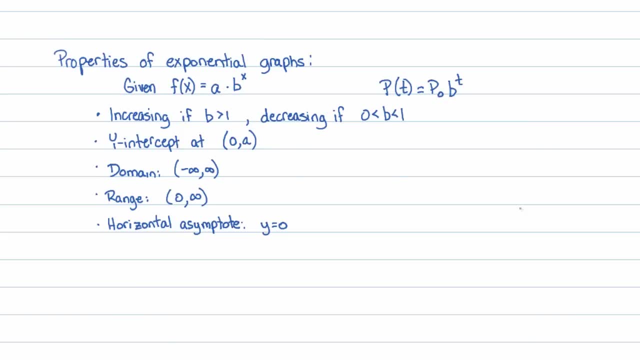 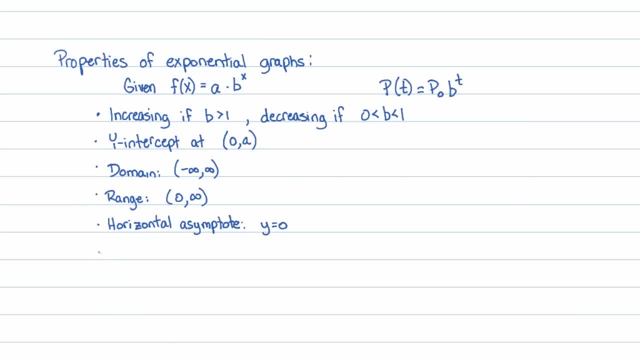 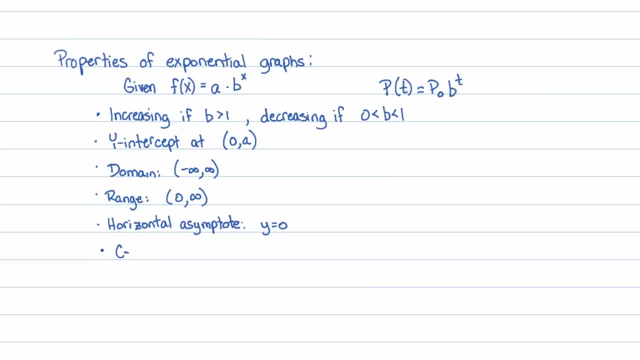 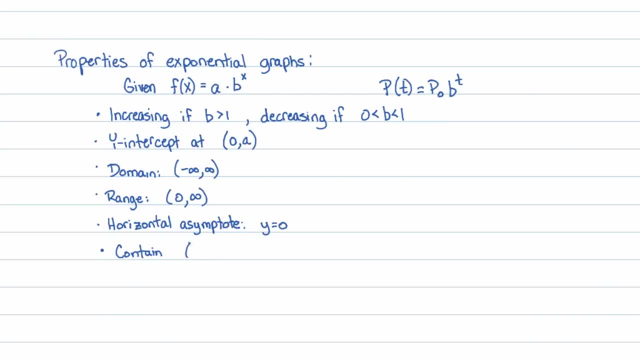 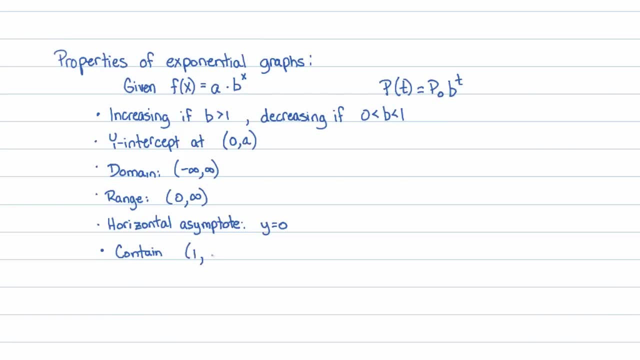 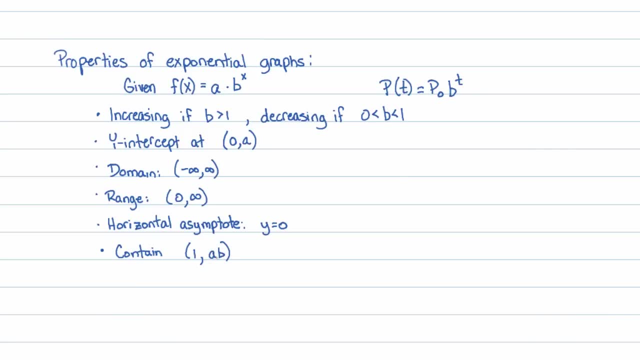 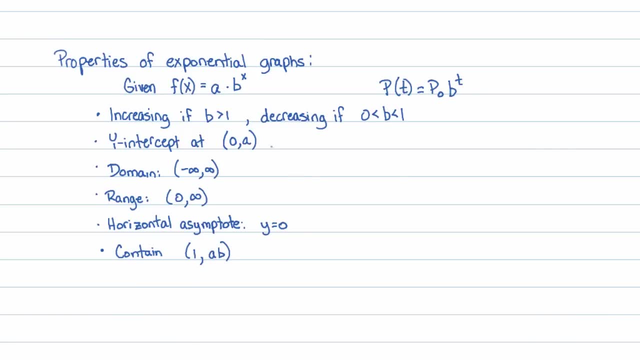 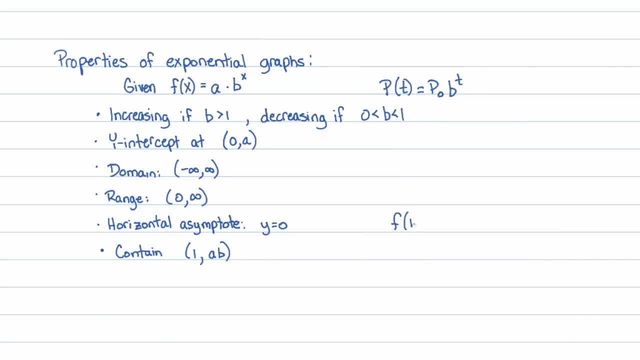 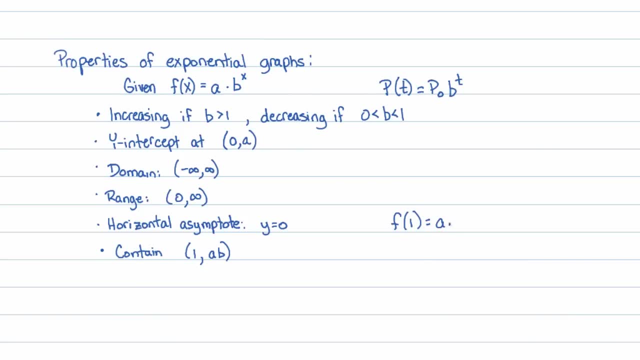 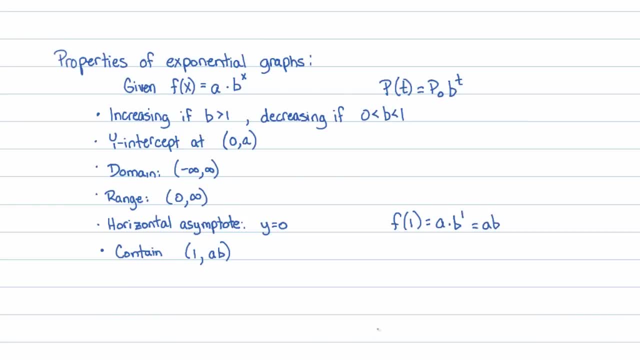 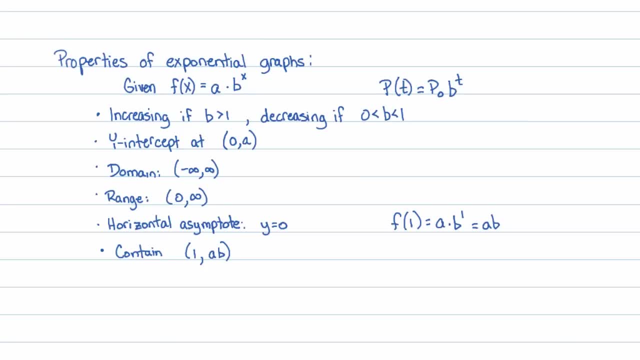 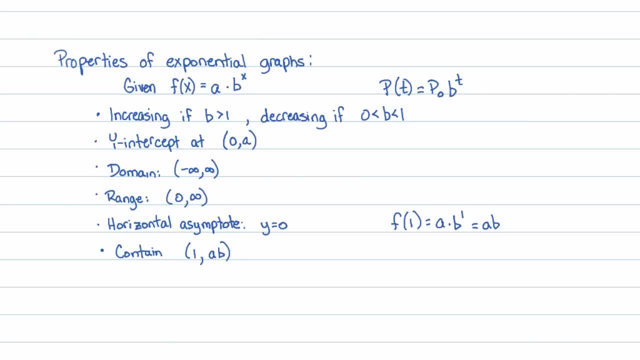 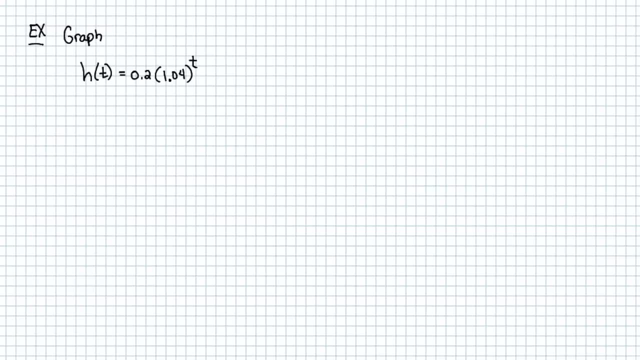 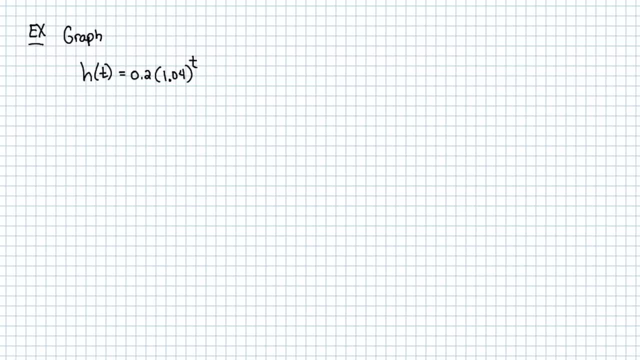 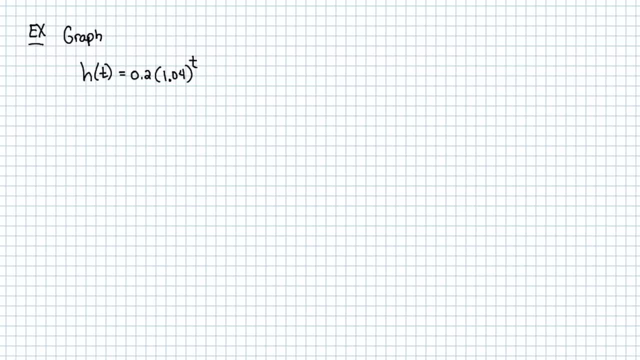 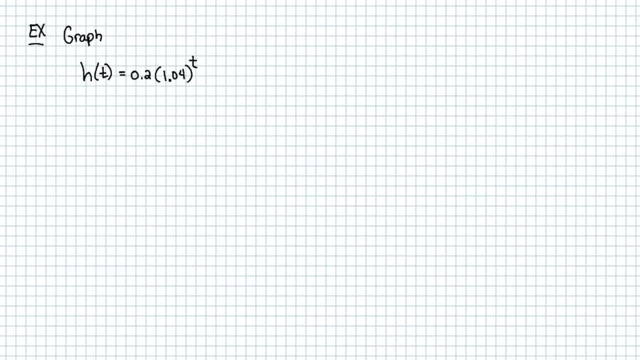 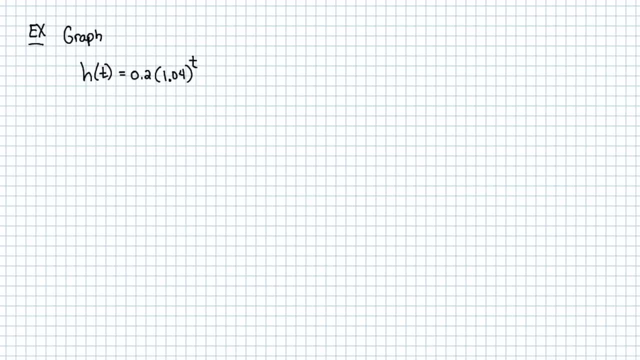 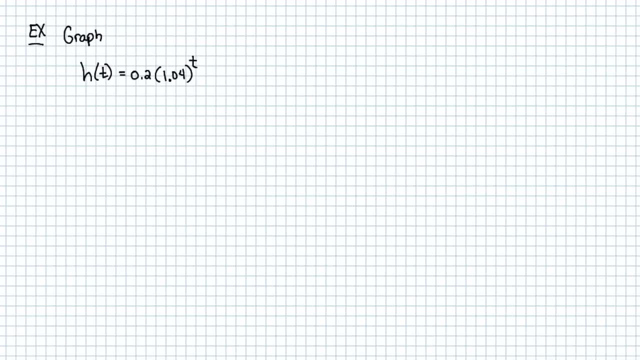 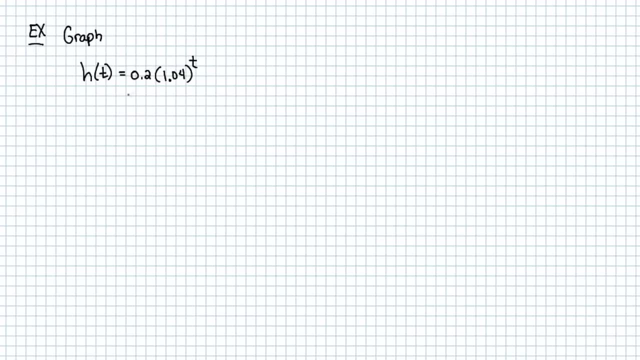 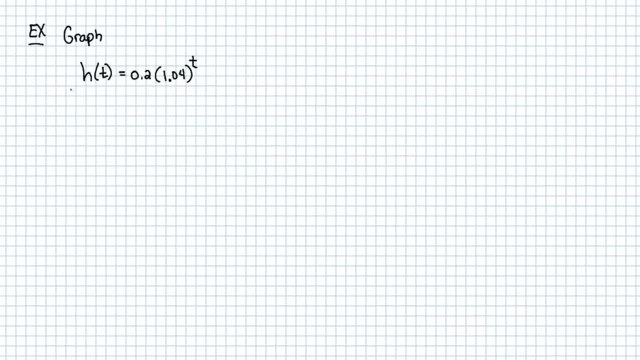 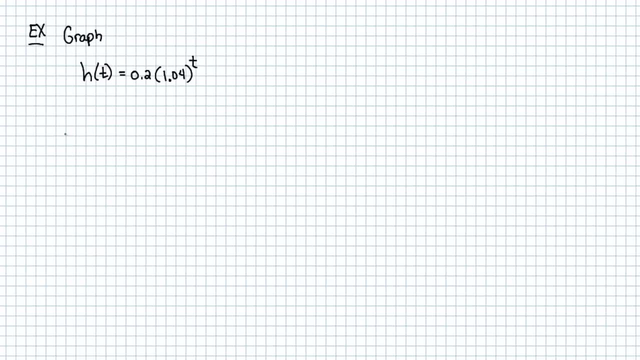 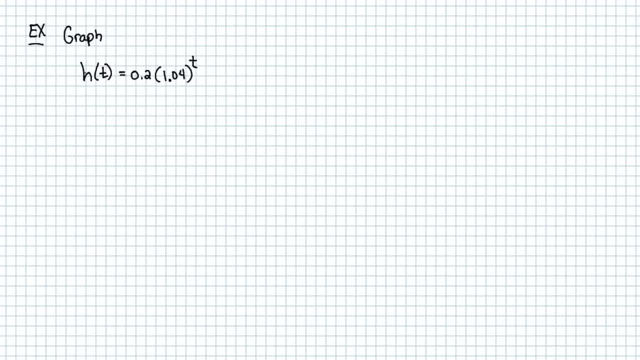 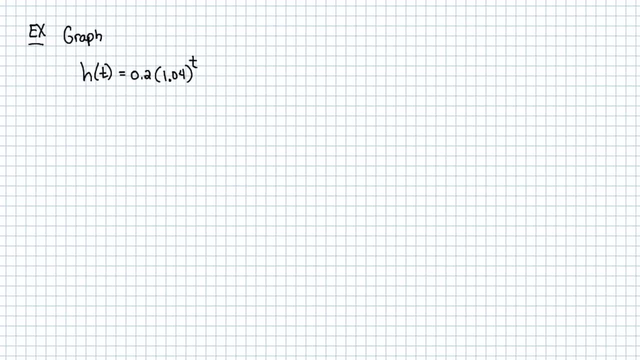 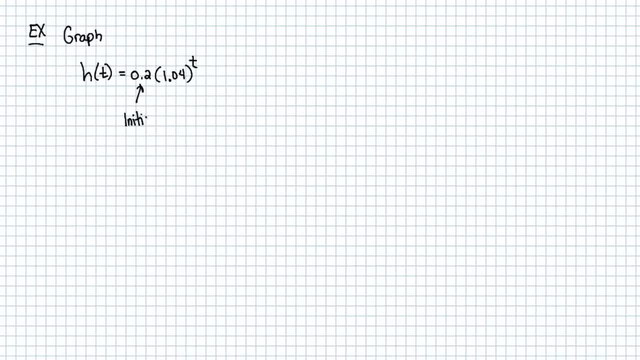 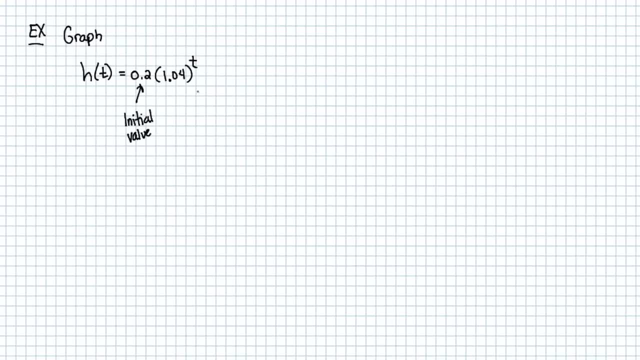 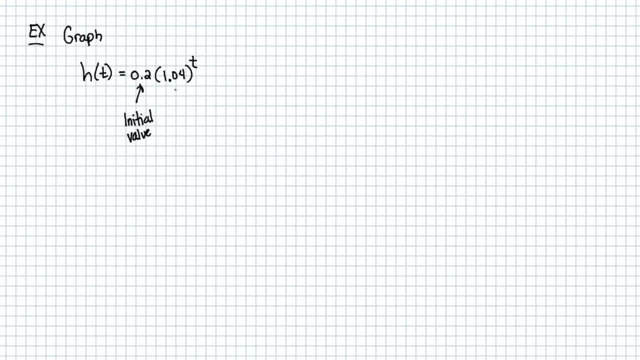 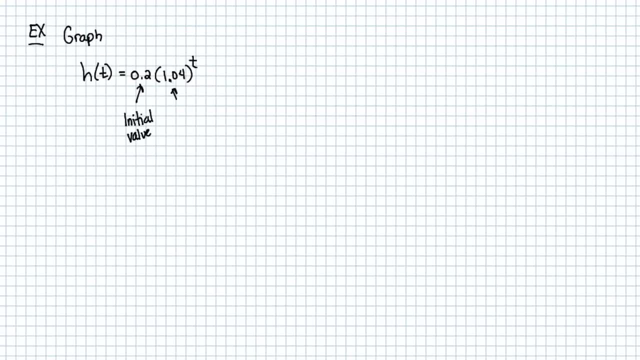 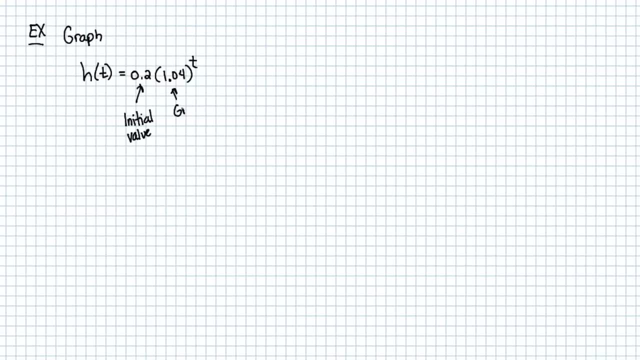 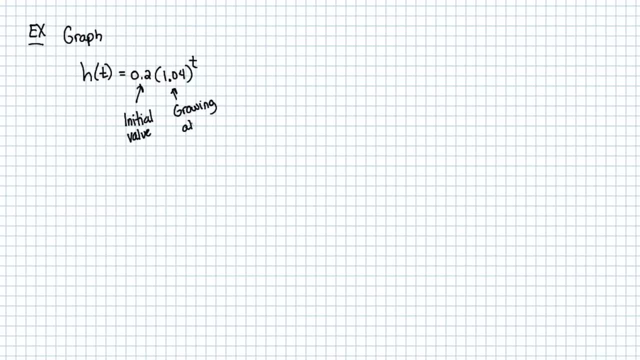 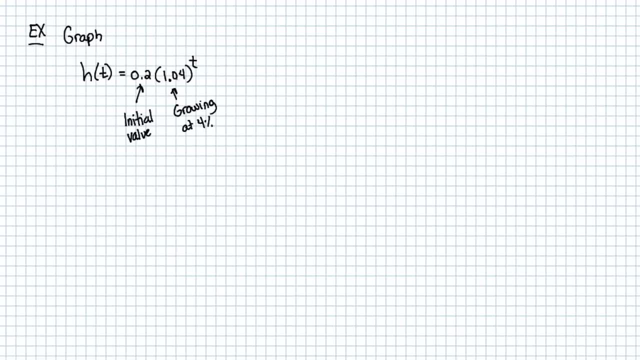 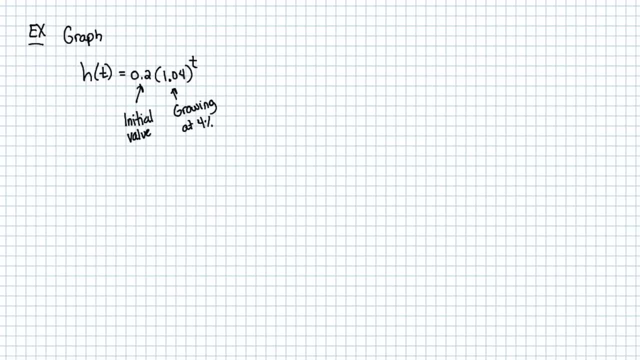 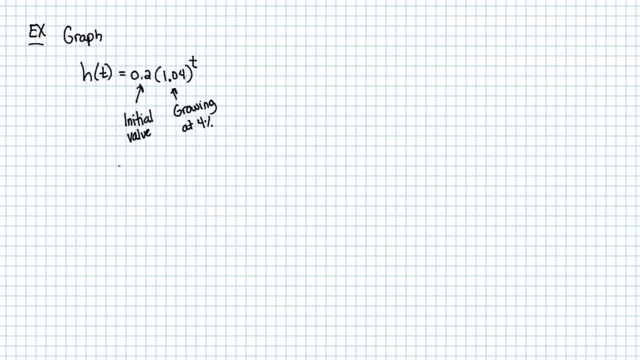 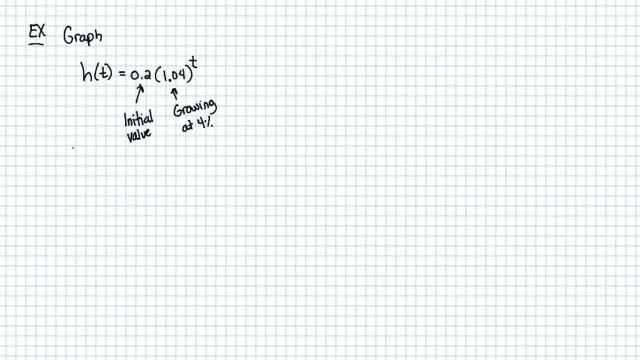 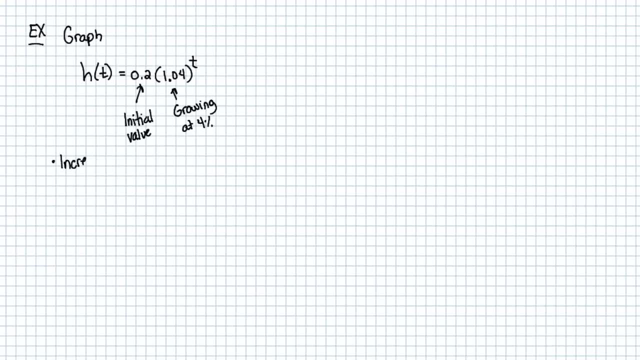 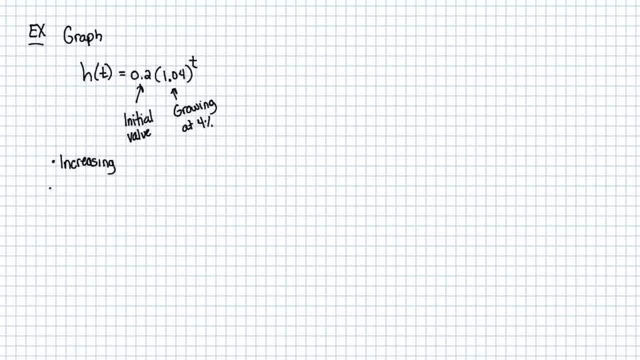 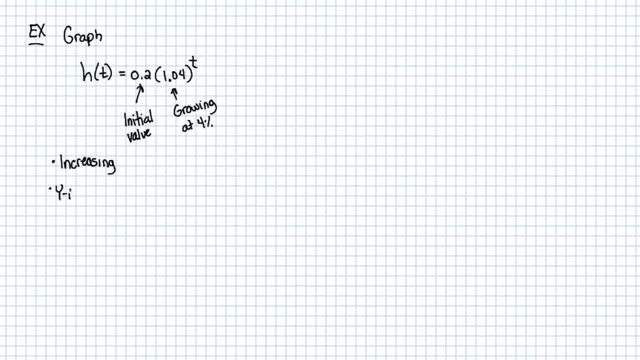 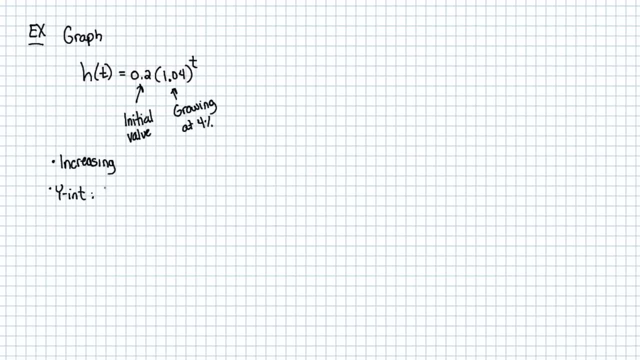 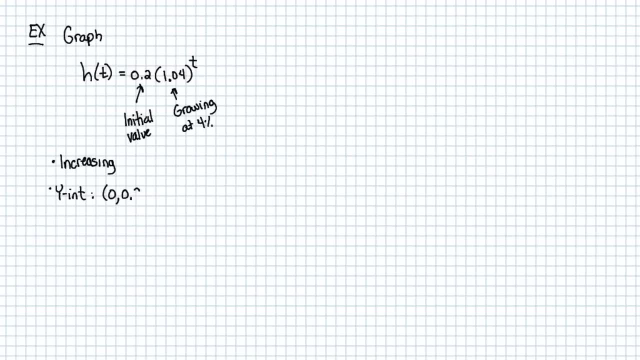 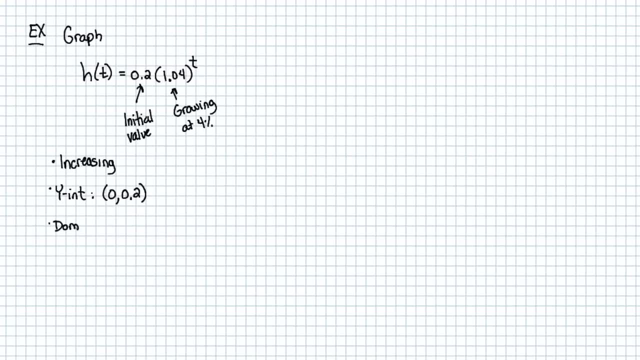 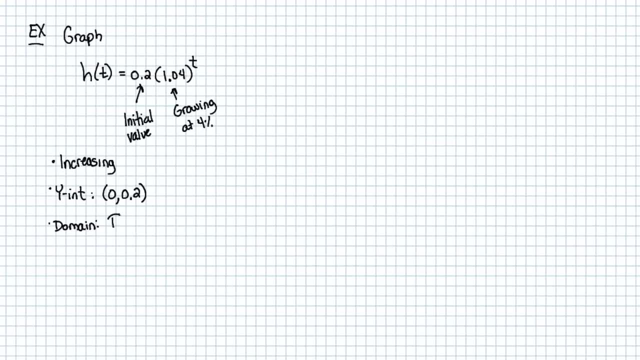 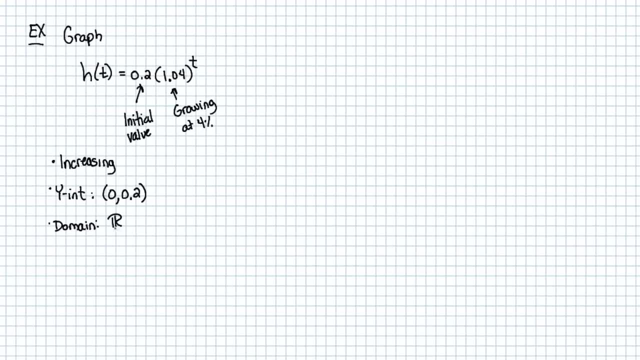 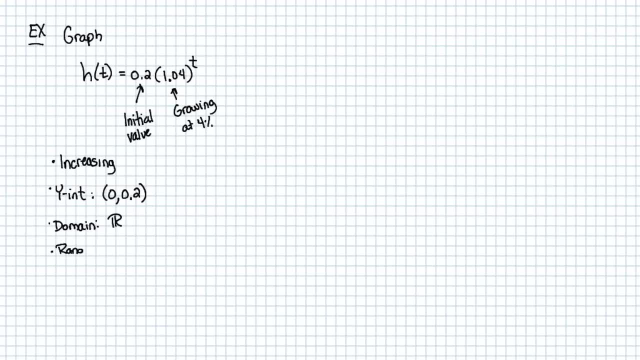 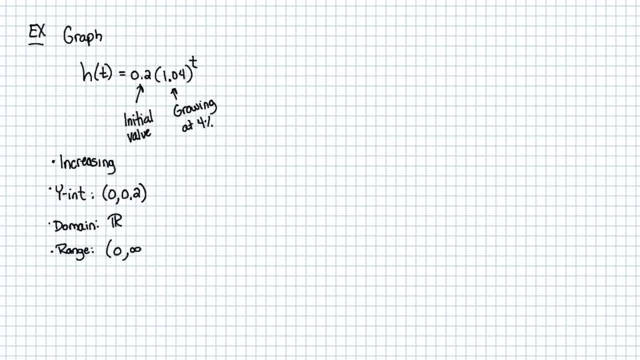 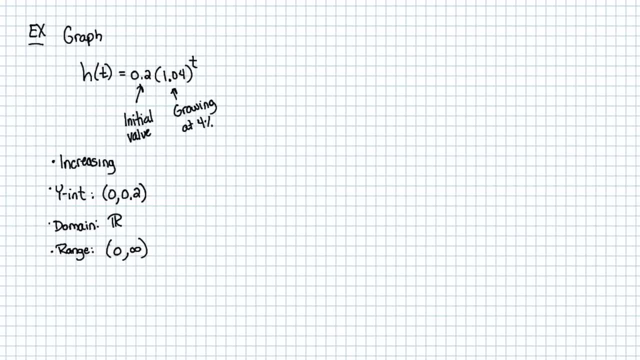 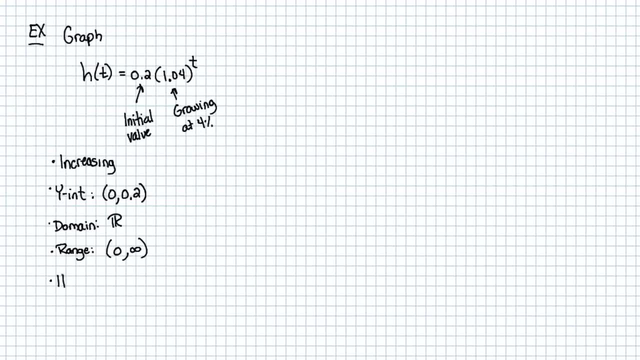 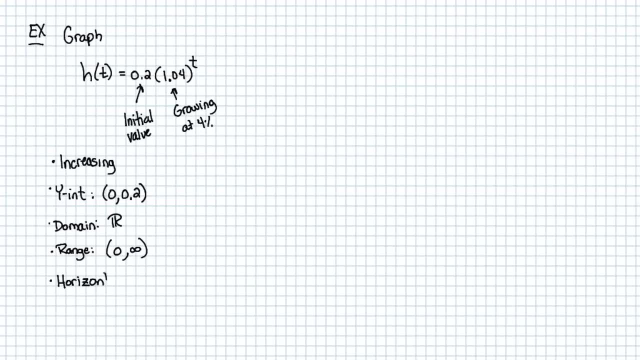 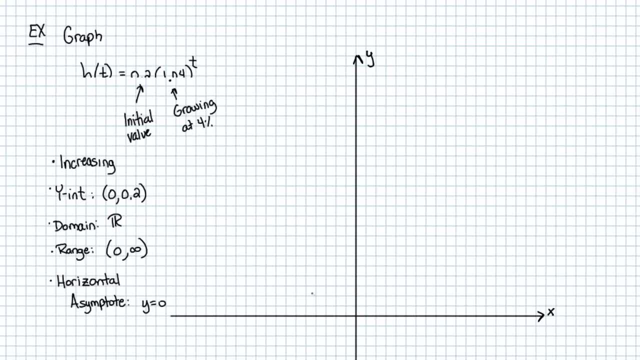 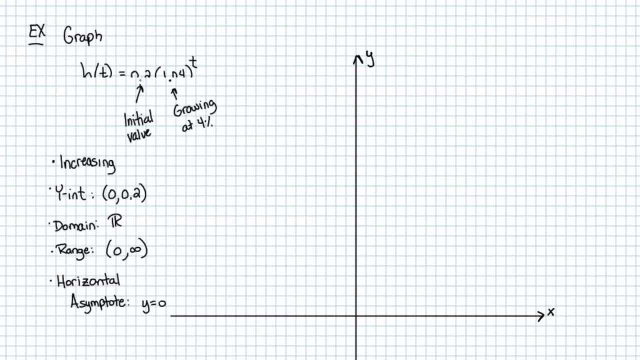 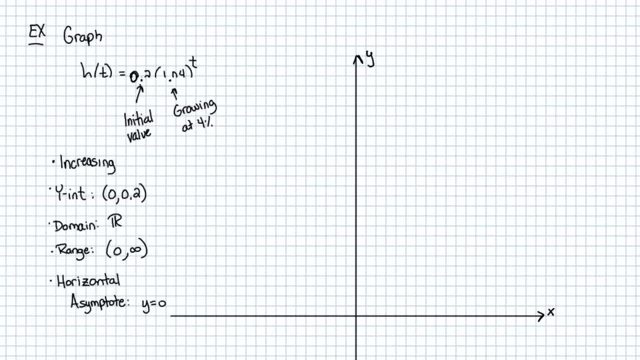 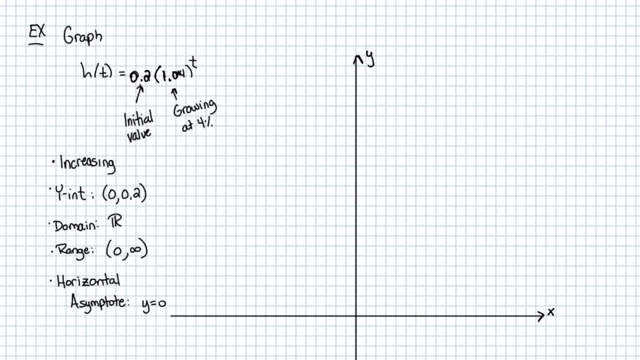 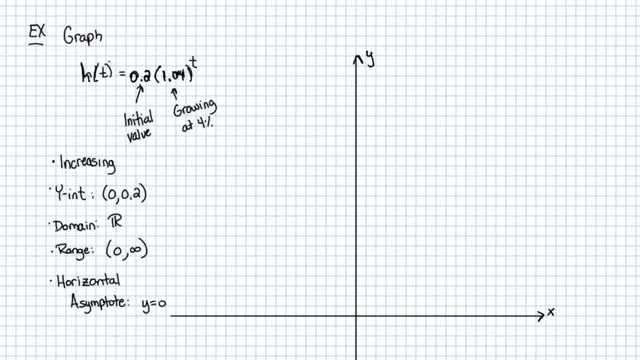 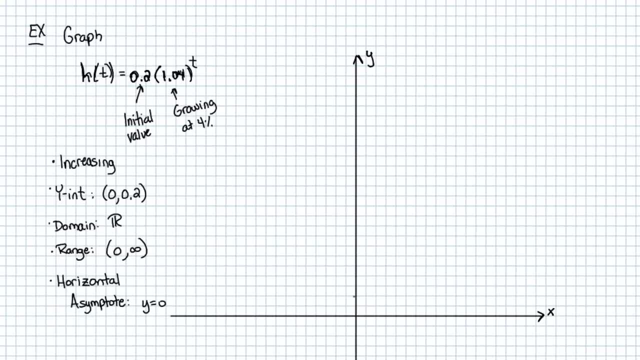 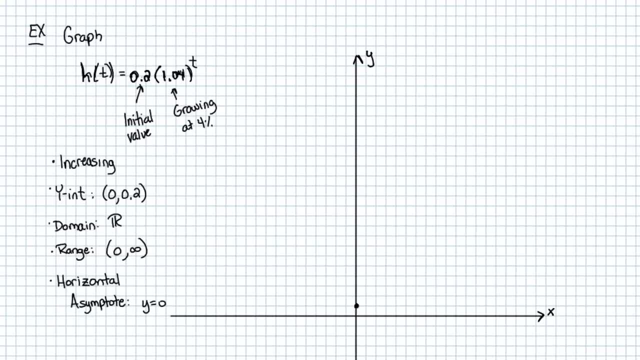 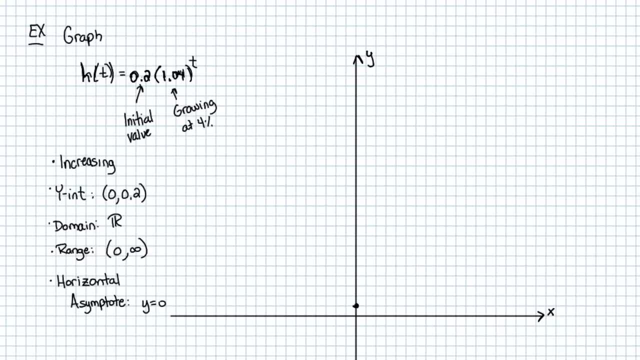 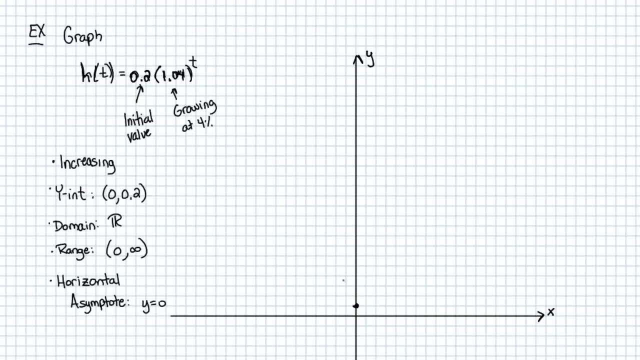 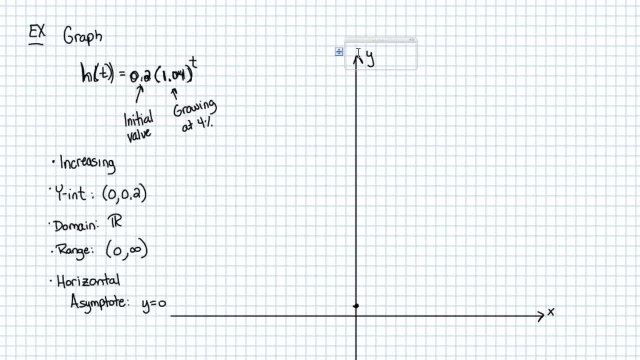 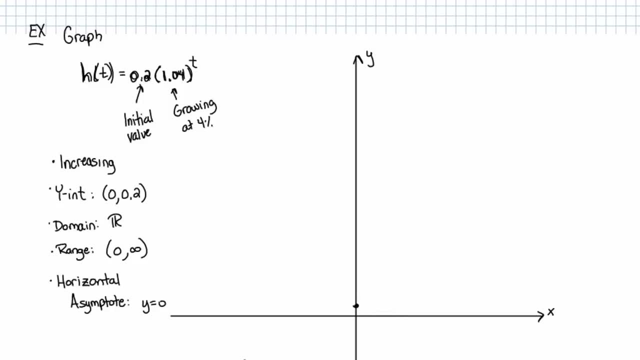 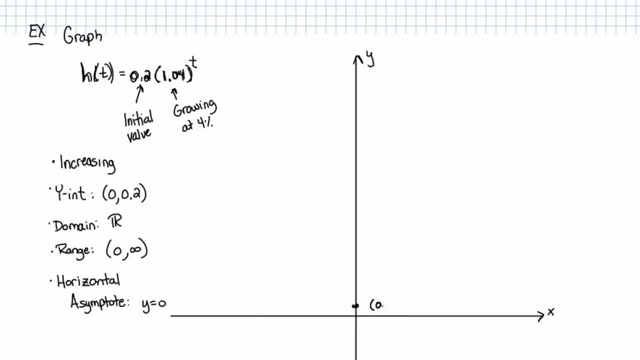 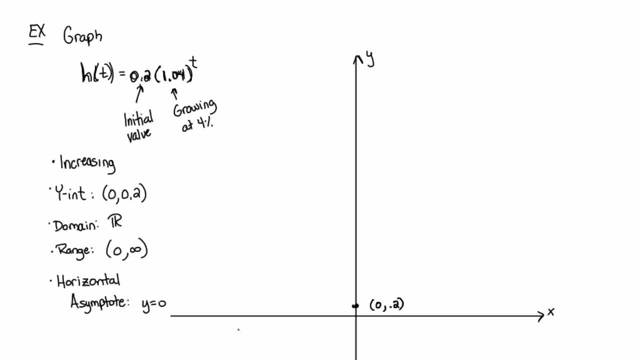 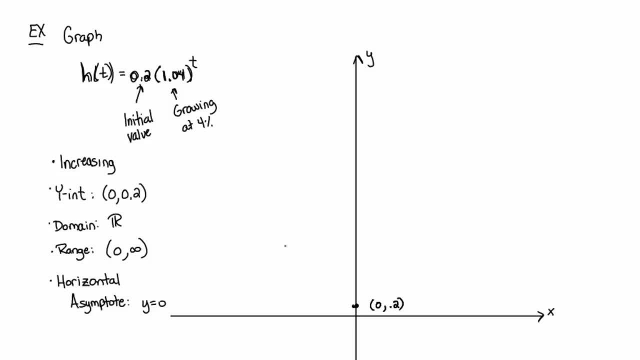 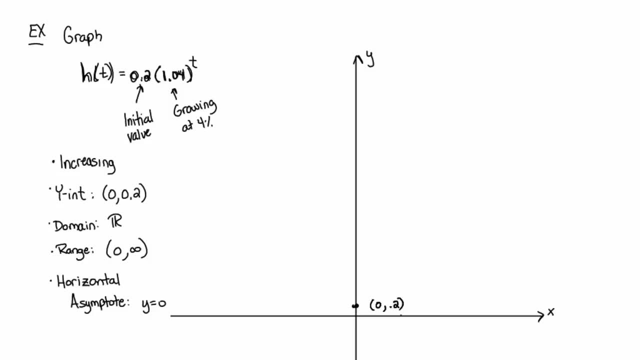 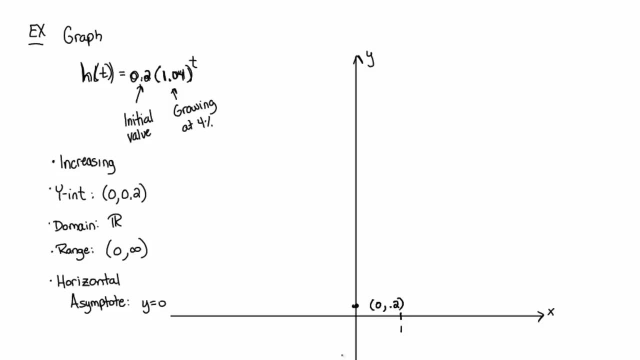 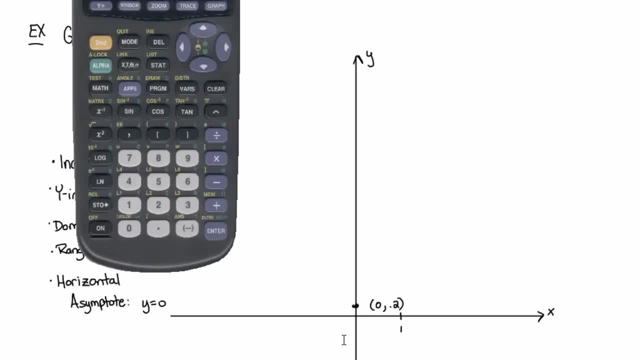 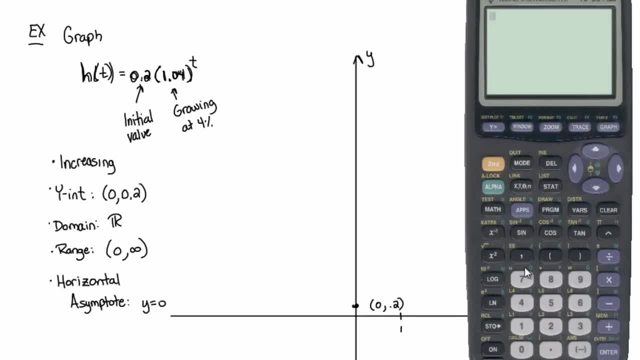 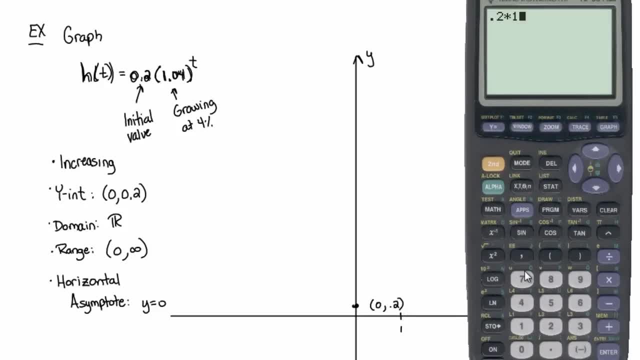 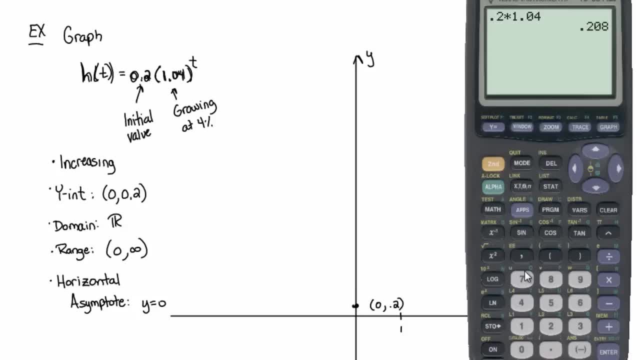 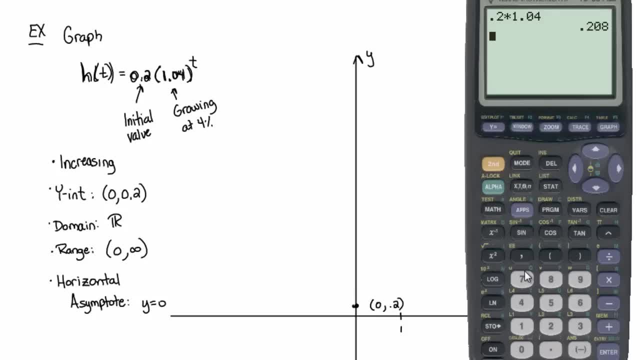 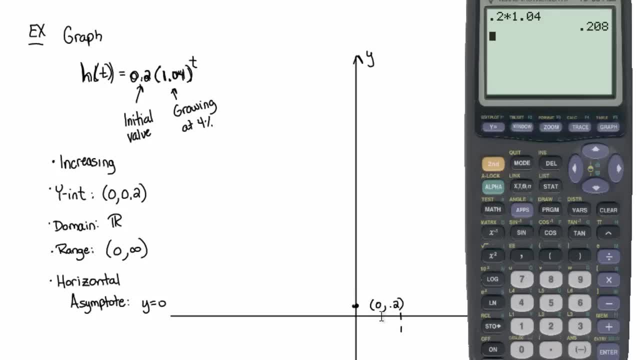 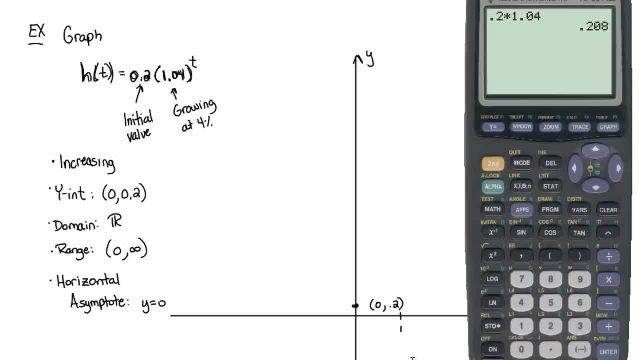 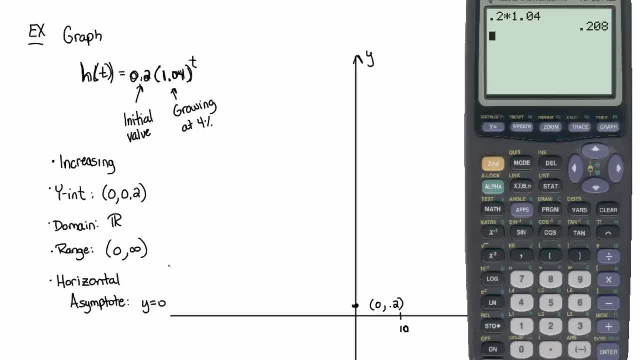 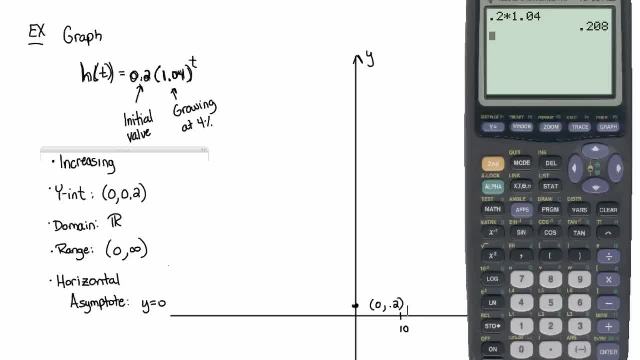 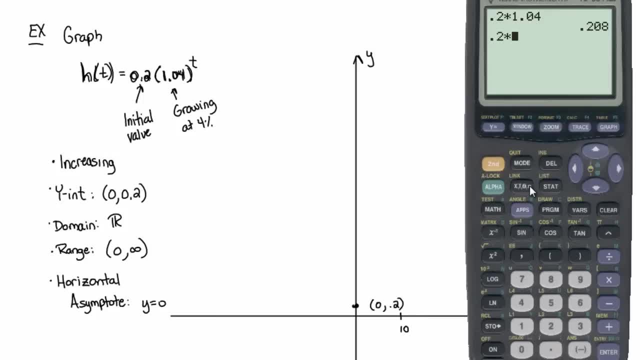 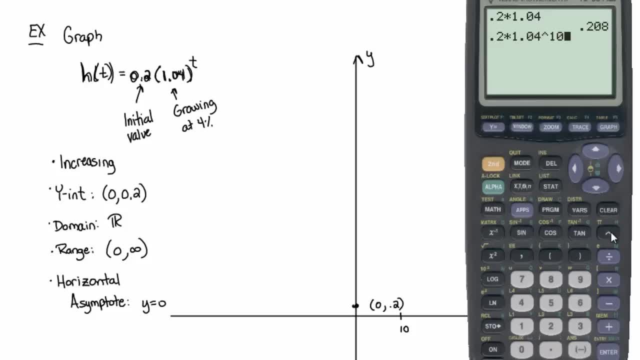 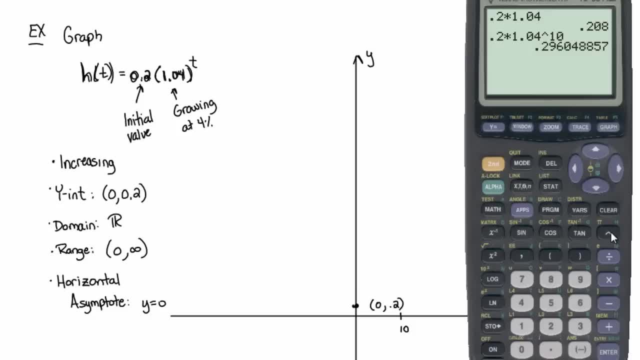 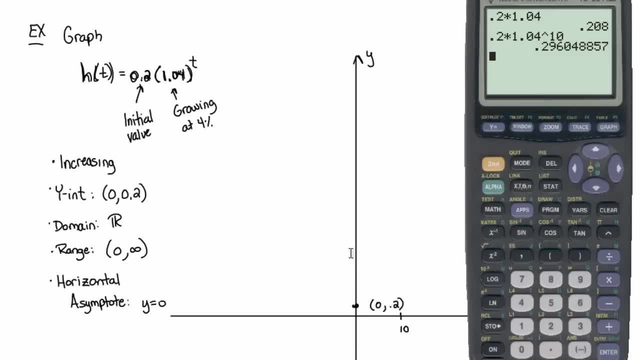 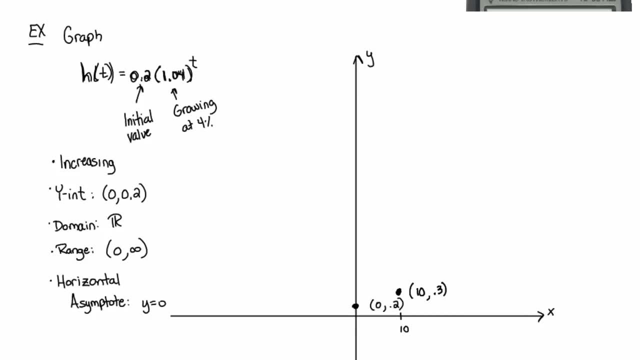 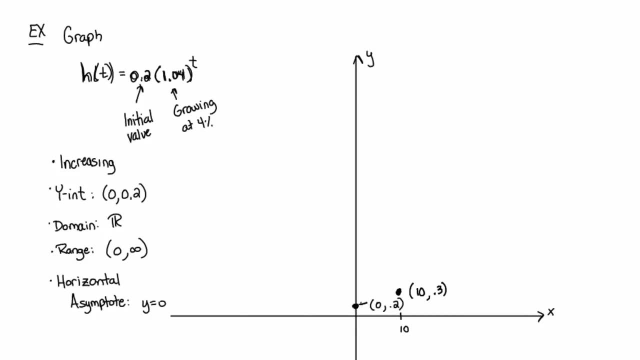 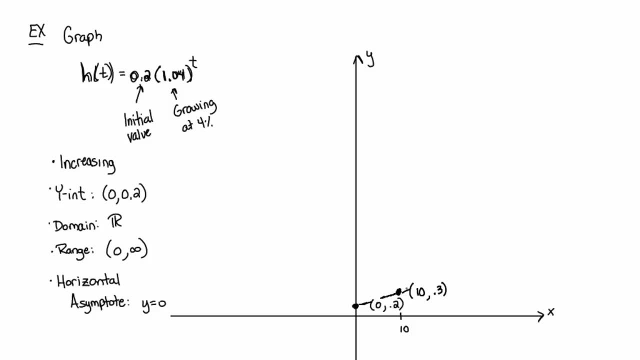 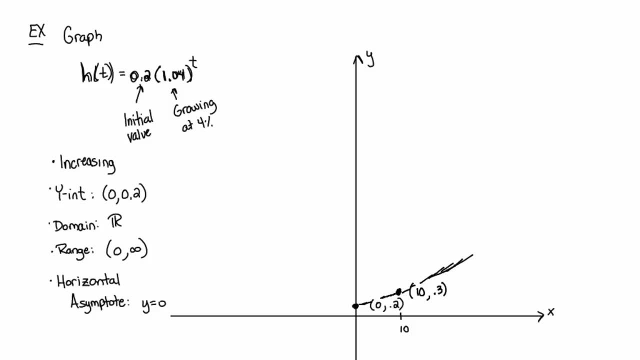 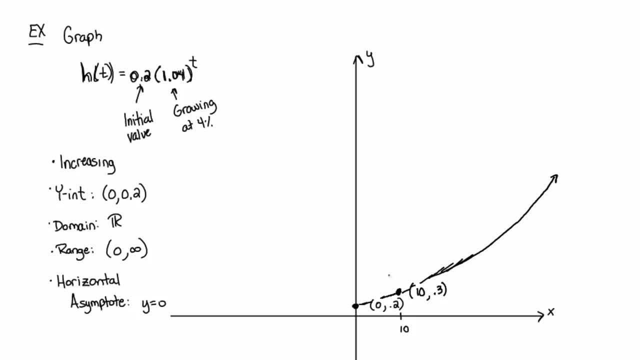 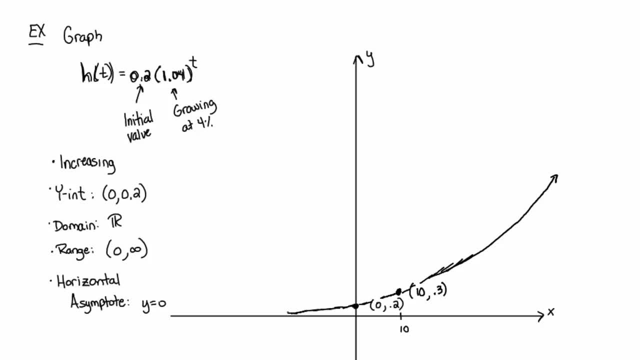 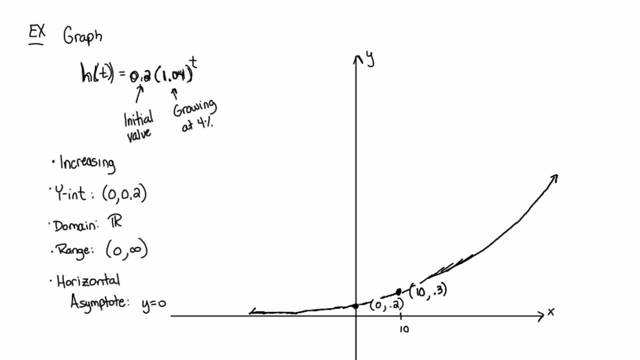 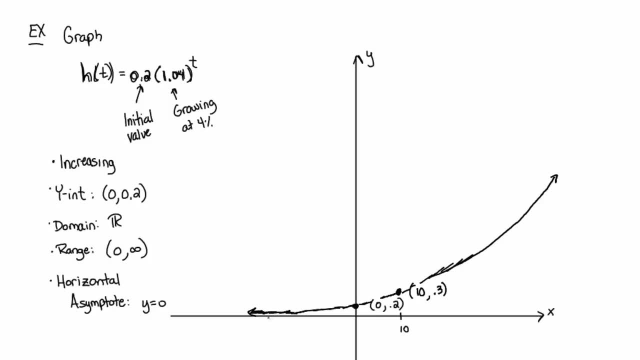 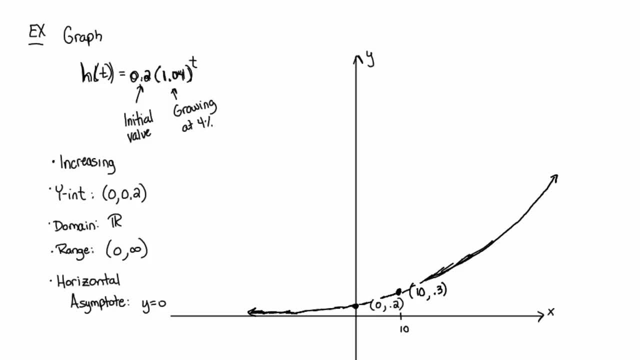 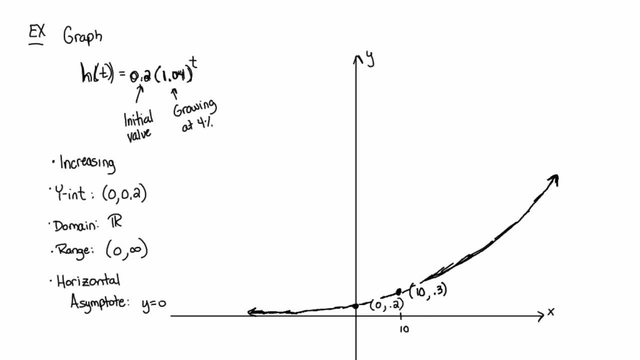 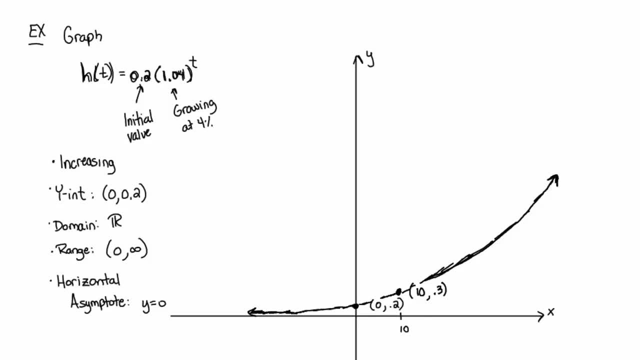 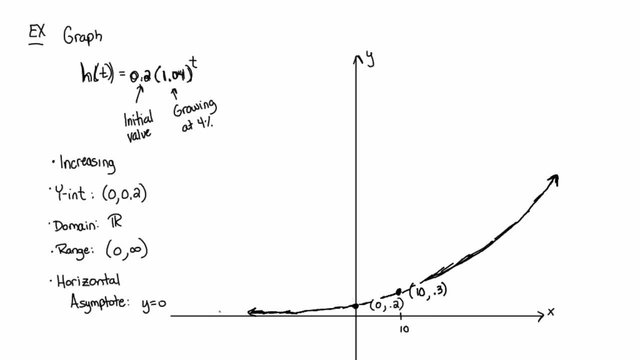 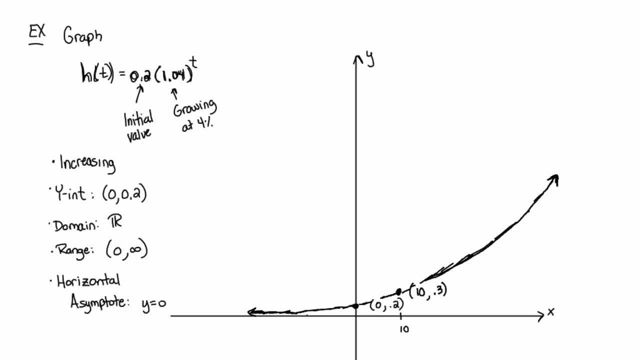 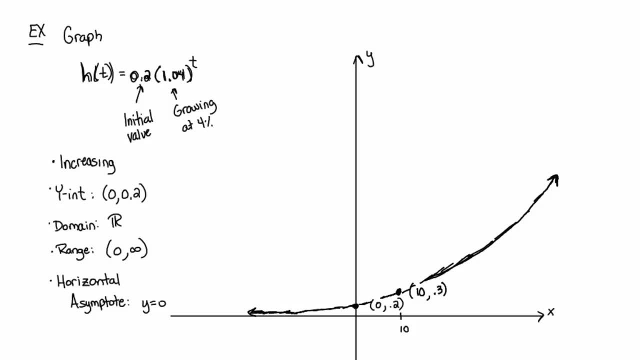 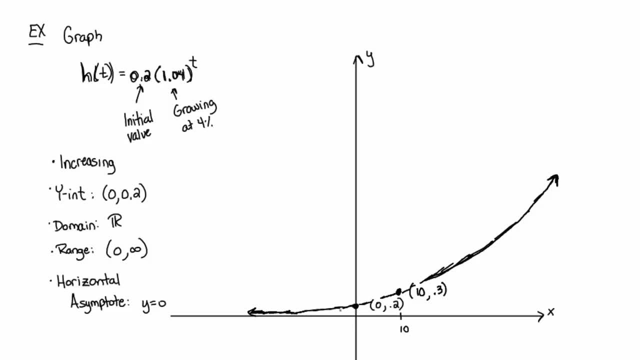 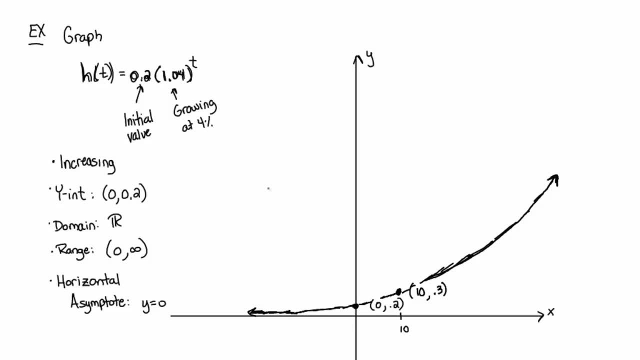 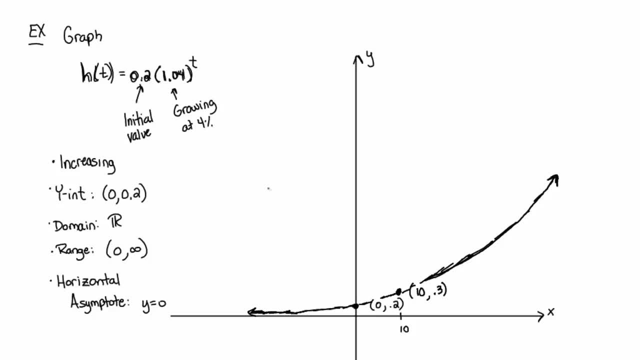 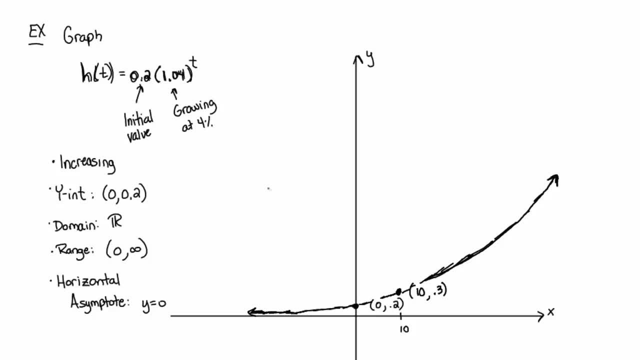 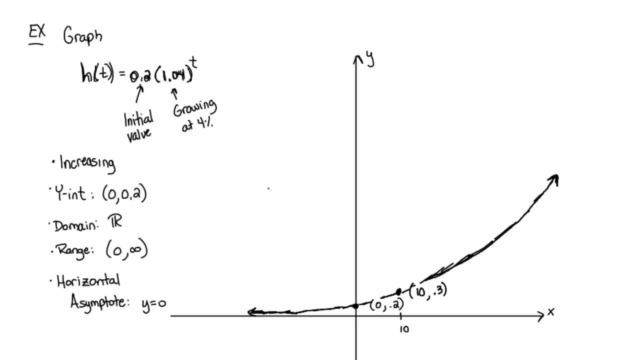 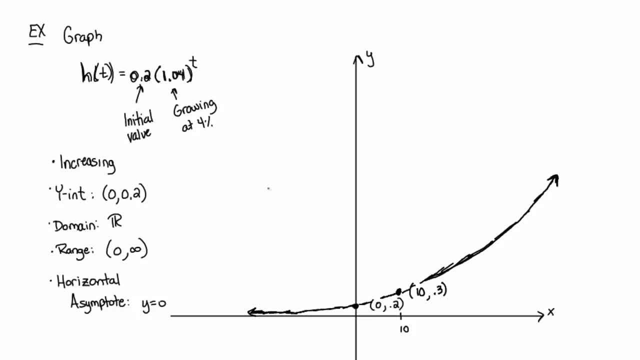 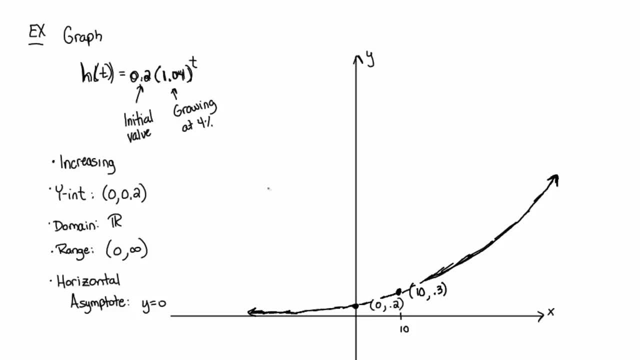 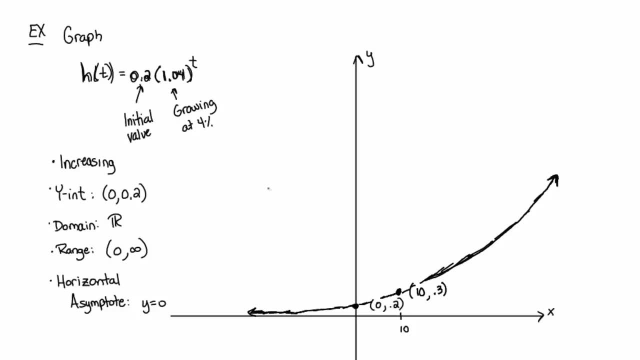 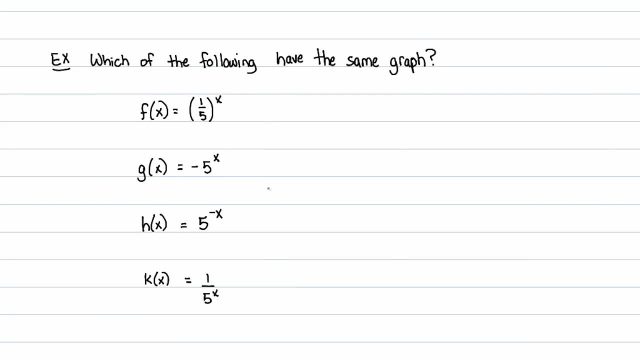 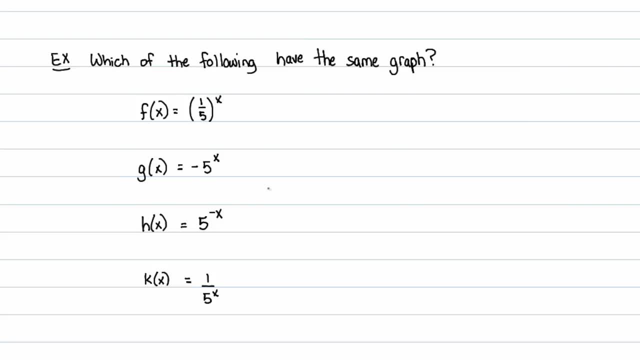 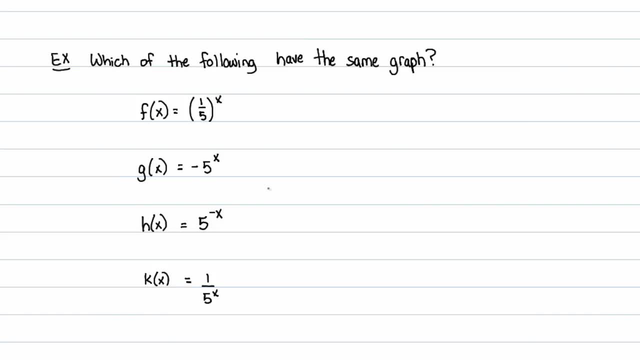 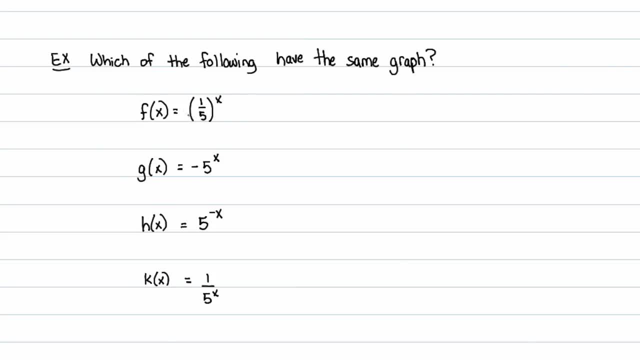 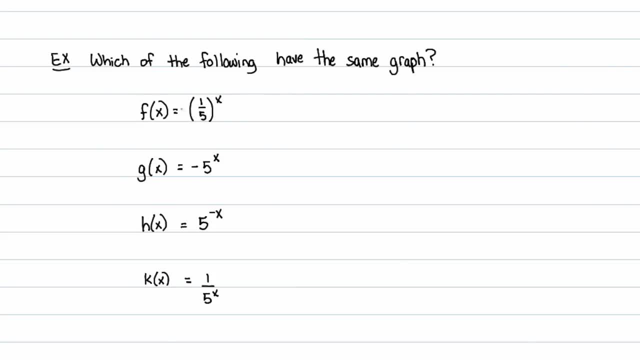 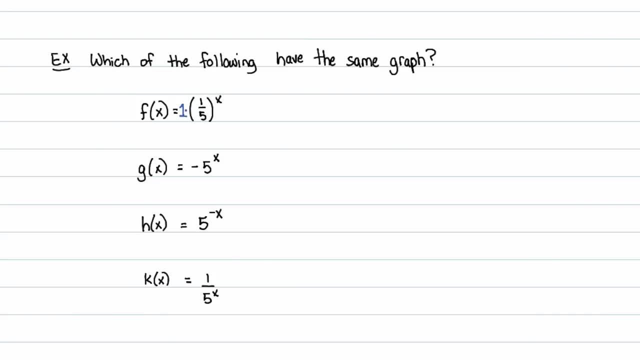 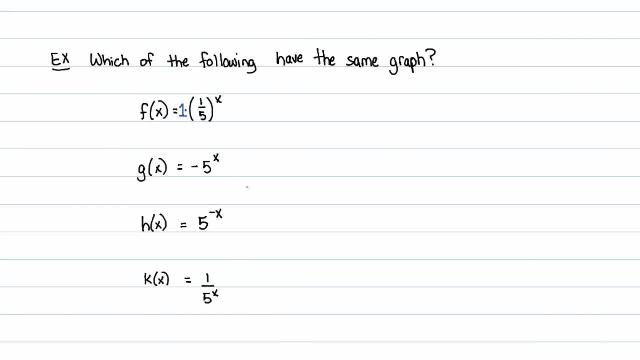 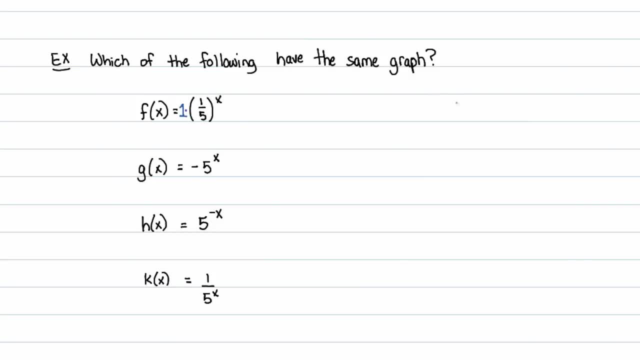 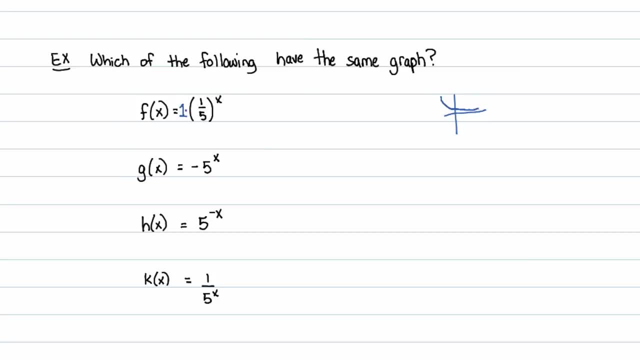 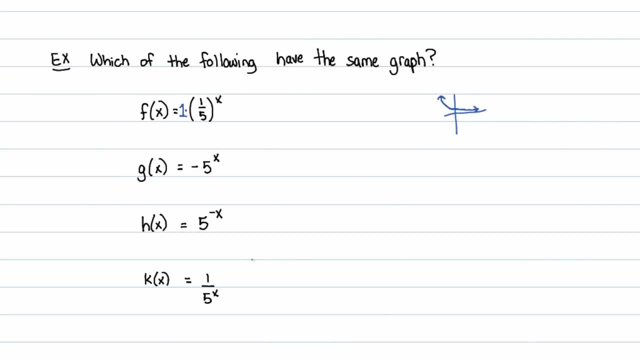 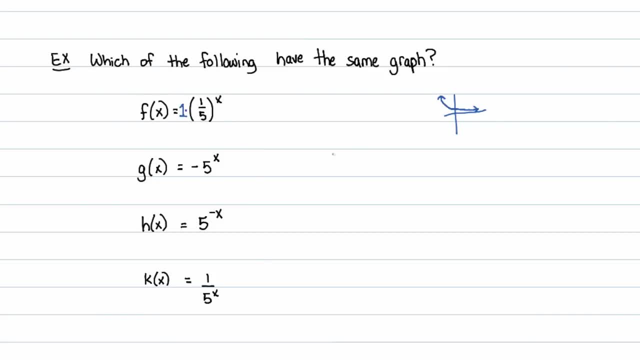 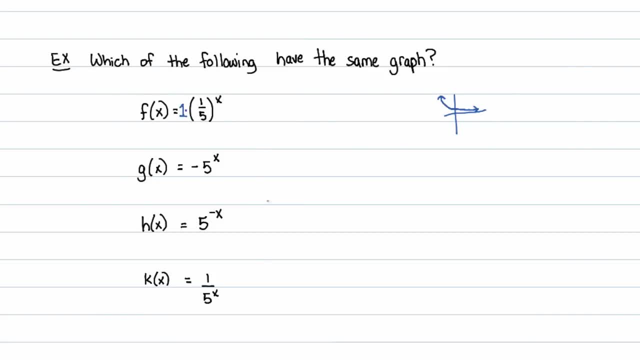 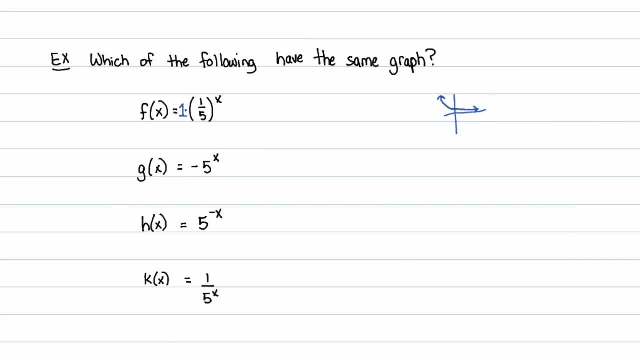 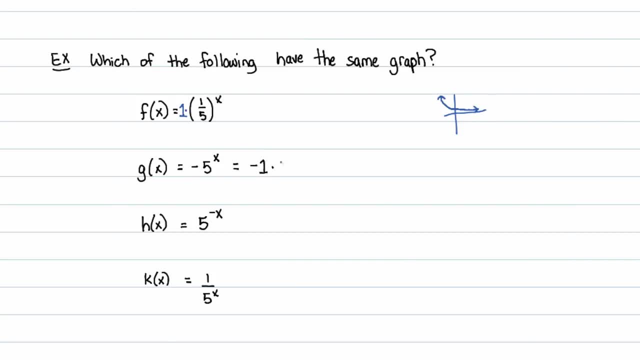 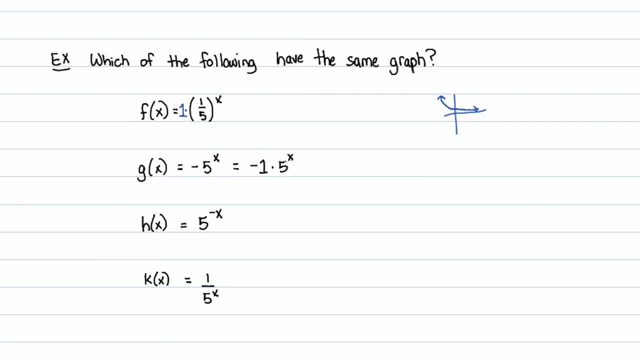 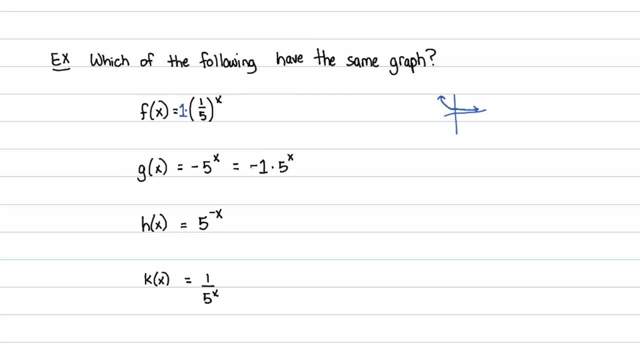 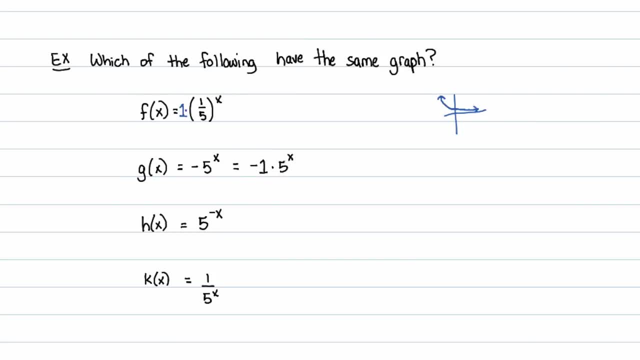 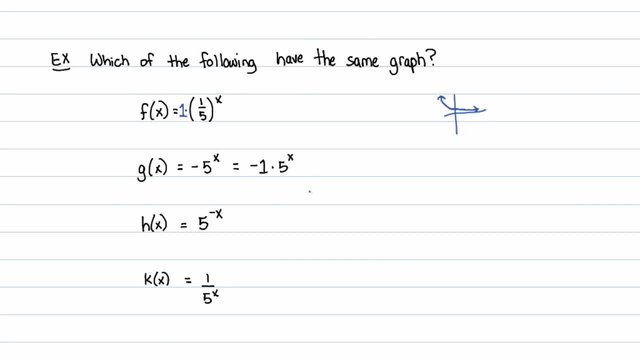 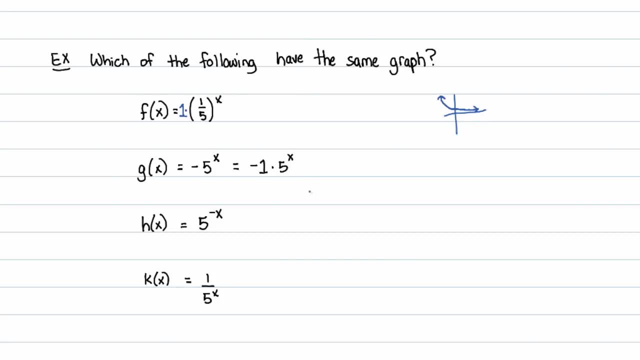 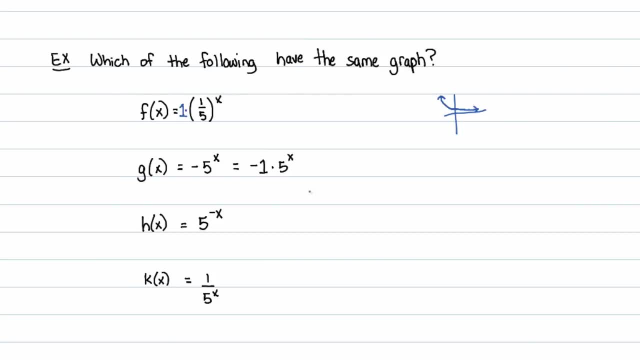 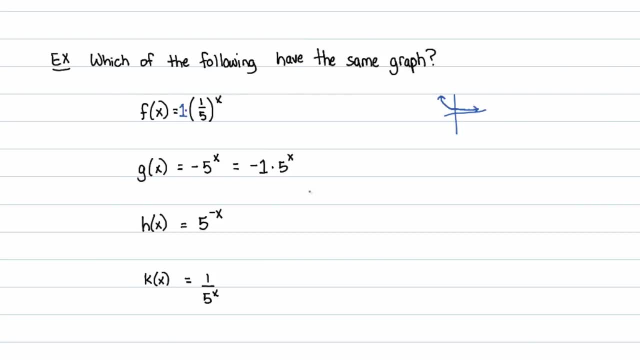 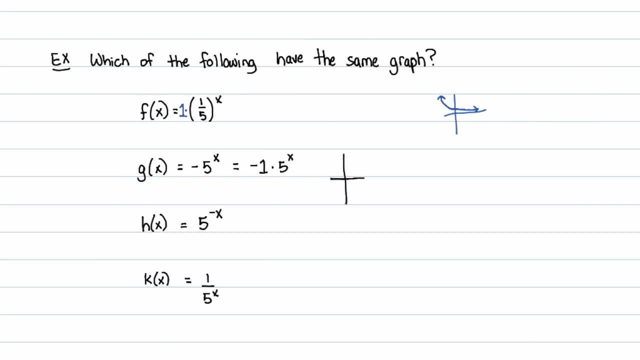 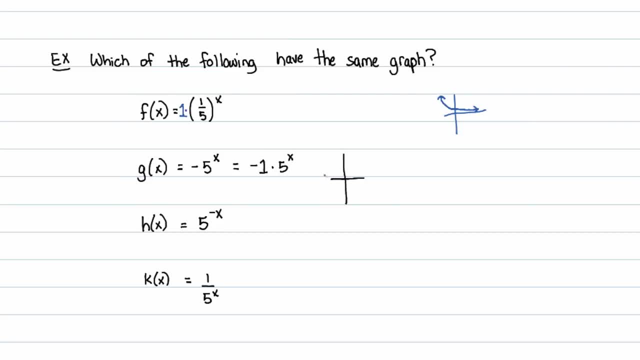 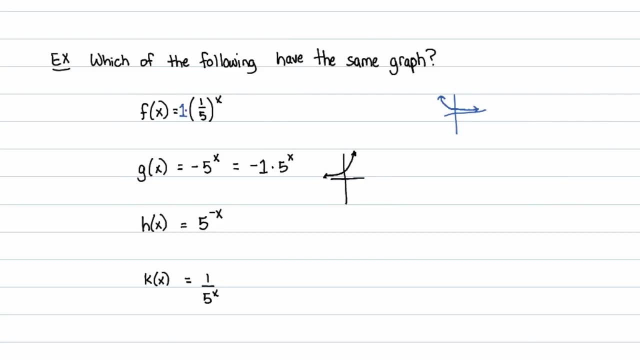 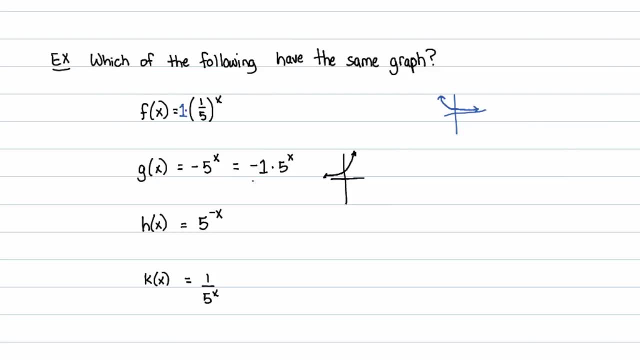 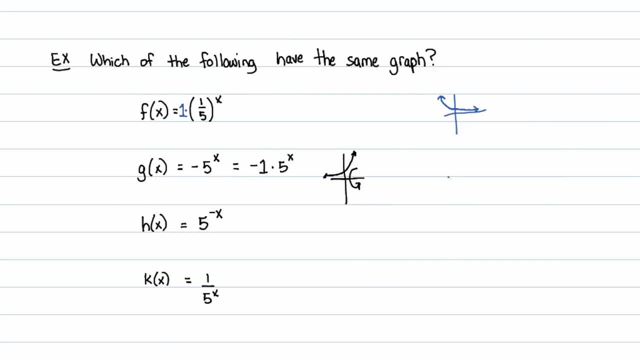 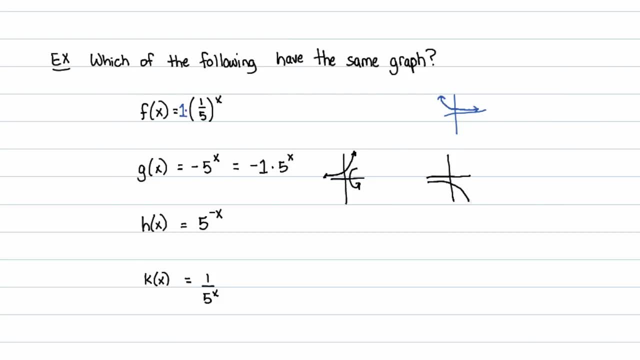 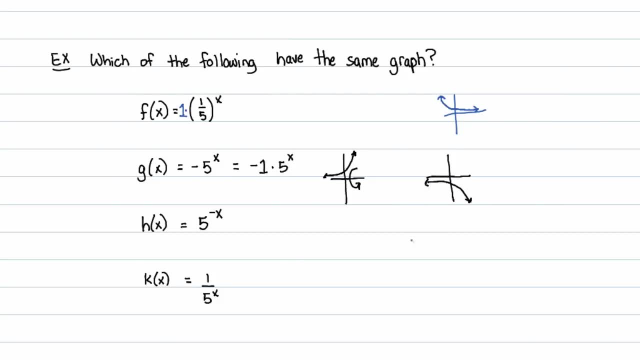 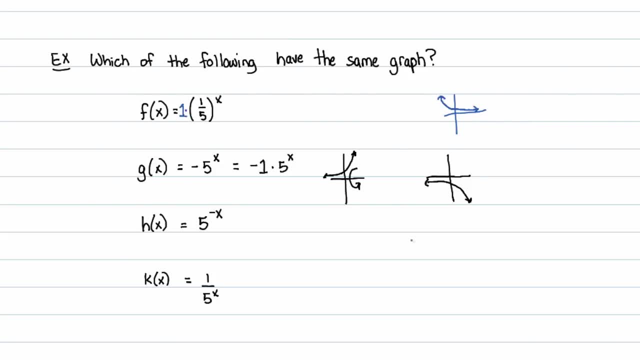 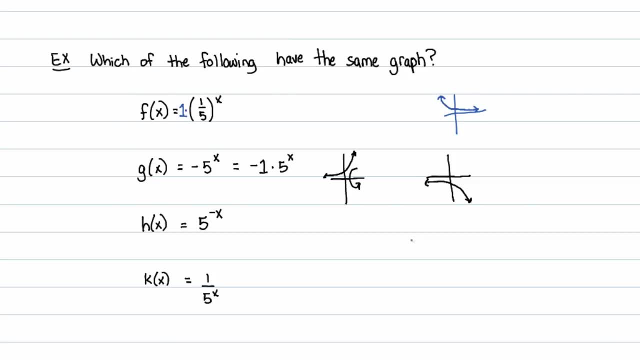 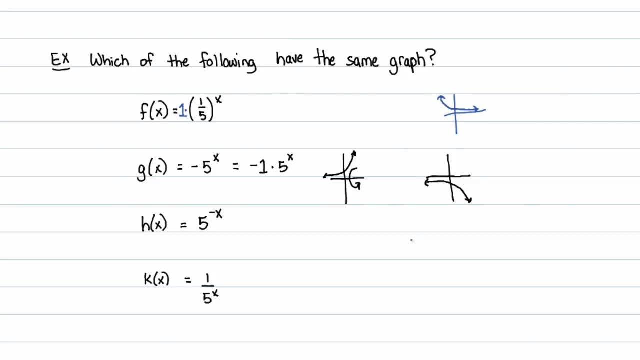 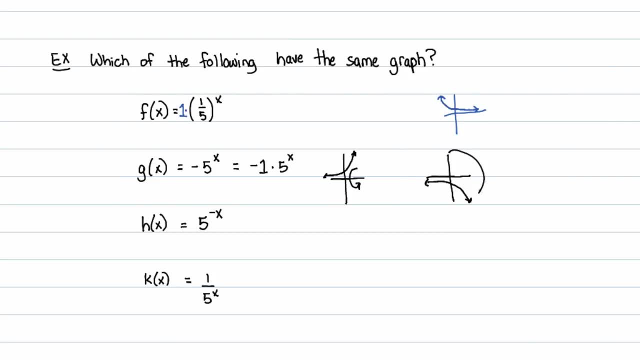 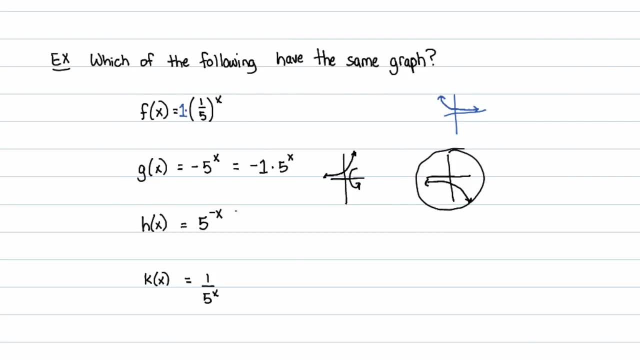 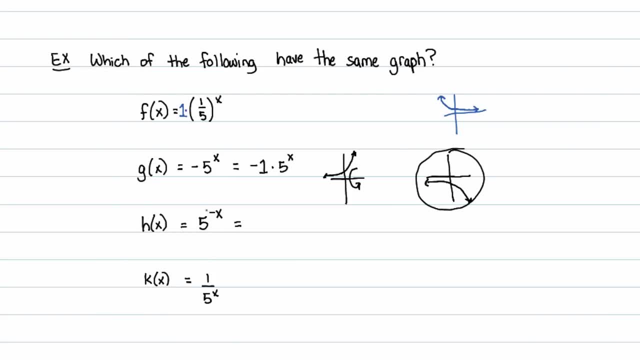 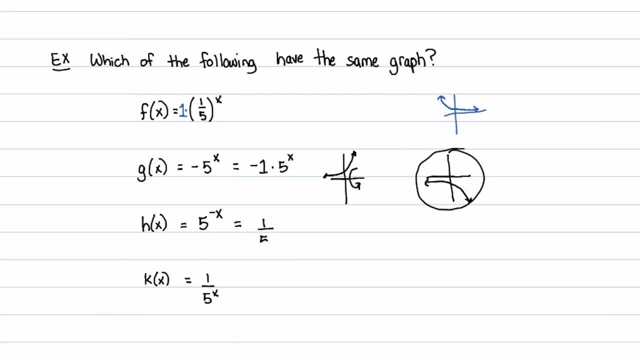 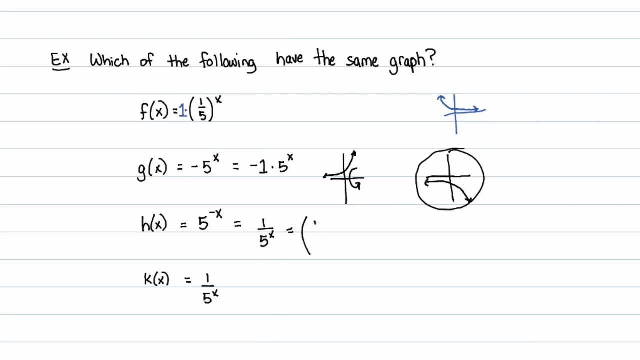 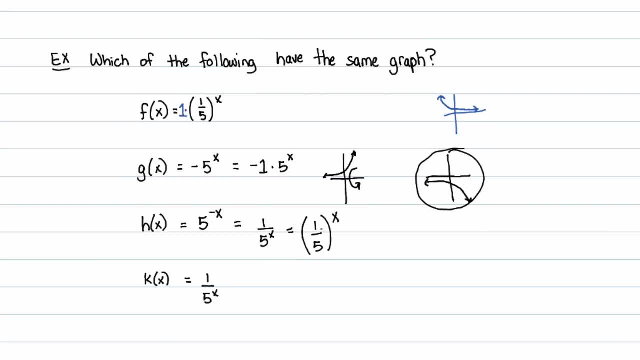 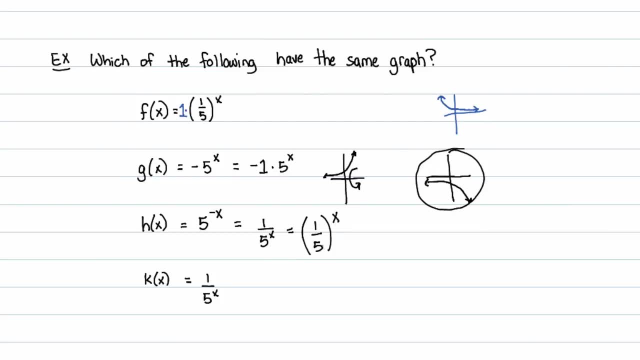 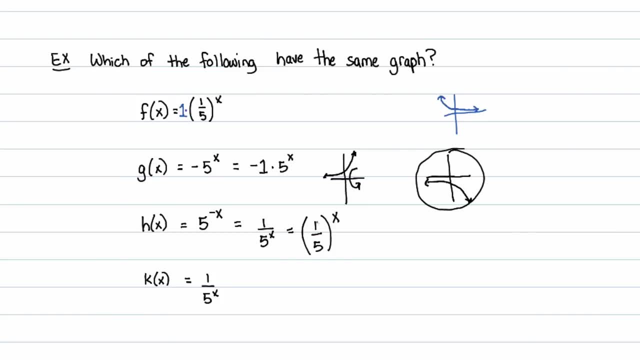 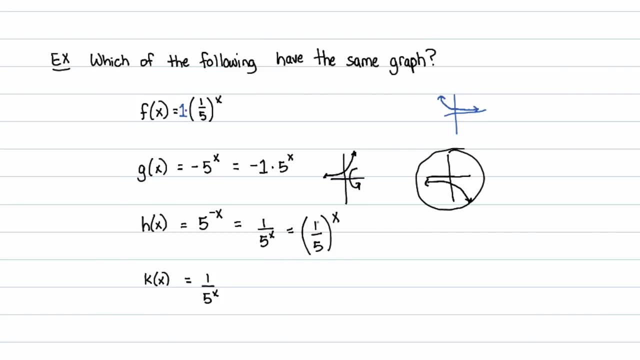 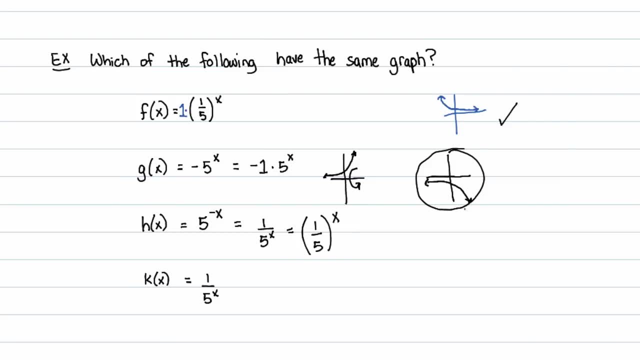 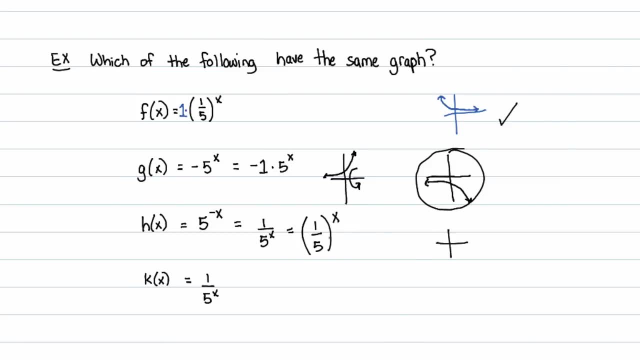 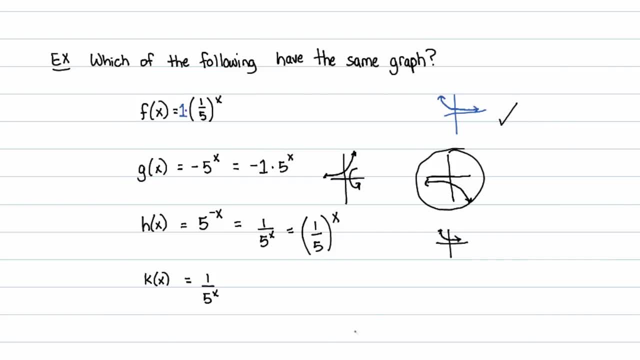 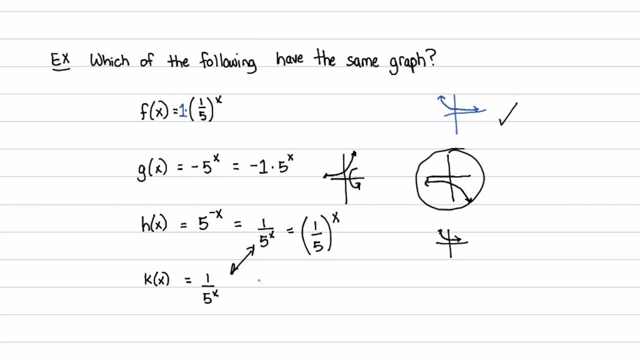 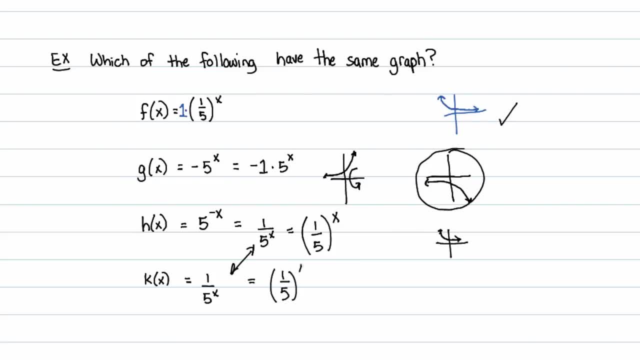 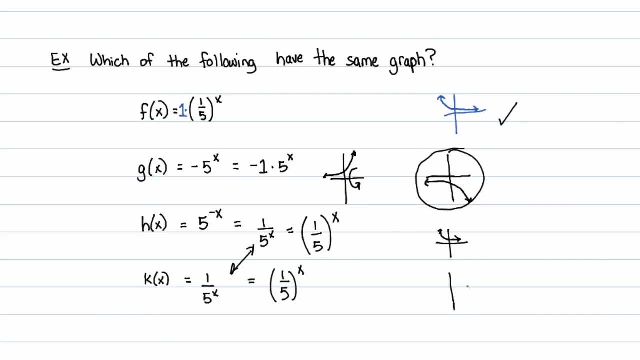 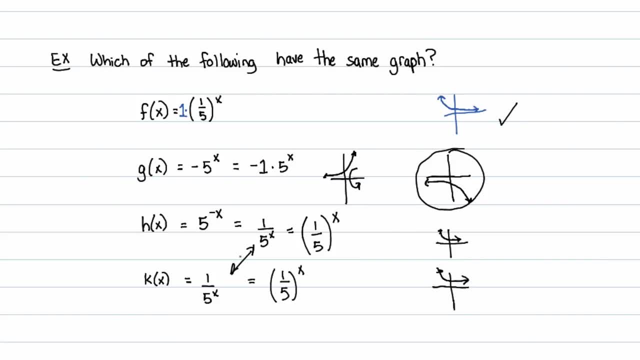 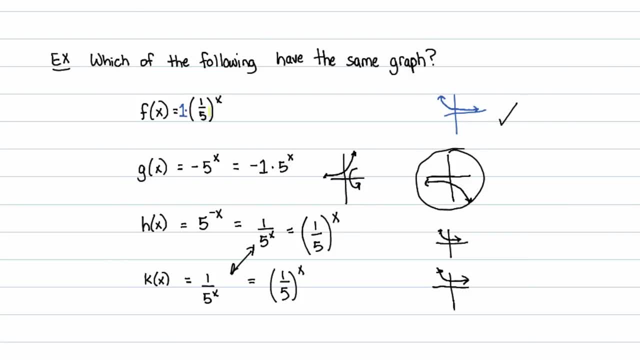 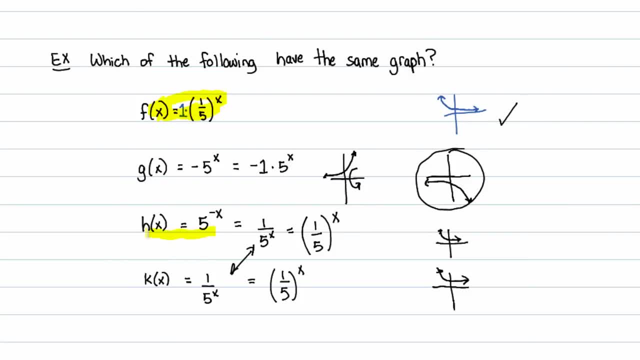 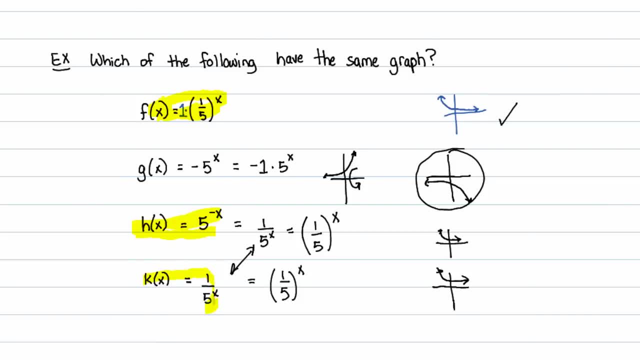 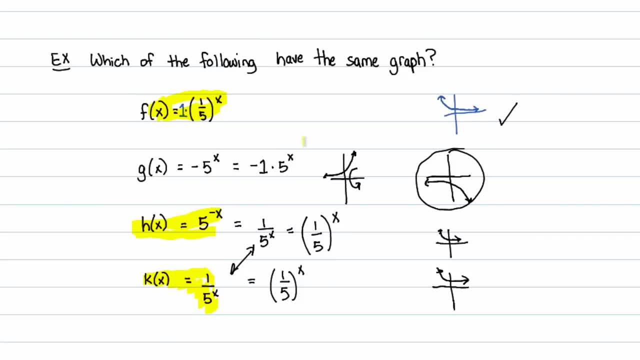 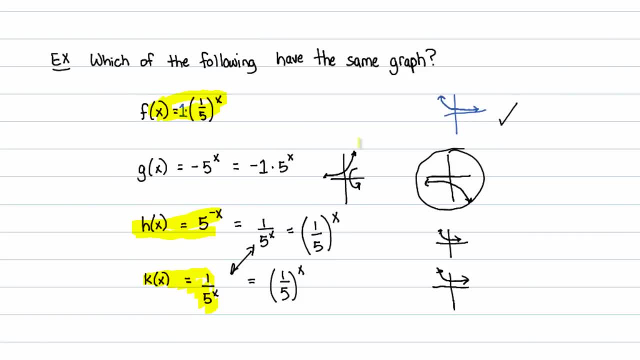 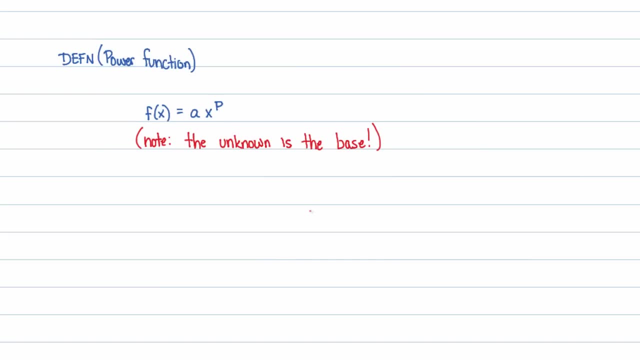 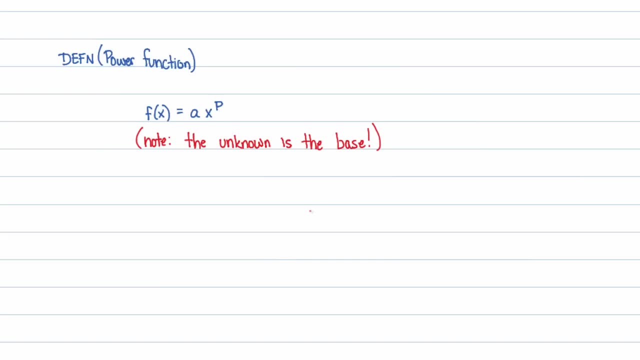 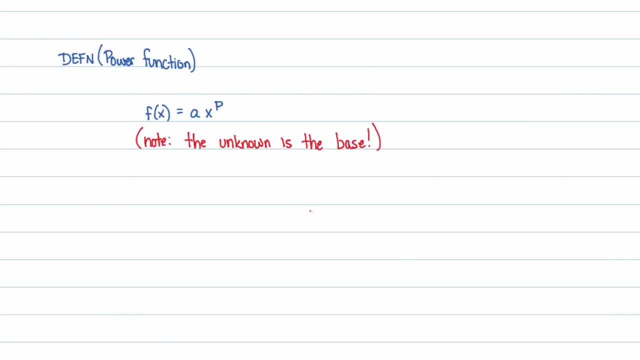 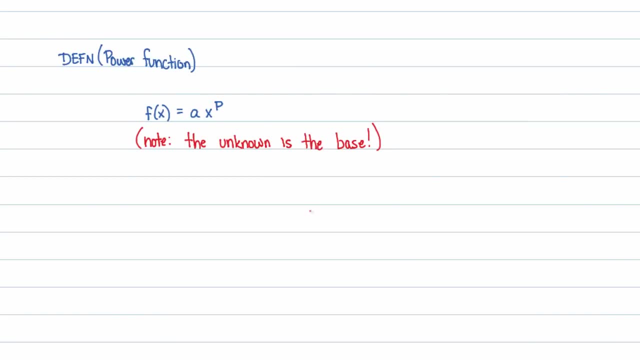 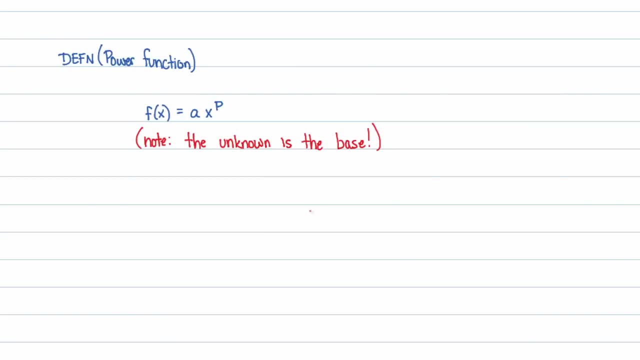 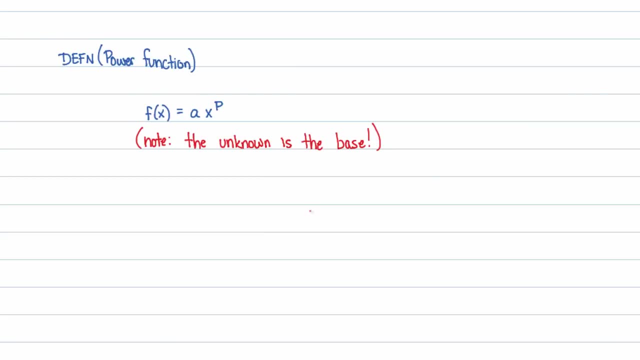 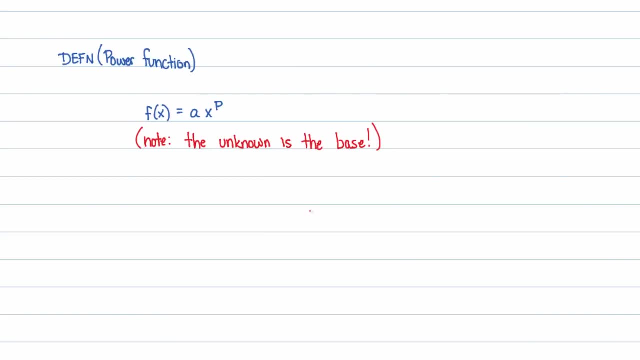 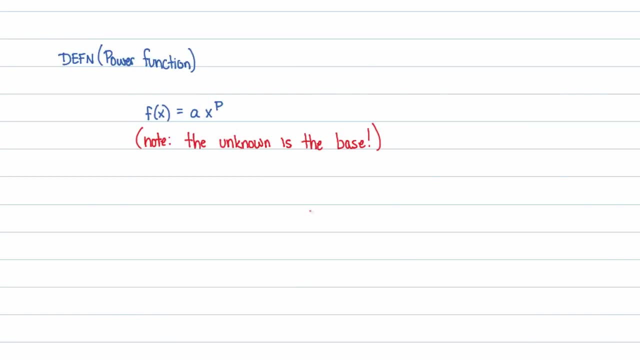 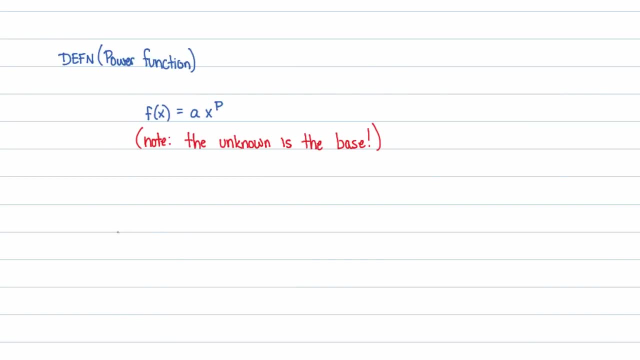 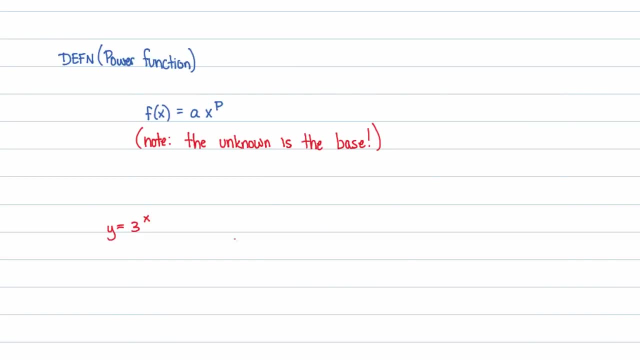 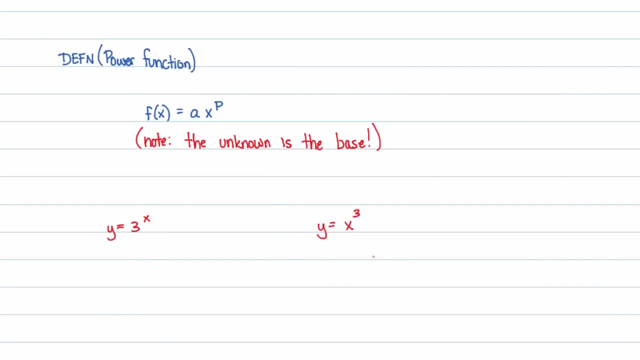 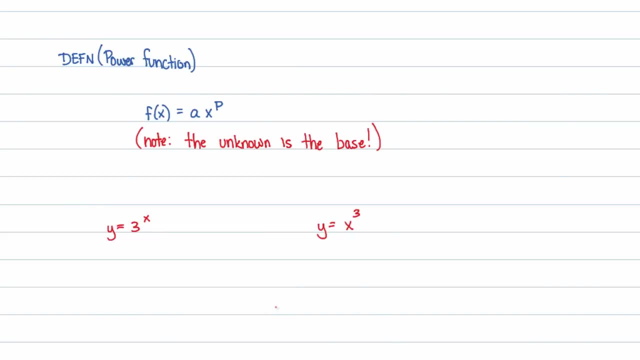 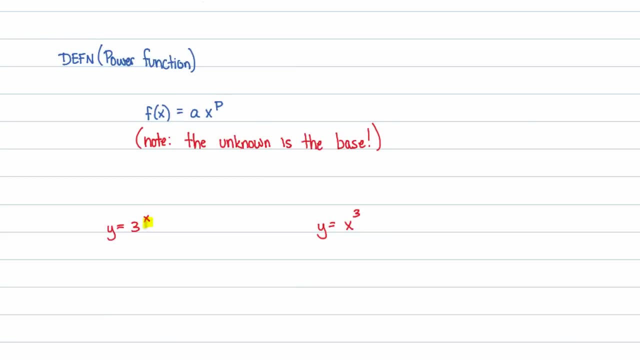 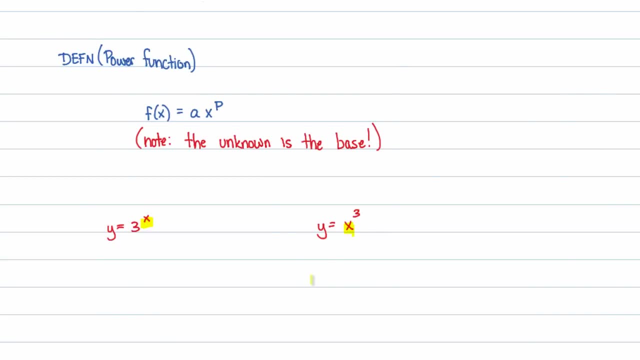 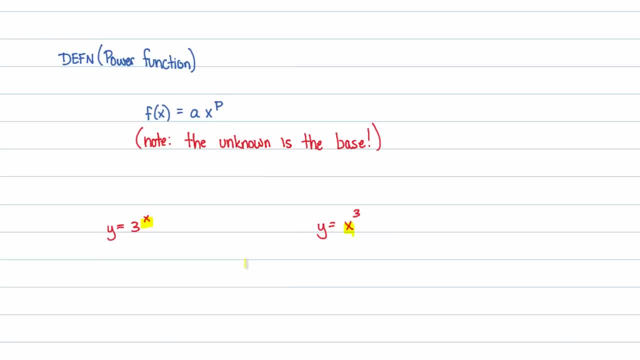 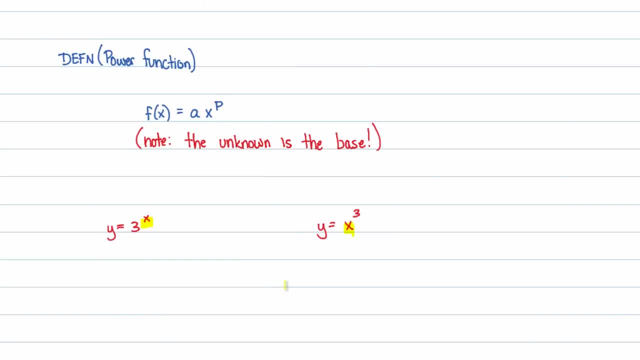 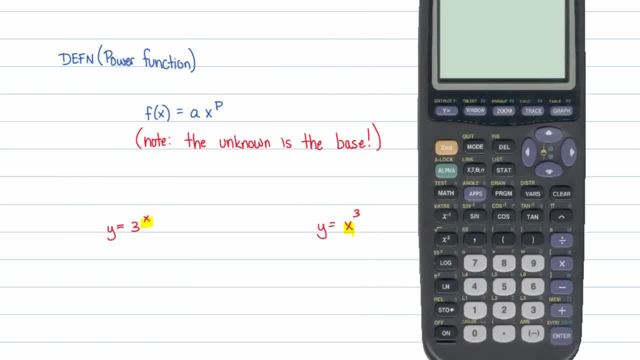 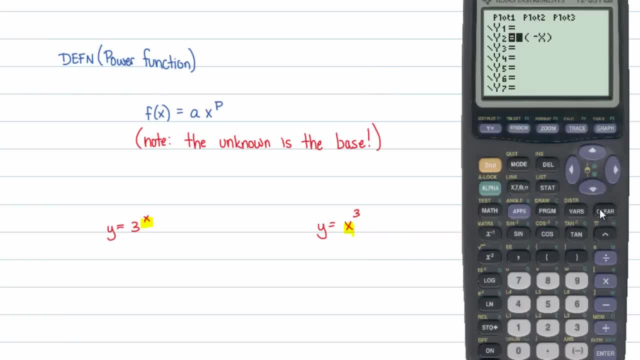 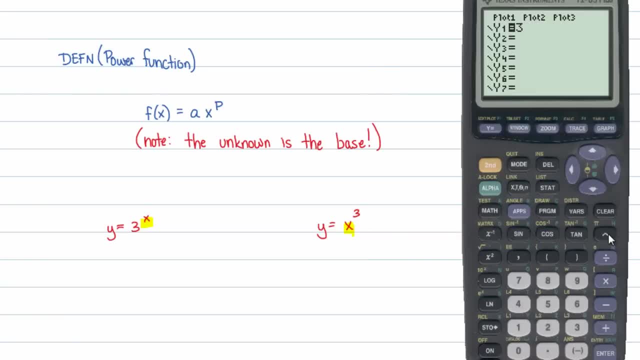 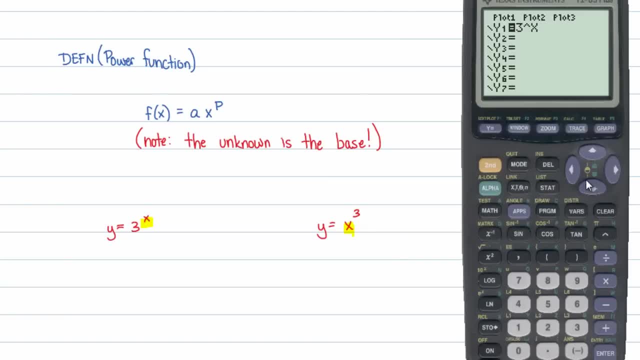 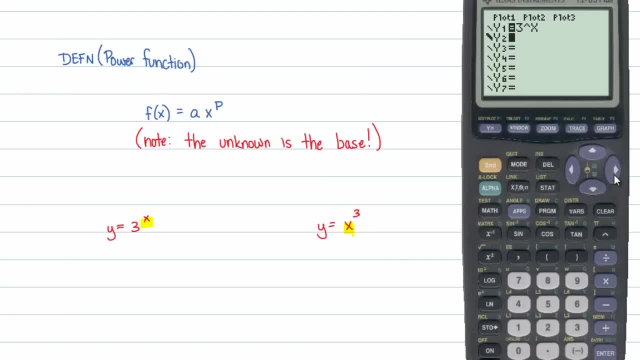 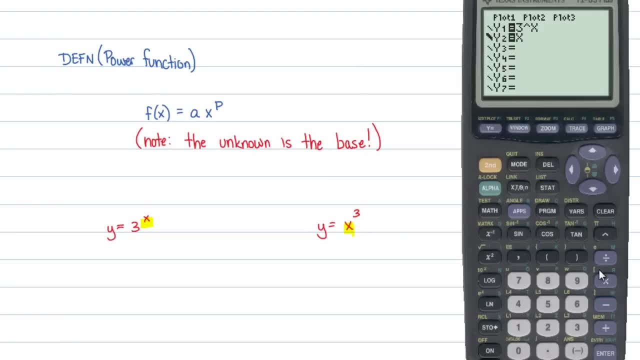 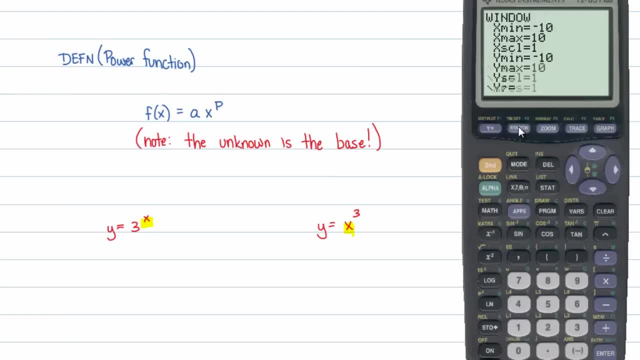 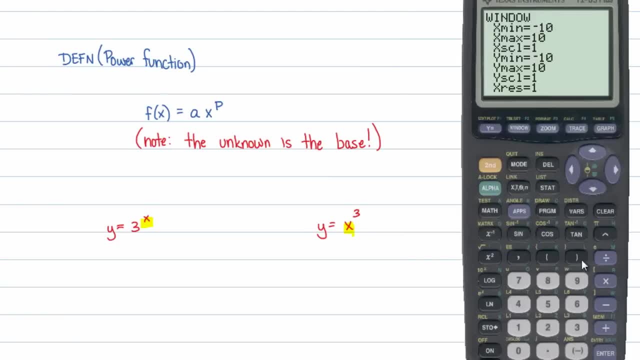 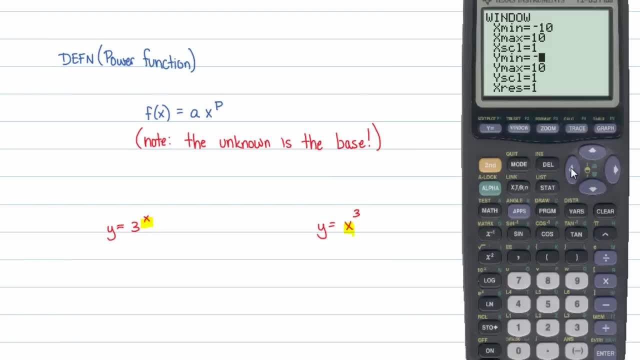 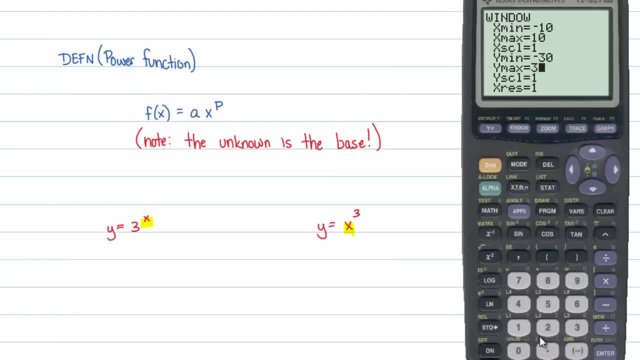 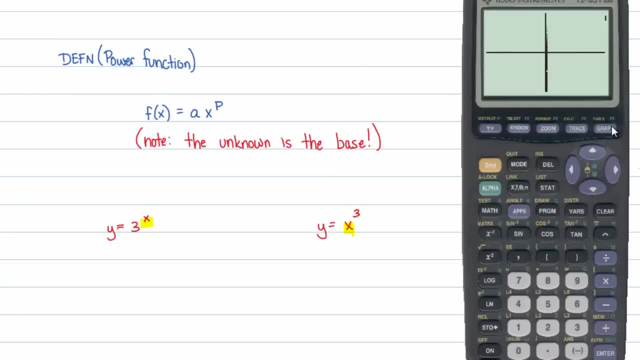 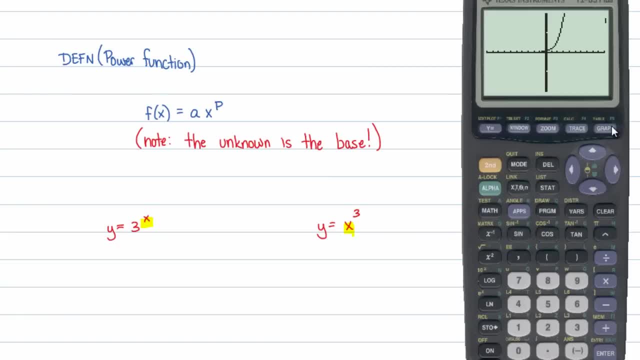 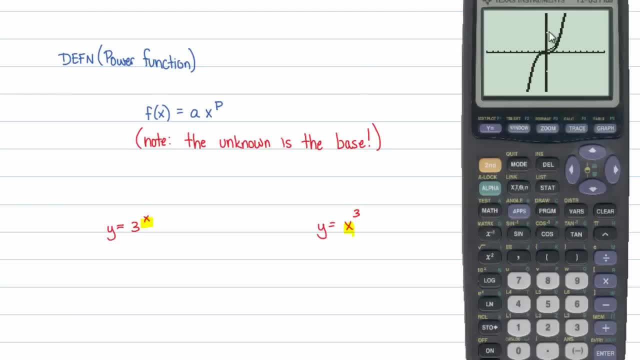 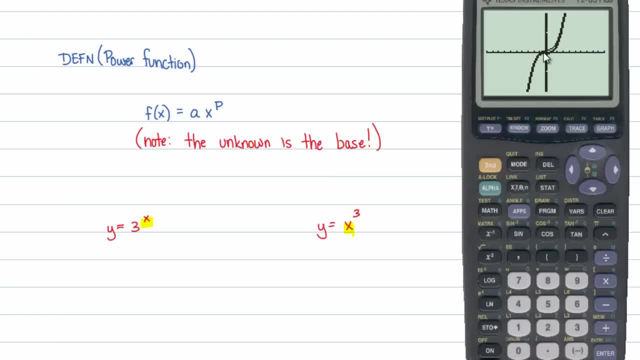 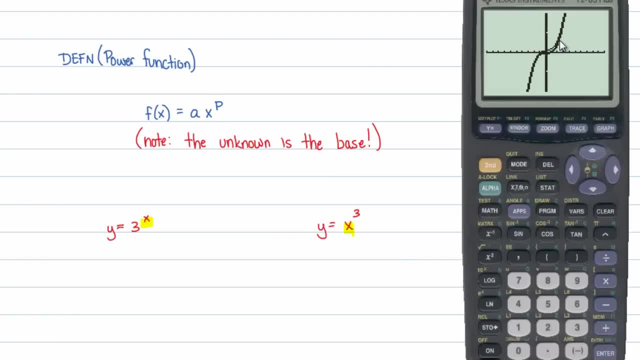 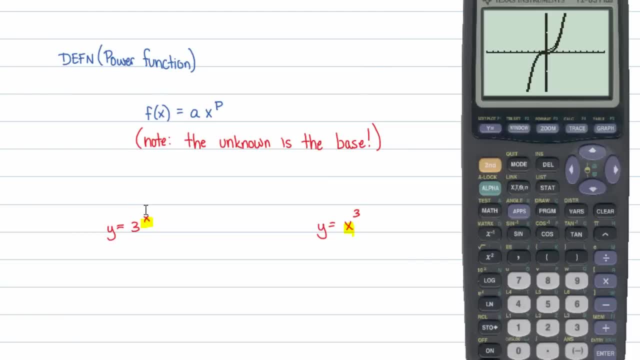 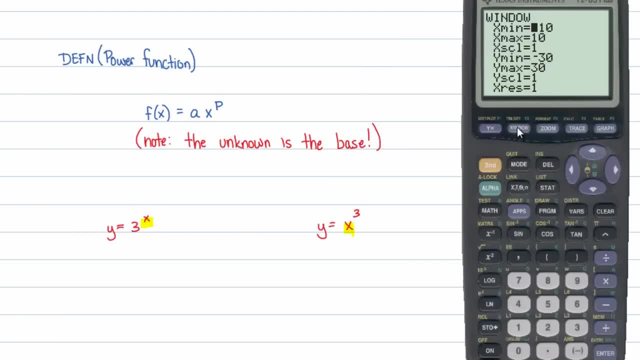 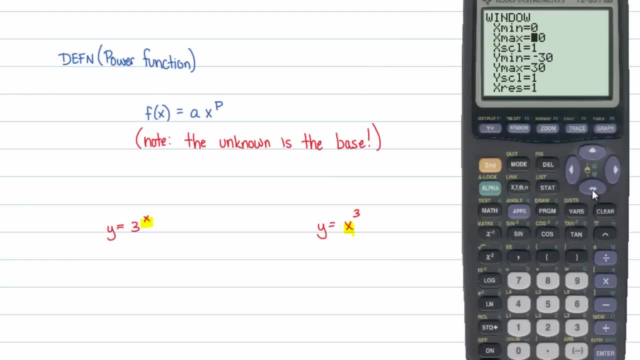 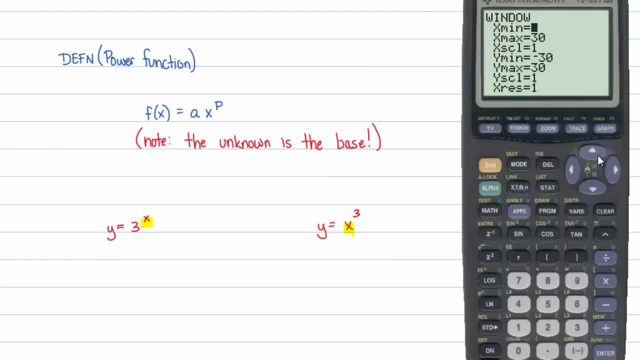 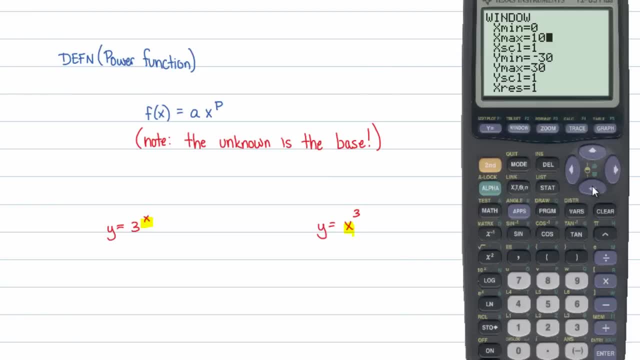 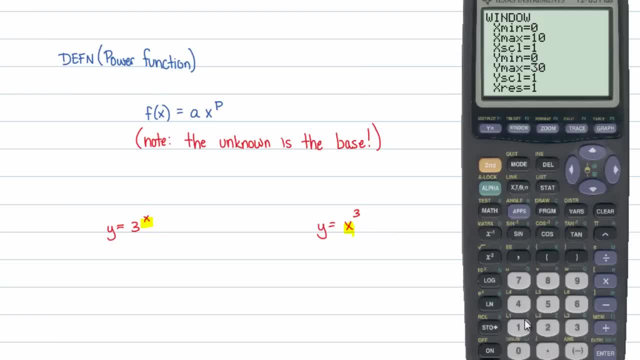 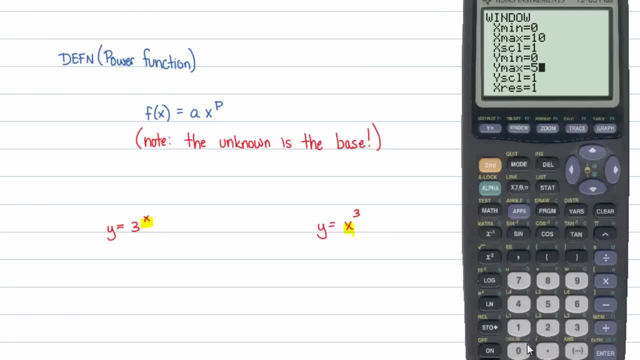 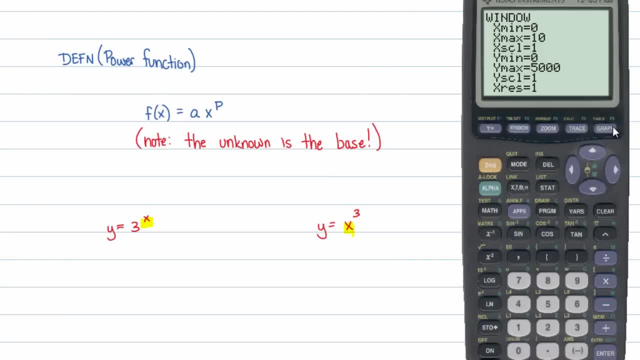 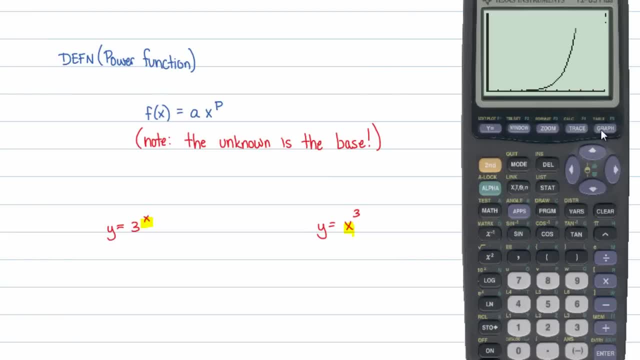 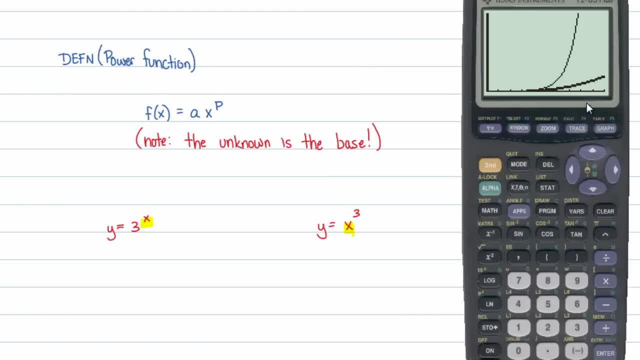 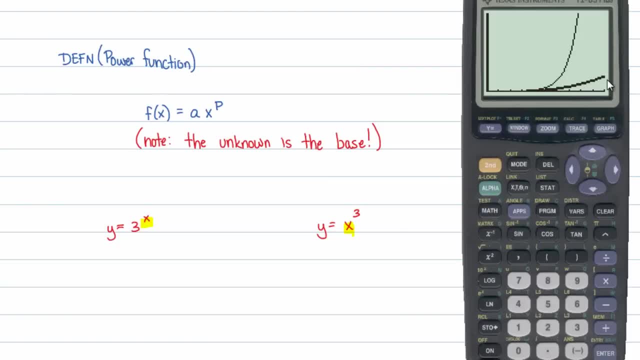 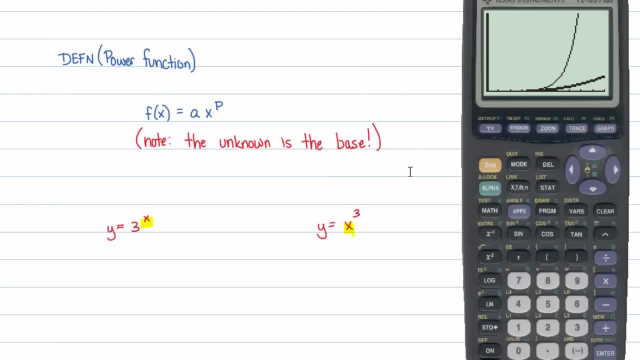 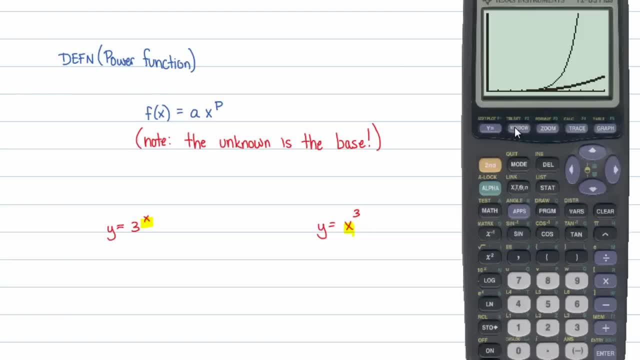 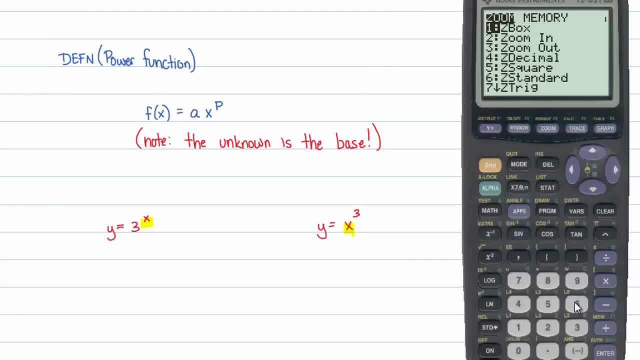 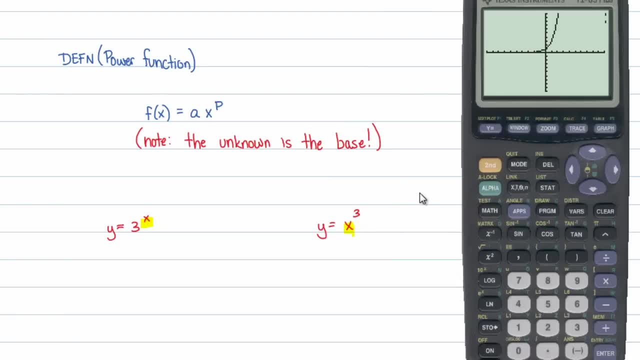 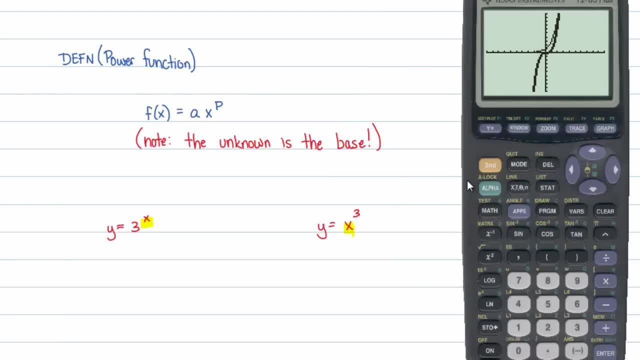 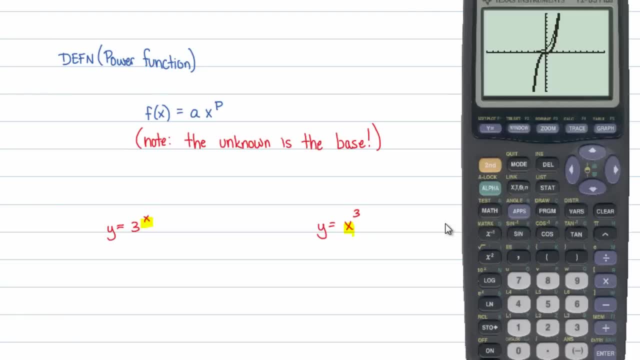 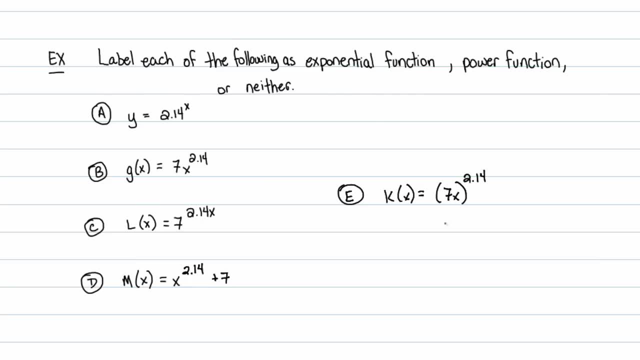 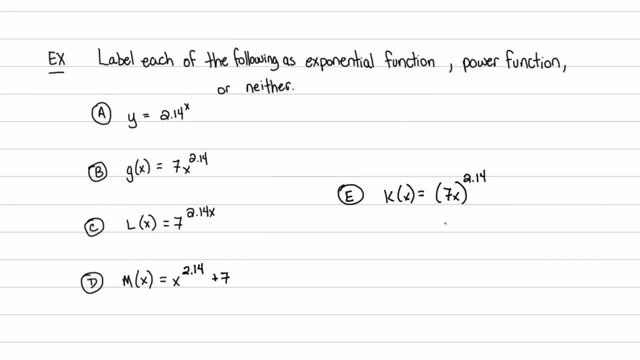 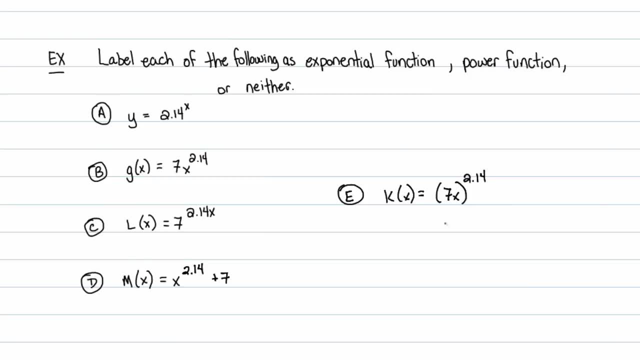 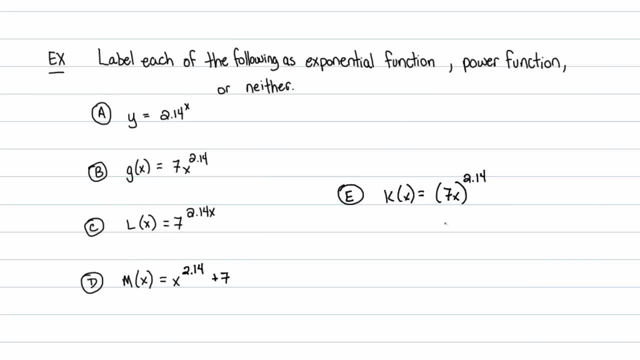 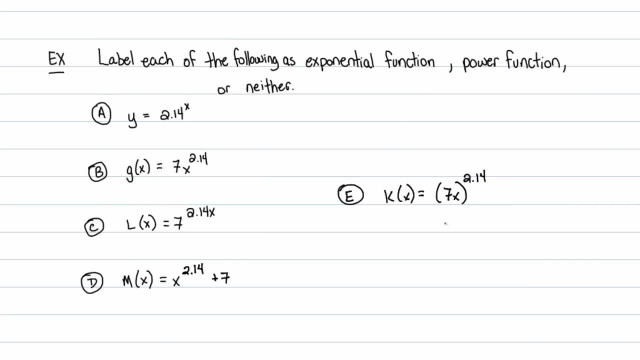 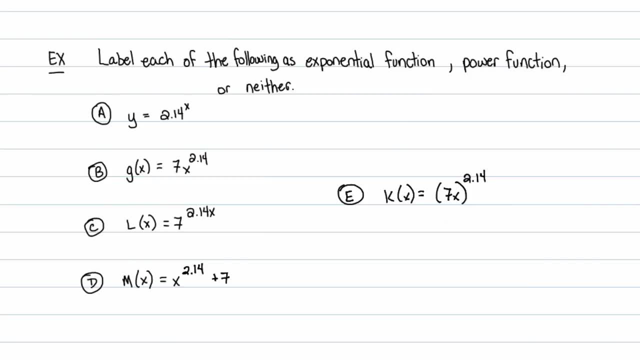 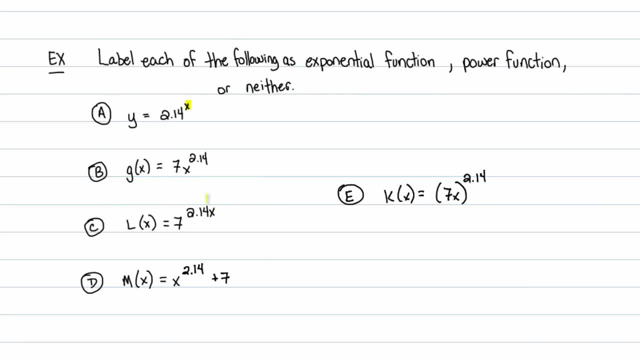 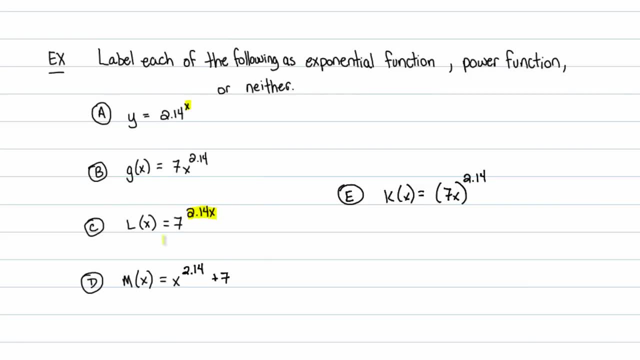 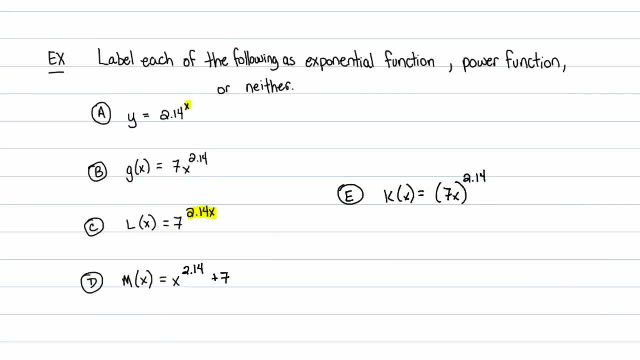 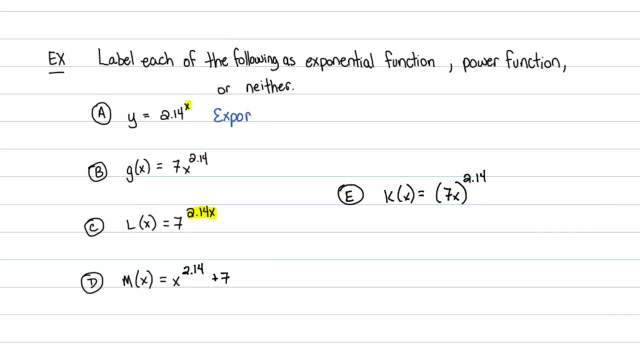 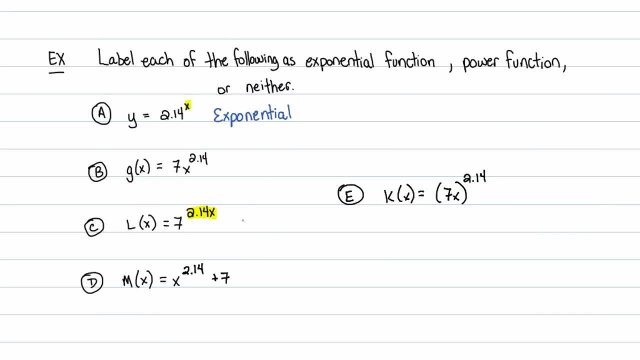 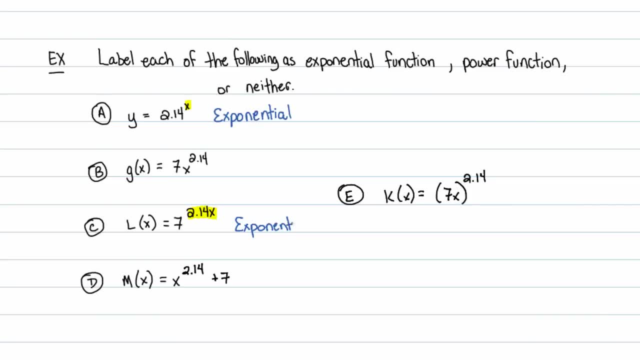 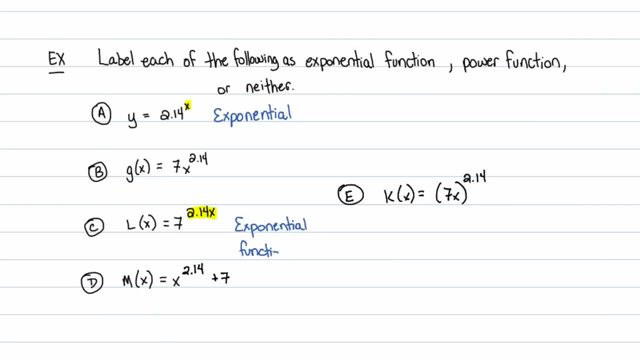 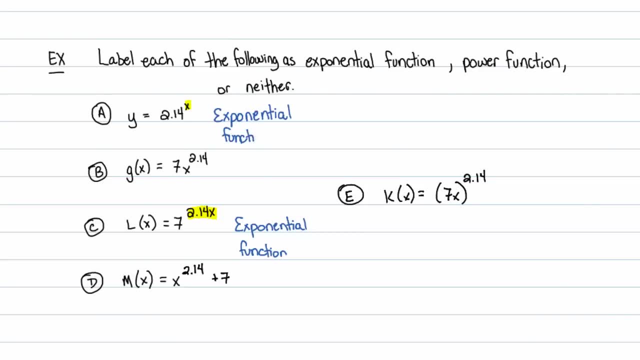 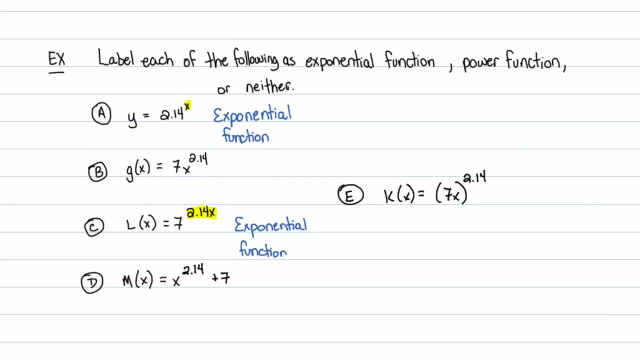 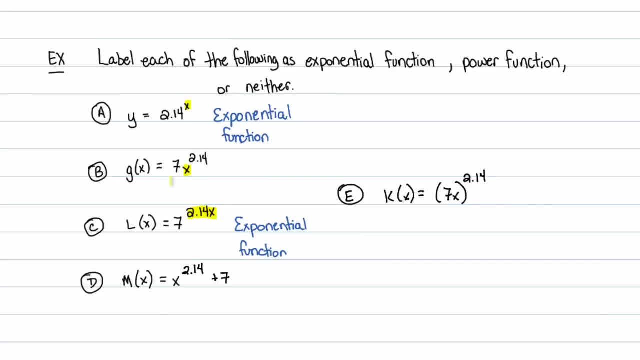 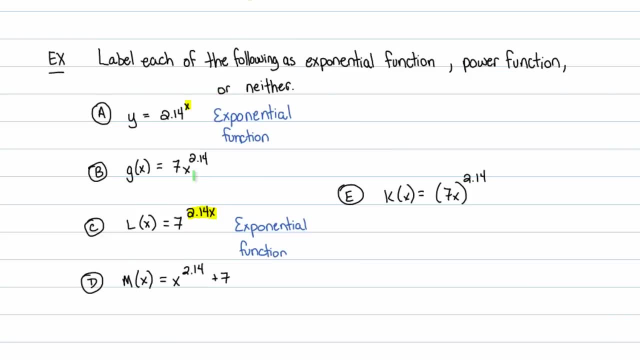 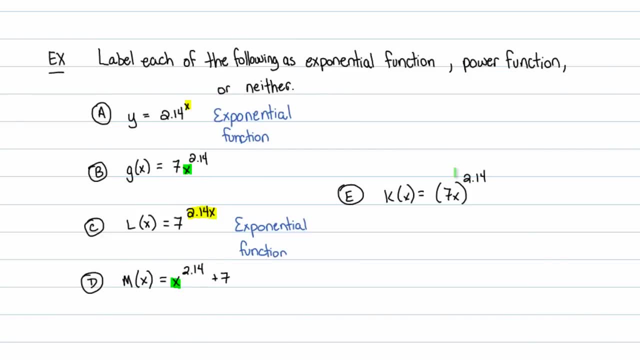 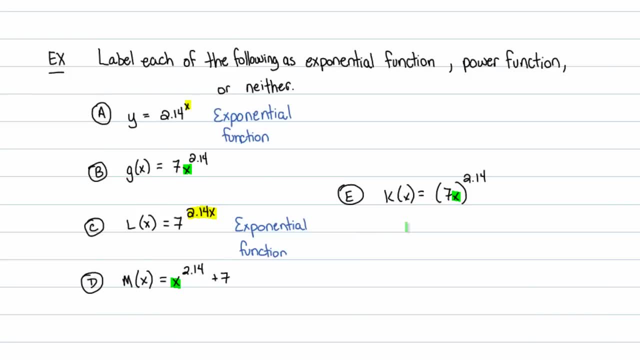 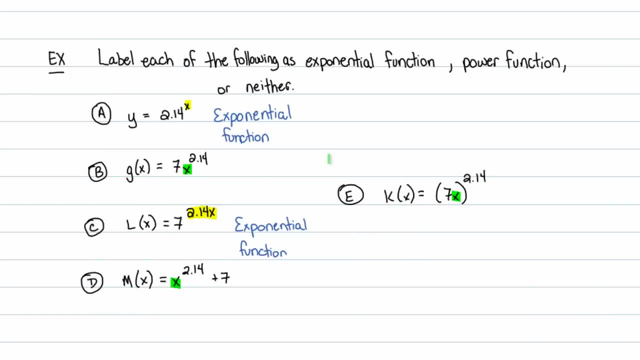 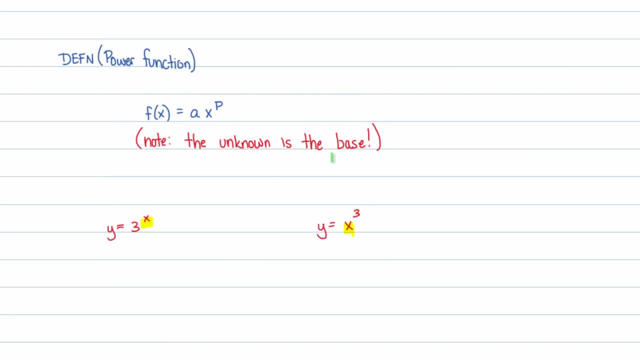 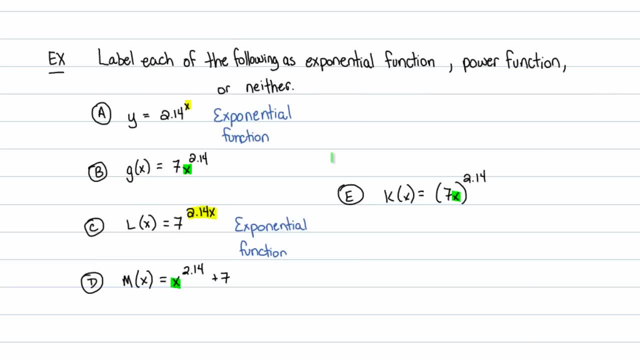 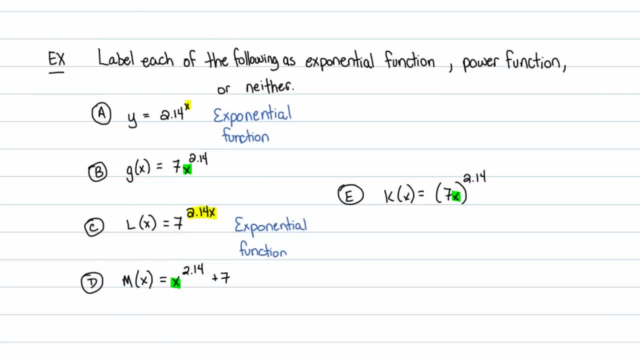 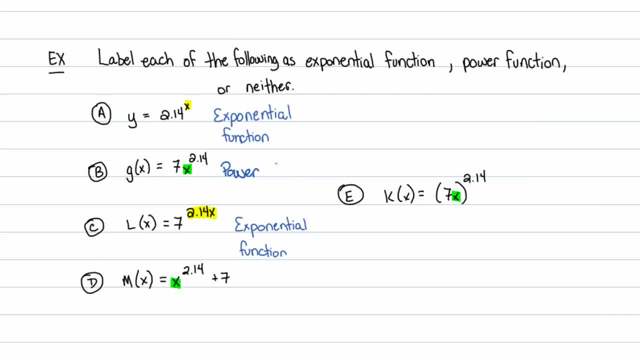 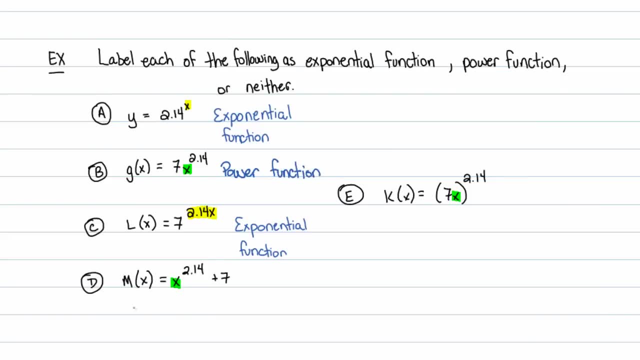 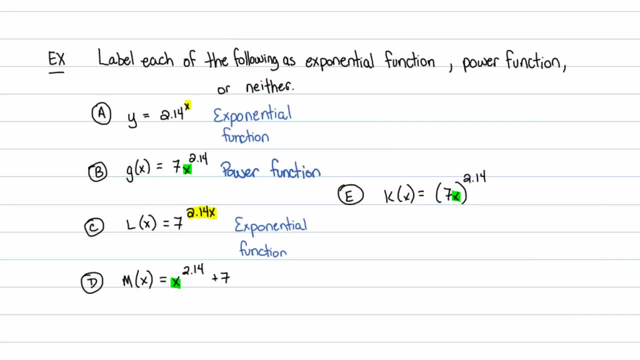 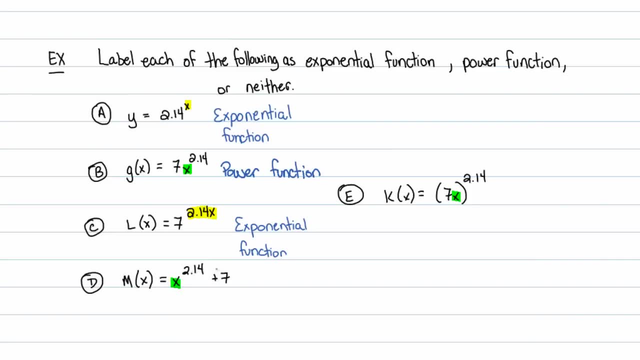 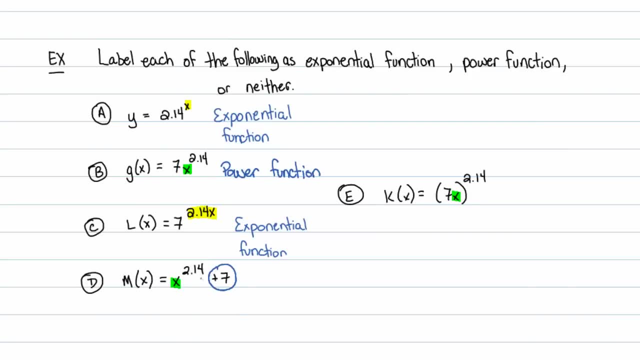 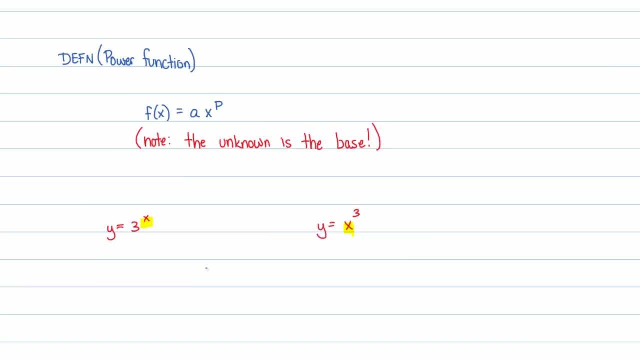 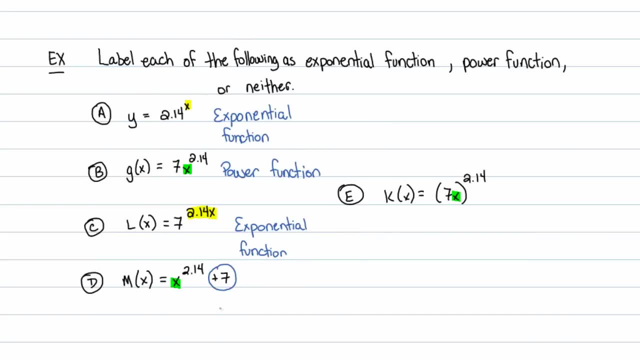 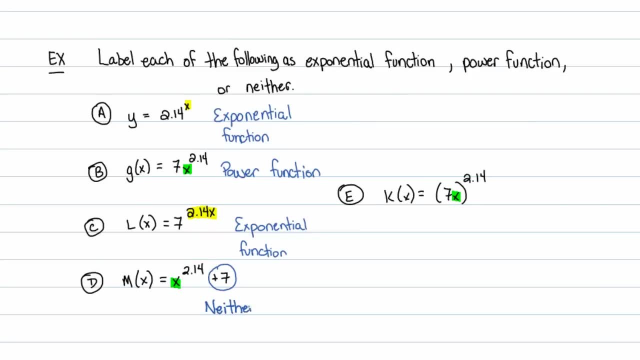 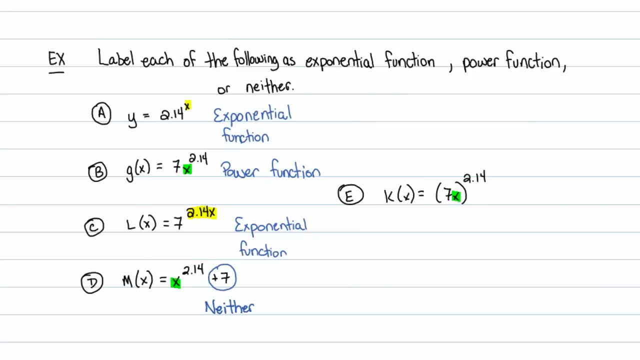 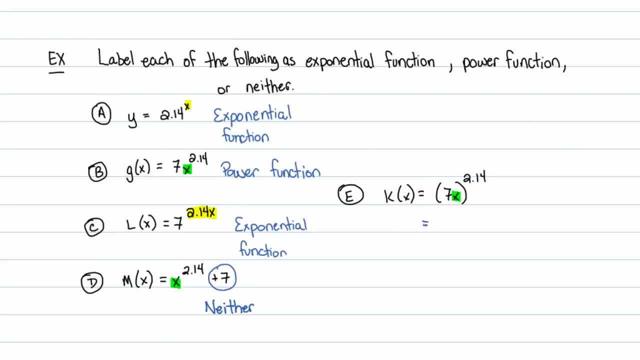 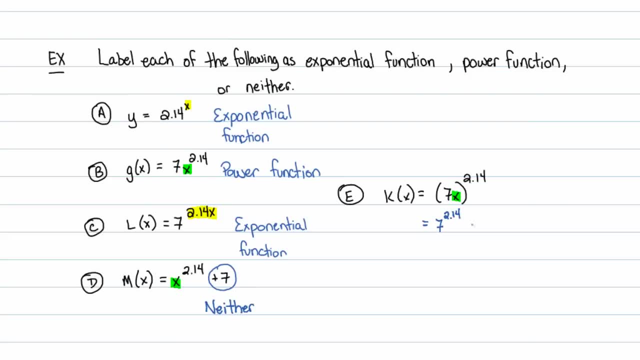 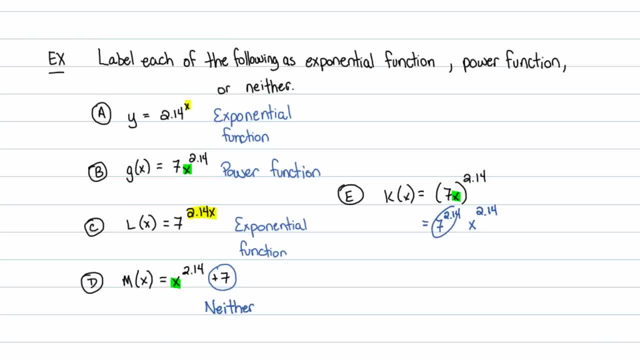 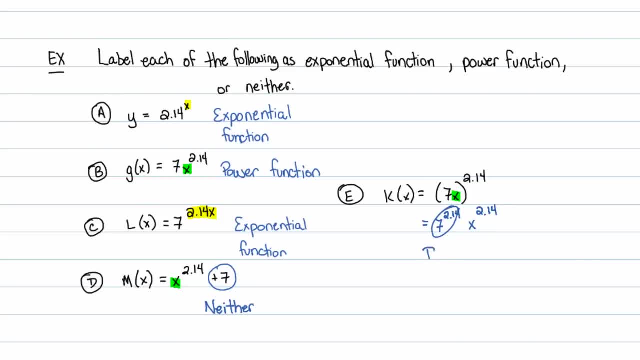 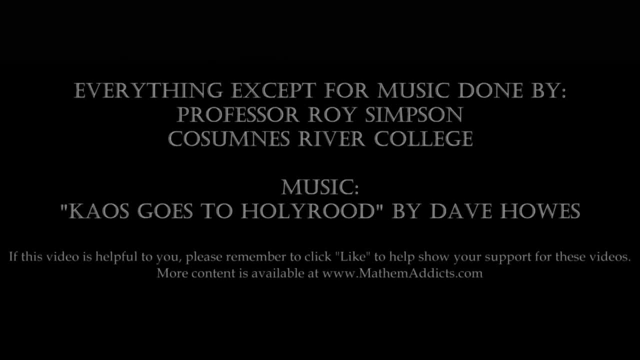 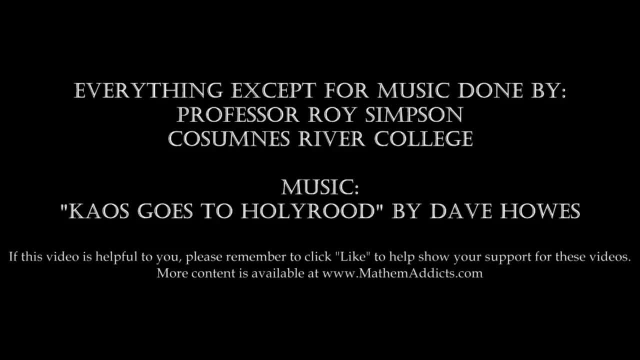